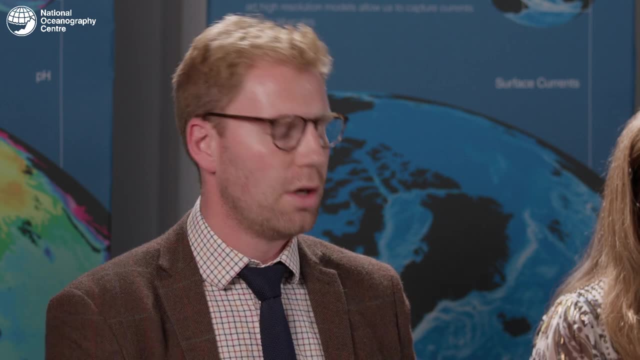 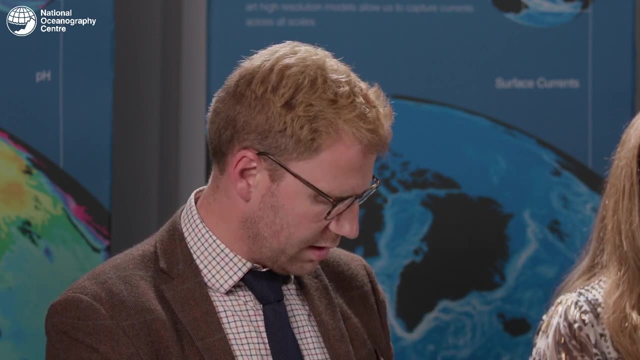 empowering position for us, Whether we like it or not. we've got the power to define the future for our generations. In so many areas we've got answers and solutions. We've got the engineering capability. we've got the wider societal support for climate change. 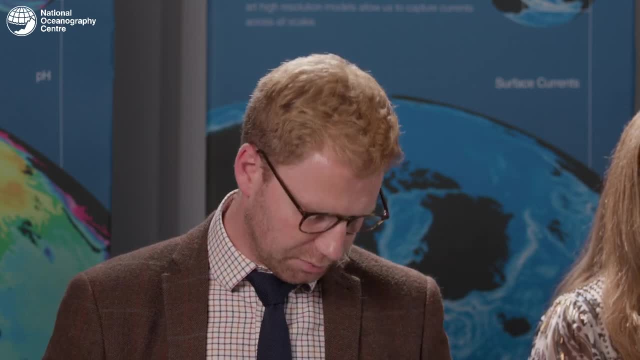 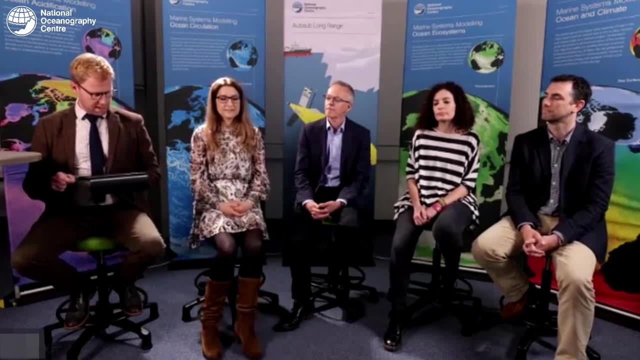 But, on the other hand, we still know so little about our planet. We're asking ourselves to build solutions. We're truly understanding the impact of those solutions And, for me, climate change solutions are not therefore just about finding a way to reduce carbon emissions or deal with carbon. 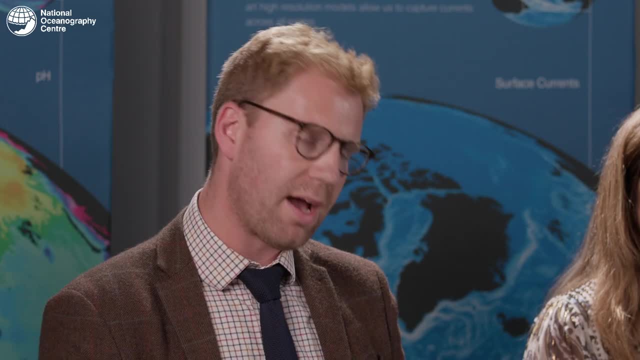 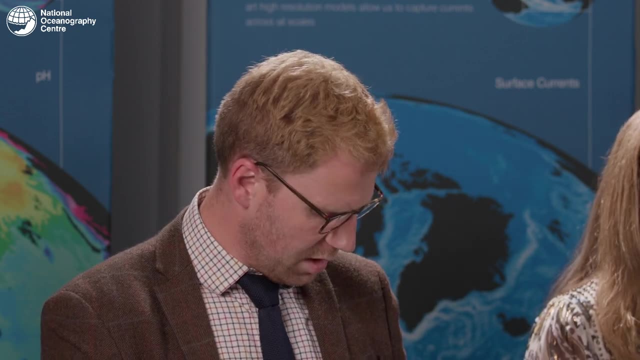 dioxide that already exists in the atmosphere. it's about how we do this in the most informed way possible, Such that the solutions we choose today don't become the problems of tomorrow. So joining me to discuss this topic are four world leading scientists from the NOC: Dr. 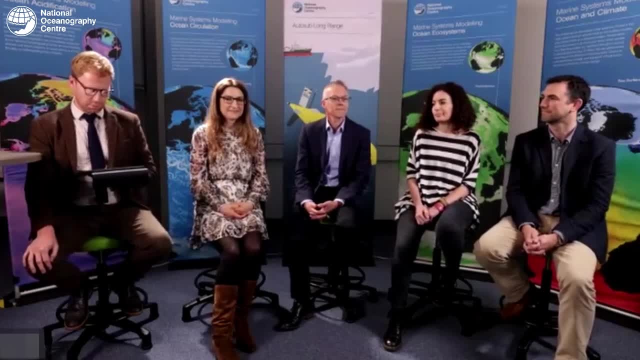 Michela DeDomenichis is a senior scientist in Knox Marine Systems, One of the leading scientists in the NOC. Dr Michela DeDomenichis is a senior scientist in NOC. Dr Michela DeDomenichis is a senior scientist in NOC. 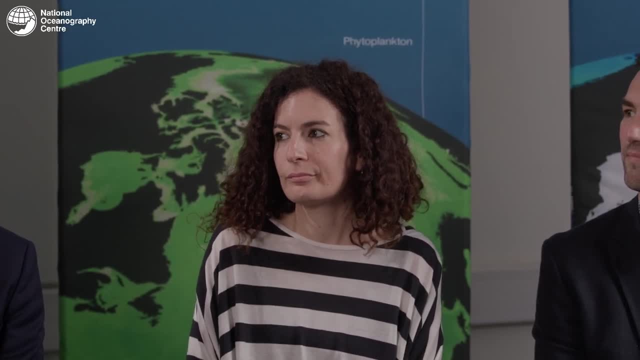 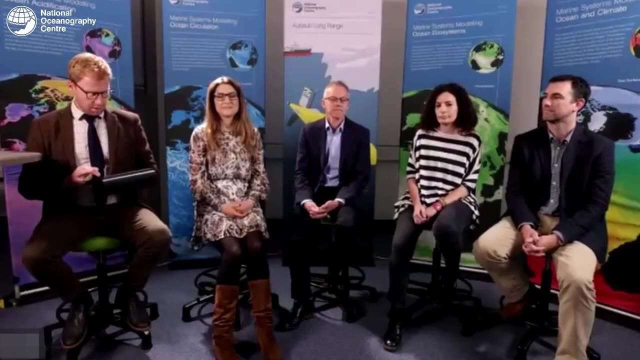 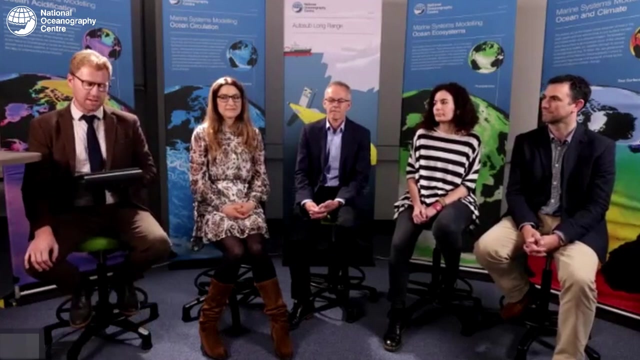 modeling group. Her particular area of expertise is understanding how the ocean interacts with any external factors, such as direct human intervention and climate change. Through her ocean modeling research, she understands the changes that might take place in the ocean in the next few decades and is particularly interested in the sort of what-if scenarios for things such as large arrays. 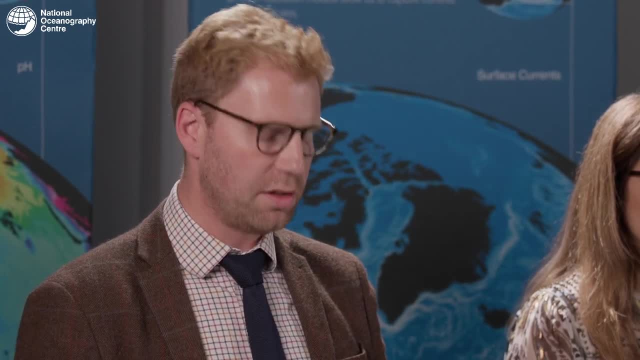 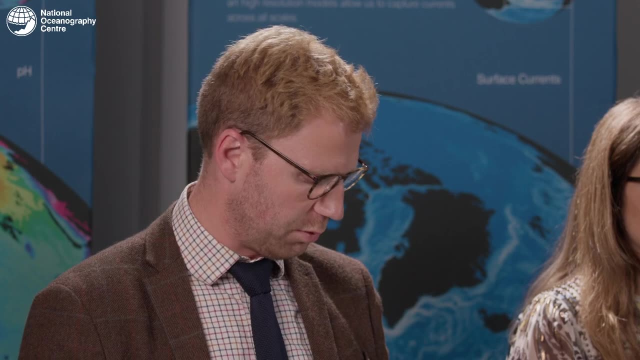 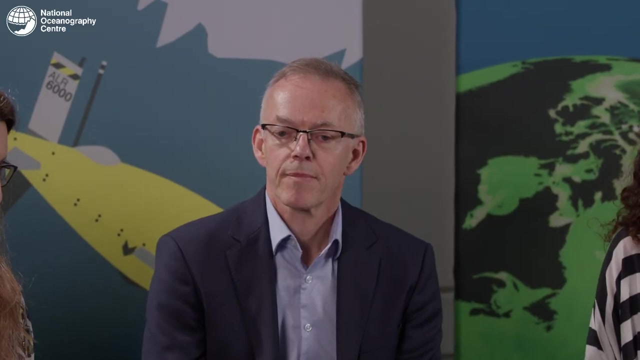 of offshore renewable energy infrastructure- wind turbines, underwater tidal turbines- and the response of coastal areas to extreme storms, sea level rise and different coastal protection measures. Professor Doug Connolly is Associate Director for Research at the NOC. He's a marine biogeochemist with a long history looking at a range of science questions that stretch right 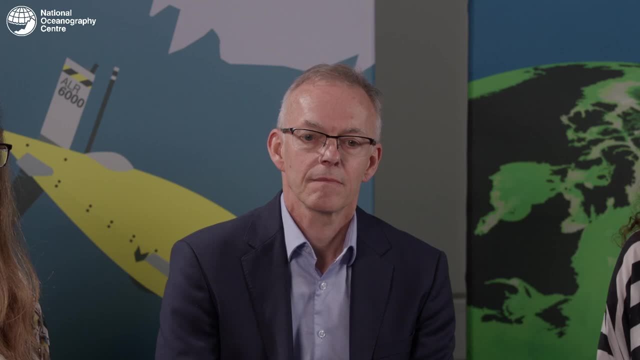 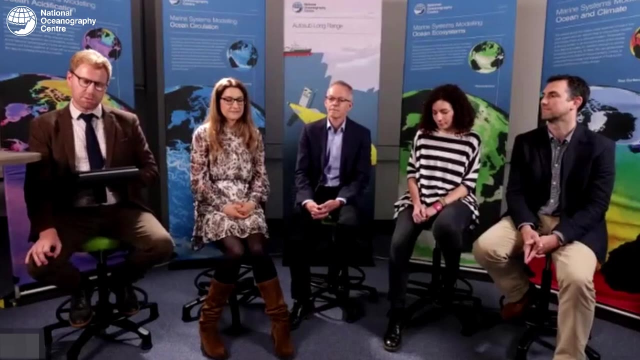 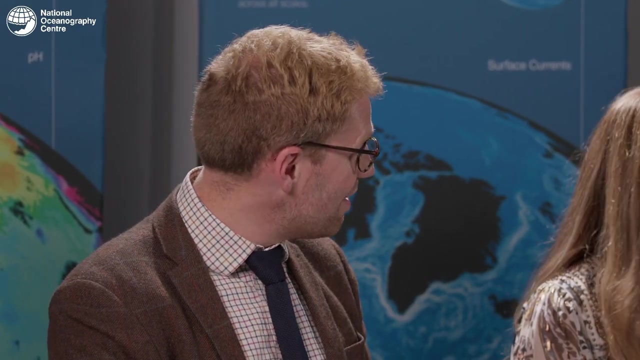 through, from underwater volcanoes through to climate change mitigation using carbon capture and storage. Doug has worked in various roles all over the world during his career and he's regarded as the top scientist for discovering and understanding hydrothermal vents. He's found hydrothermal vents in every ocean in the world. 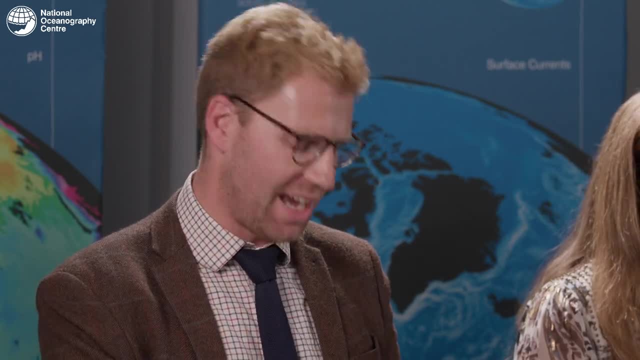 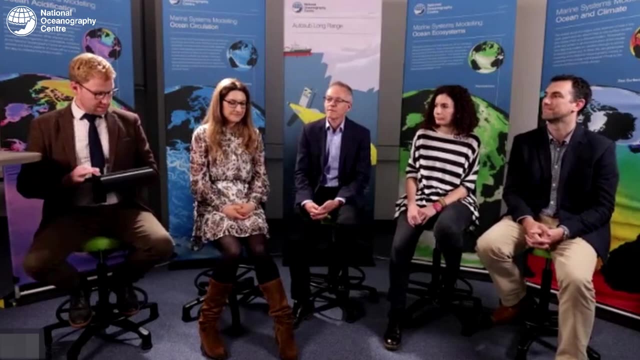 on the planet, and that includes the deepest ever found in the Caribbean Sea. He's also the UK stakeholder representative on ICOS, which is the International Carbon Observing System. Dr Claire Evans is a senior biogeochemist whose area of expertise is in understanding and 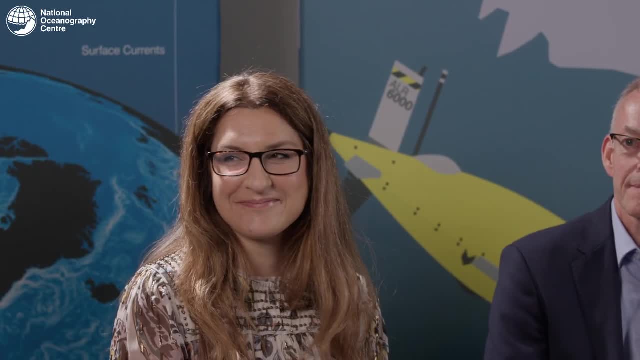 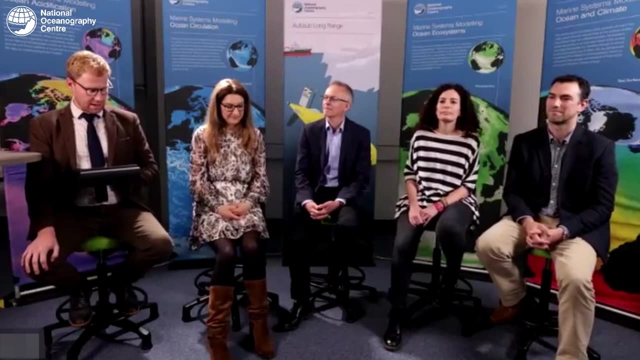 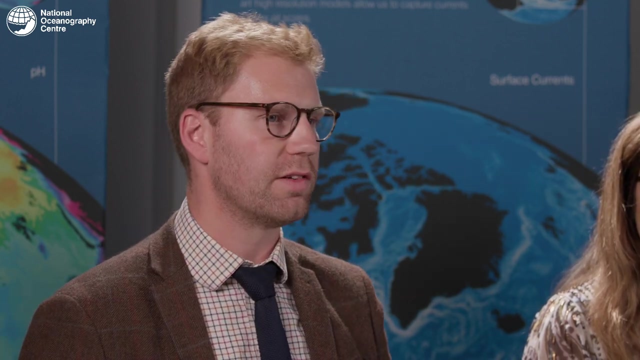 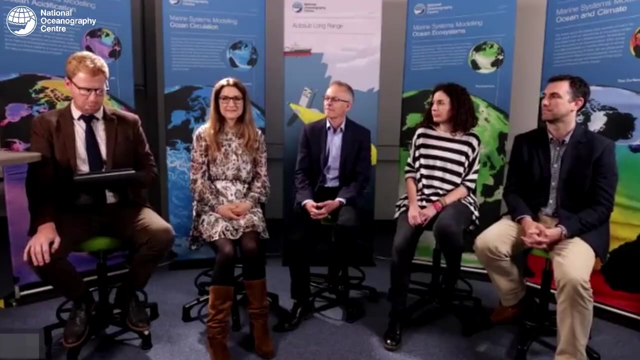 integrating biogeochemical cycles into the larger socio-economic context. Carbon sequestration is her principal focus and research, and that encompasses themes such as blue carbon and integrated coastal zone management. For her research, Claire employs quite a pan-disciplinary approach by working closely with a range of different scientists and engineers. as 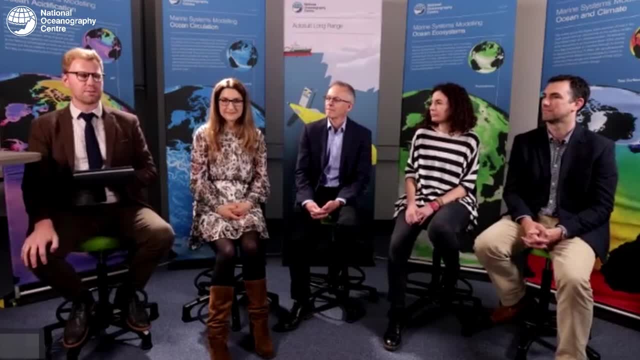 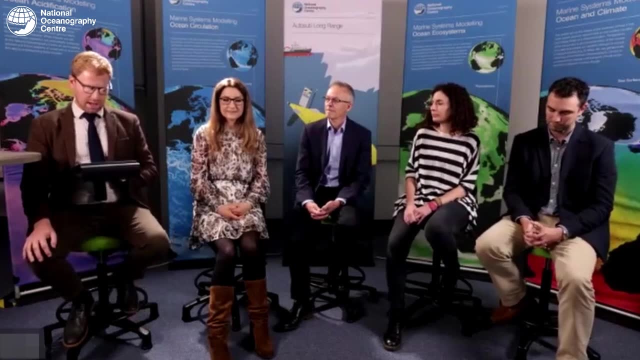 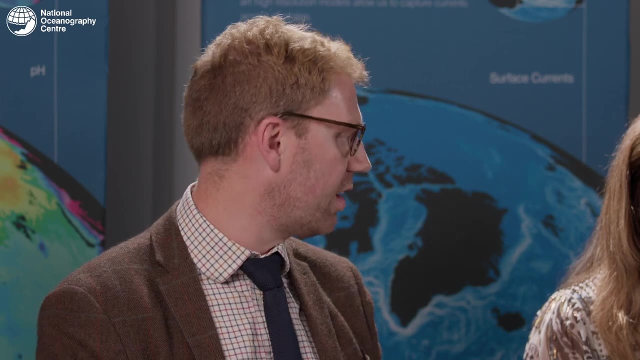 well, with different expertise, to build up a really rounded scientific picture of the environment that she's studying. This is particularly important for a number of stakeholders that Claire works with, as her scientific knowledge and understanding is really key to making economic and societal based decisions. And finally, Chris Pearce. Dr Chris Pearce is a marine. 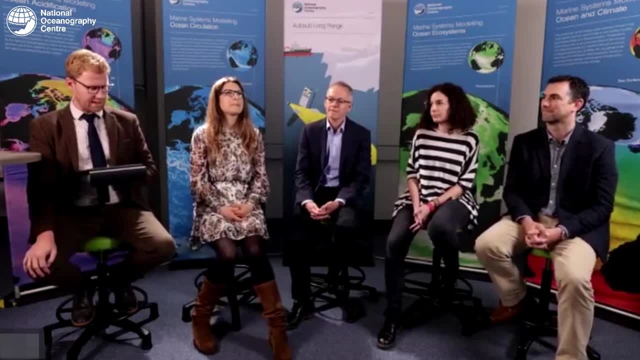 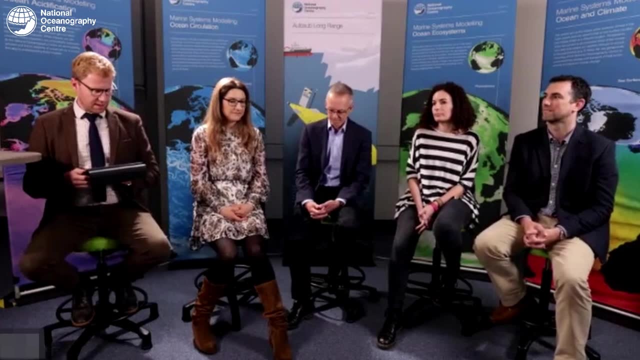 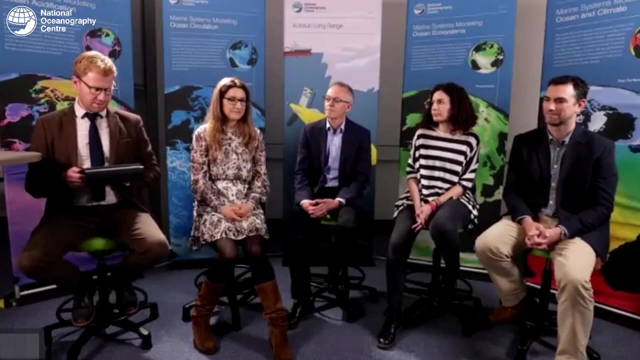 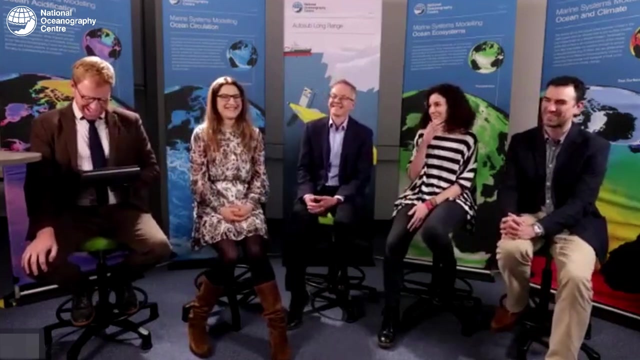 geoscientist whose research aims to better understand the processes that cause and help mitigate global climate change. His expertise is in geochemical techniques has enabled him to investigate how global systems and biogeochemical processes are affected by environmental perturbations, as well as how long the planet took to recover from past climatic events. 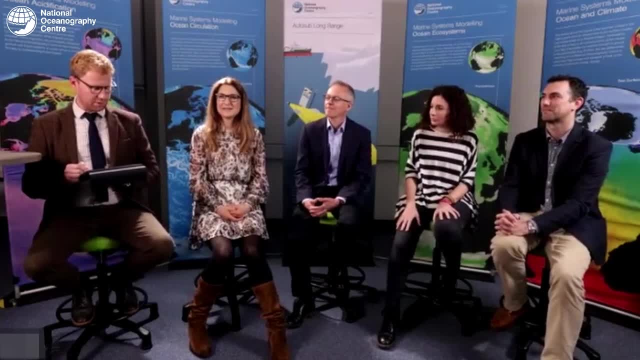 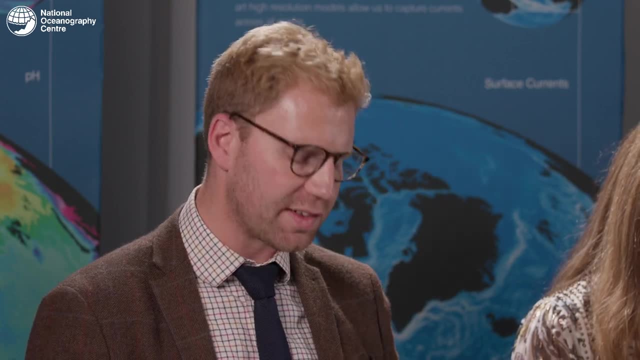 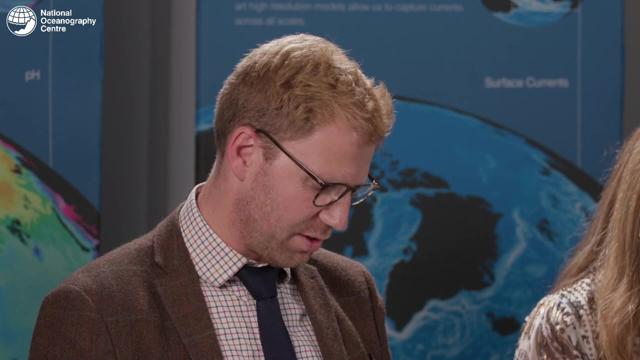 Chris is currently using that knowledge to investigate potential mechanisms for combating modern climate change, such as enhanced rock weathering and carbon capture and storage, with a particular focus on the application of state-of-the-art technologies to monitor and assess both the efficiency and environmental impacts of those approaches. 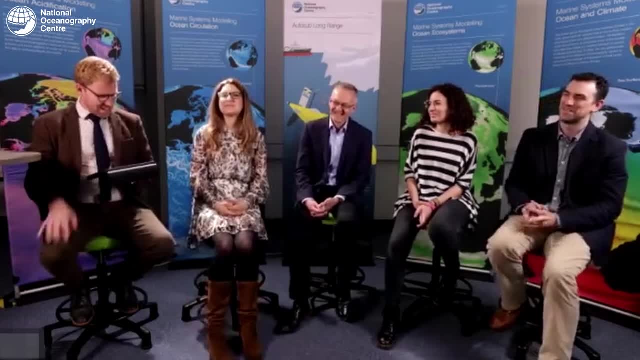 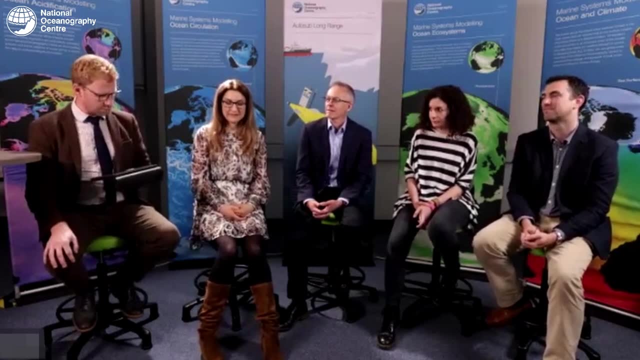 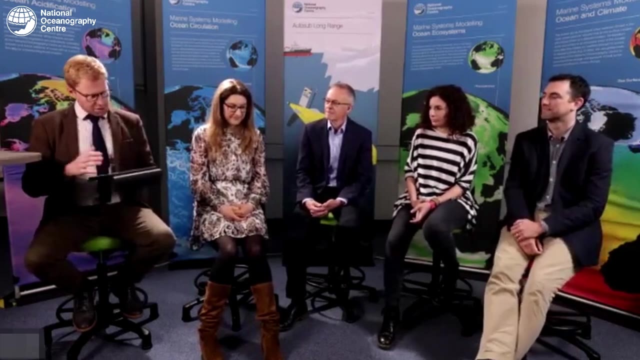 말씀 landscape. i guess, in terms of climate change solutions and and doug, i'm going to sort of direct this one to you, if i may, with that sort of overarching view. so i think you know the majority of people are aware that we've got a range of solutions for reducing carbon. 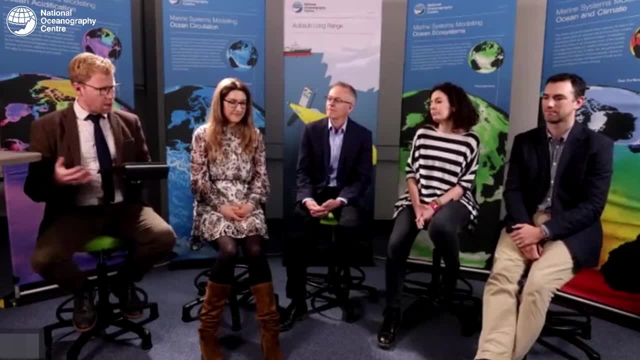 emissions electric cars renewable energy sources etc so you know a plethora of solutions if you like could you give us a bit of an idea of how you approach climate change and how we as a beforehand gel and 199 00 � delete or generate enough steam is genuinely necessary to emerge carbon emissions from the dark and mount wow that we're coming to. So it's a question i will give some answers to when the climate changes and drug JCстве is a big time factor for best тон but covering this 노래 of climate change solutions right in the bottom of the chamber in the name of habitat quite clearly doesn't happen in this舞 so Anatomi 180 00 RCPIt under current circumstances growth 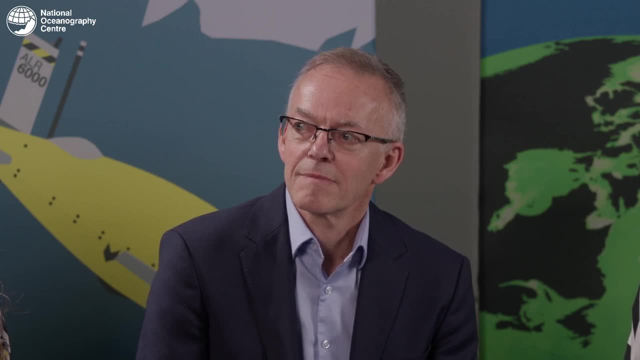 bit of an idea of the scale of some of the less well-known solutions perhaps, and maybe how well they develop they are in relation to things that we know about. i was sort of splits into two with claire actually, because clay can probably talk to them more sort of the biological basis. uh, i. 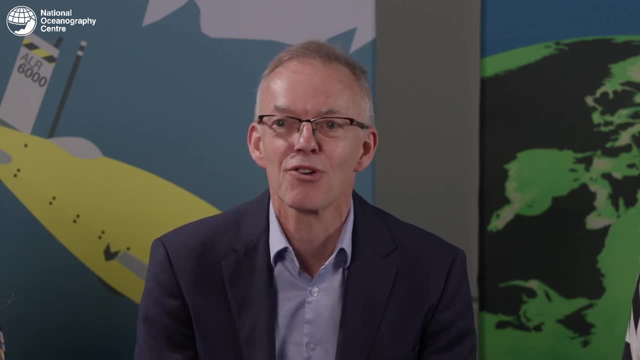 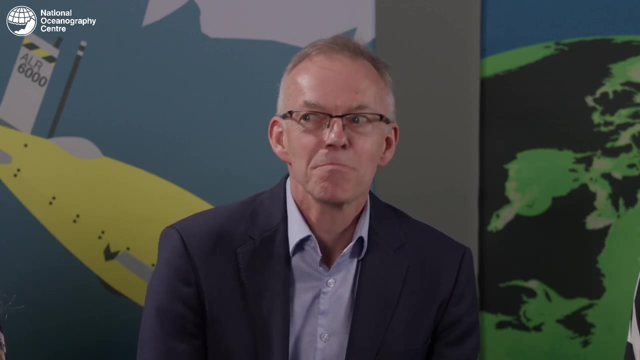 spend most of my time doing the sort of interventionist approach, sort of carbon capture storage, direct air capture. um yeah, we're producing about two tons of co2 per person per year on this planet, about 36 gigatons per year, and we've got, obviously, climate change as a response. 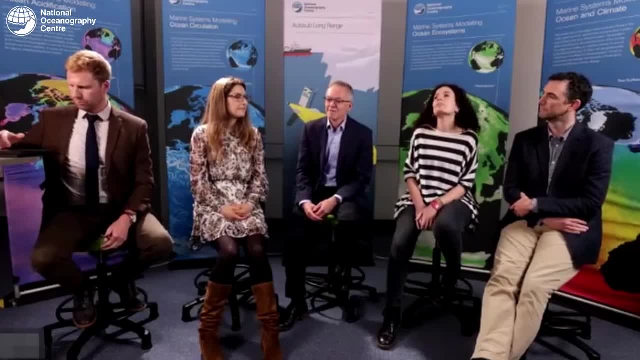 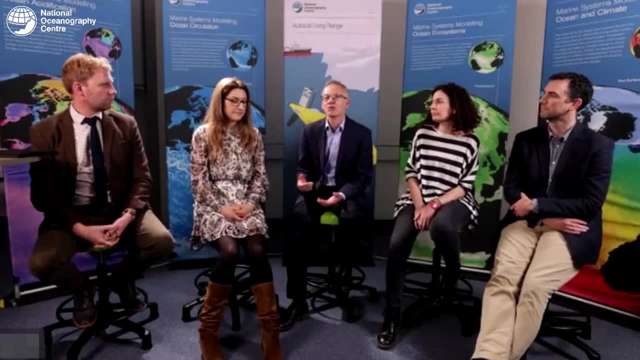 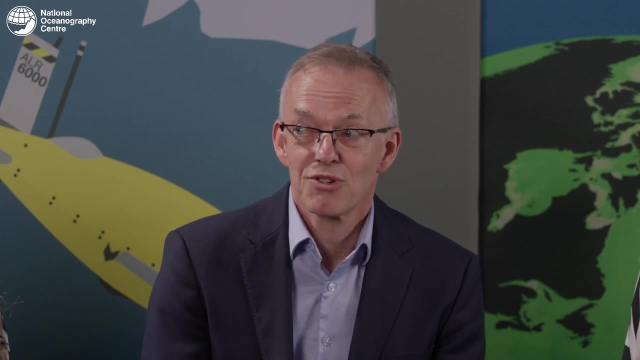 to that release. the idea of using- basically capturing that co2 and storing it in some way or reusing it, is actually a driver behind one of the sort of more industrial interventionist approaches. to give you some idea of the scale we we've estimated in terms of storing co2, just for: 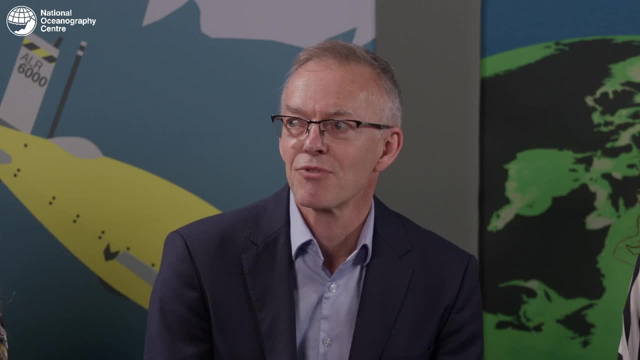 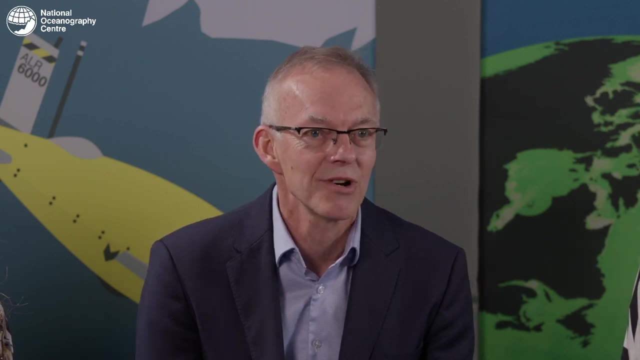 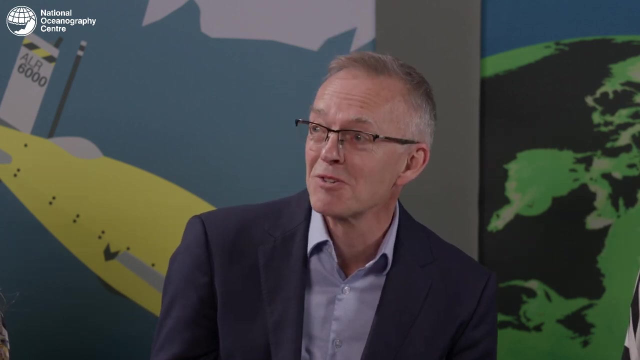 the uk we can store 500 years of co2 emissions from the uk current emissions just in the north sea basin alone, using a combination of depleted oil and gas reservoirs or or some sea aquifers. so in terms of the the this the space to store the co2- we've got it. it's um a relatively developed area of research. 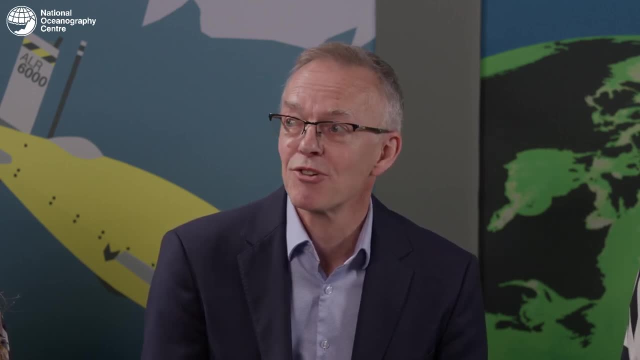 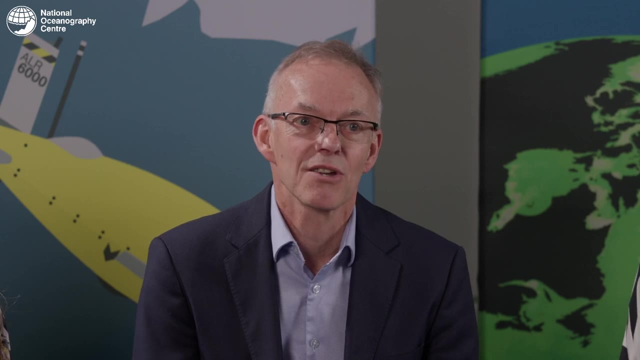 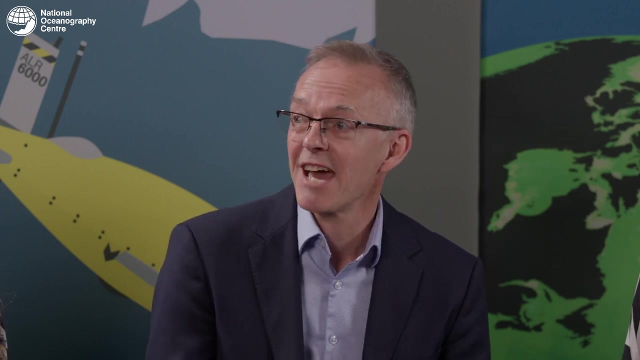 uh. the slightener um ccs program has been capturing co2 uh in the north sea of norway since about 1997 and they've captured and stored a million tons of co2 every year since then. so it is a demonstrated and proven technology. it's just not been used at the scale we're probably. 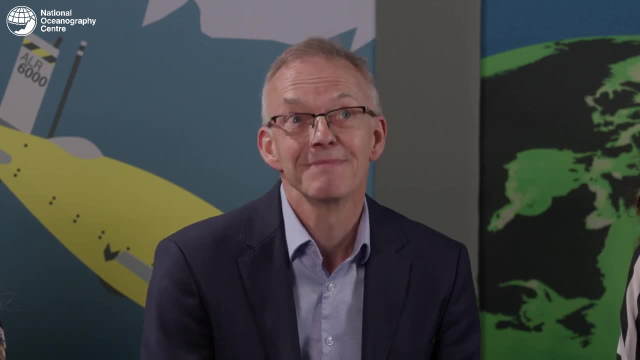 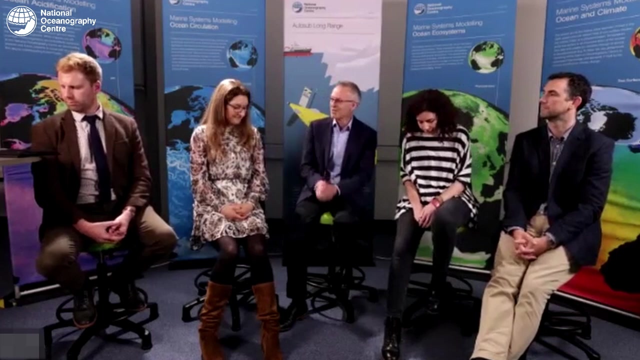 going to need into the future, and so it's sort of one of the low hanging fruits really. um, it is purely a mitigation and a stop gap. it is not the solution to producing co2. it just offsets what we're producing at the moment, where some of claire's work i can hand on to you onto. 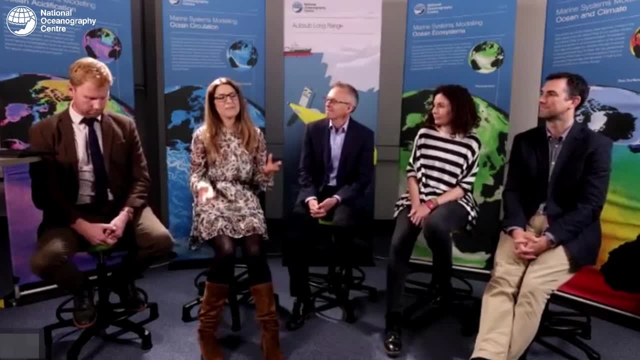 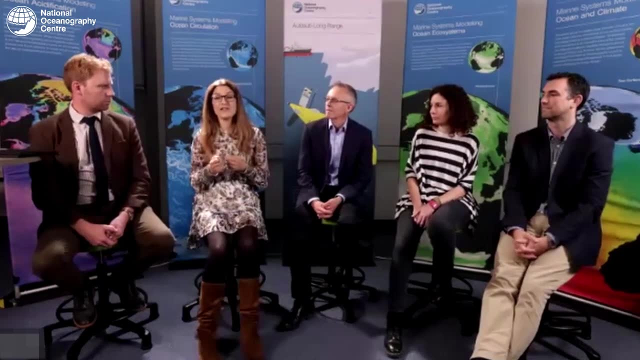 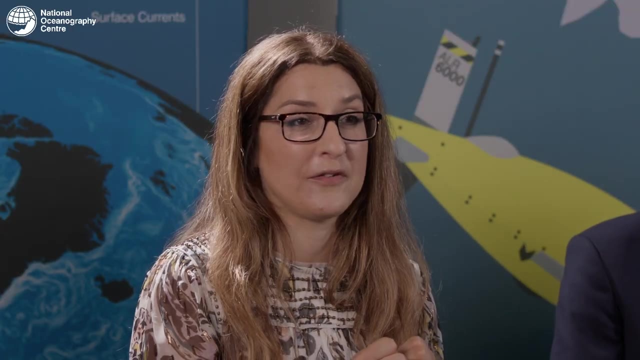 the bio approaches? sure so um, the sort of work that i'm interested in in terms of mitigating, uh, the climate crisis, as it were. um basically utilizes natural solutions. so nature has a fantastic way to actually capture carbon dioxide from the atmosphere, and that's via photosynthesis. so 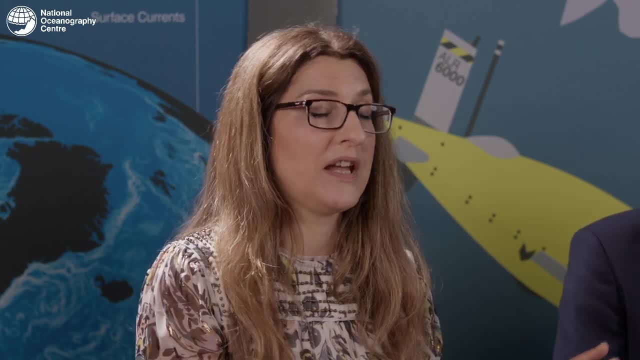 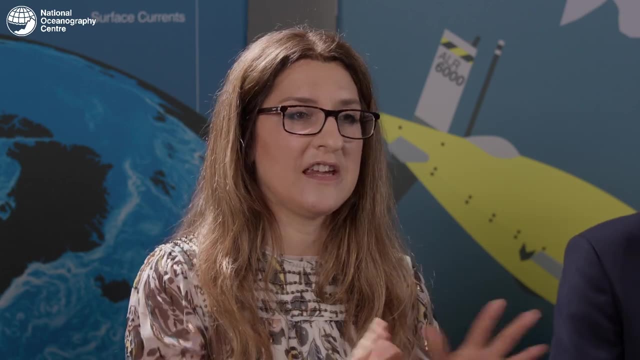 what we're looking to do is utilize that process and try and control it in the marine environment. and you might think, well, how can we do this? so there's a number of ways, and you spoke about feasibility, so some of them are quite easy and straightforward, and then some are more complex and 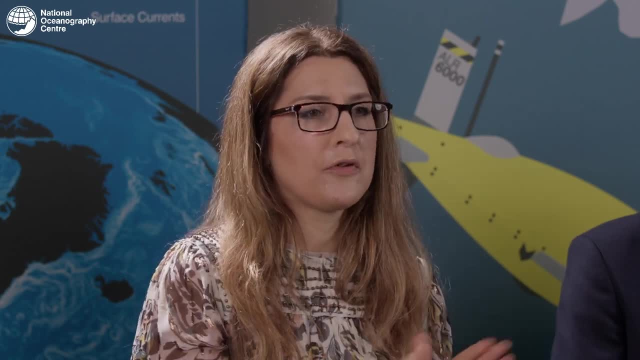 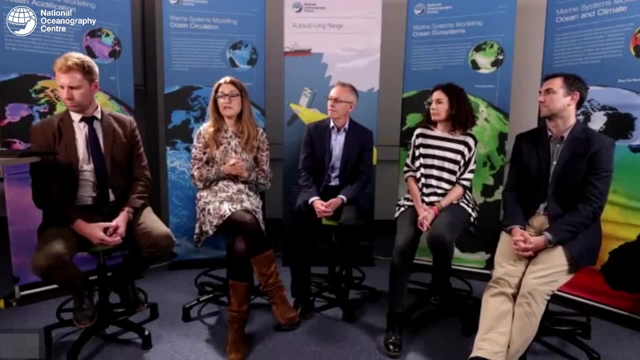 have various performance indicators, and some are quite complex and have various priorities, which are what we're looking to do in the future. I'll give you a moment to think problems associated with them, but talking about the one first that people have probably heard about, and that's this term: blue carbon. so blue carbon means different things to different people. 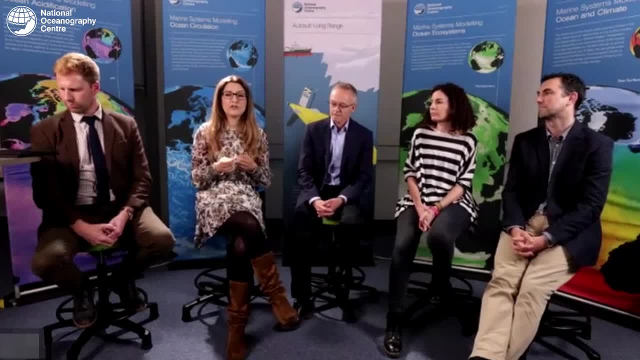 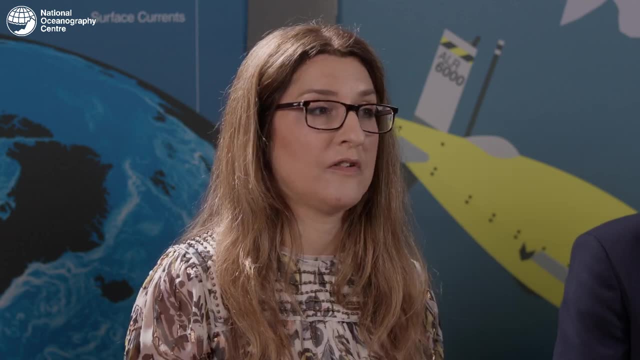 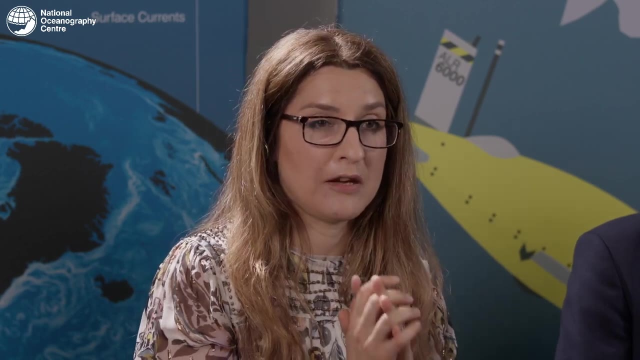 but mainly it's it's associated with coastal vegetated habitats. so these- typically we're thinking about things like mangrove, seagrass and salt marsh. so these occur around the coast and what they do? they're really good at trapping organic matter either in either- excuse me, in the 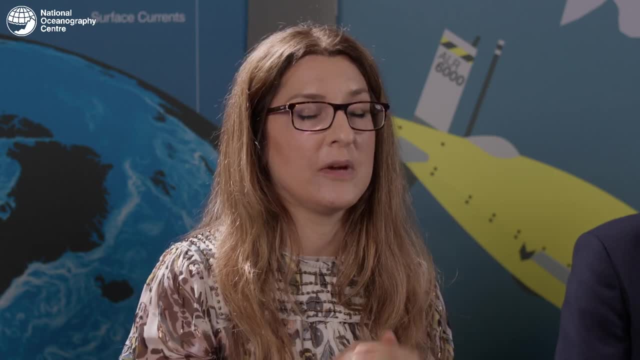 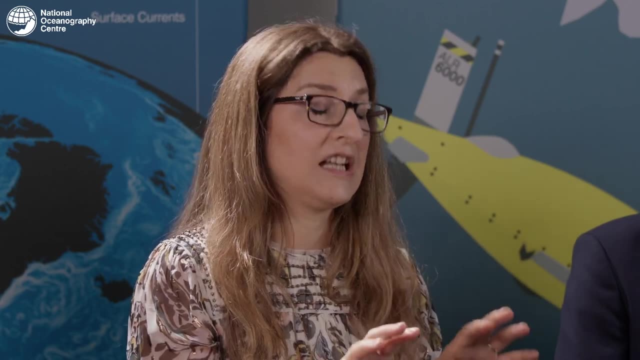 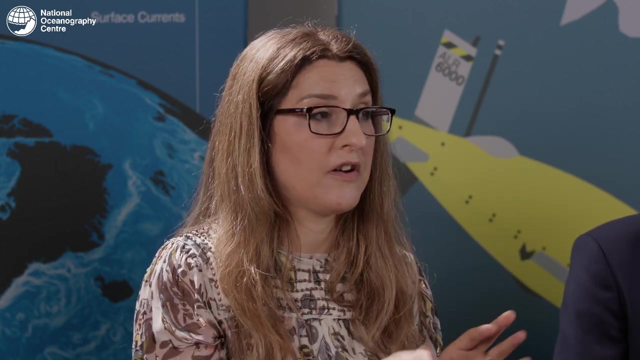 biomass of the plants or in the soils or sediments below the plants themselves, and once that that organic matter or that carbon is locked up there, it literally remains for millennia. so it's a natural process that effectively captures a lot of carbon dioxide. now, the scary thing about this: 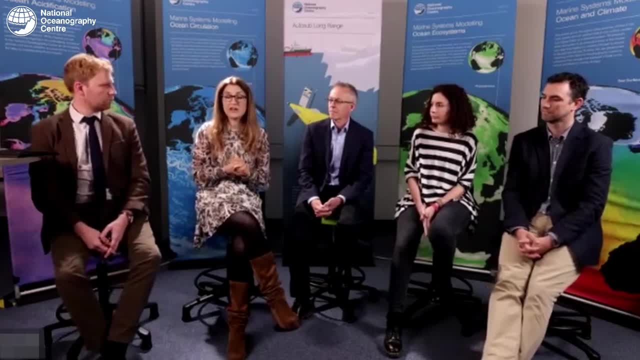 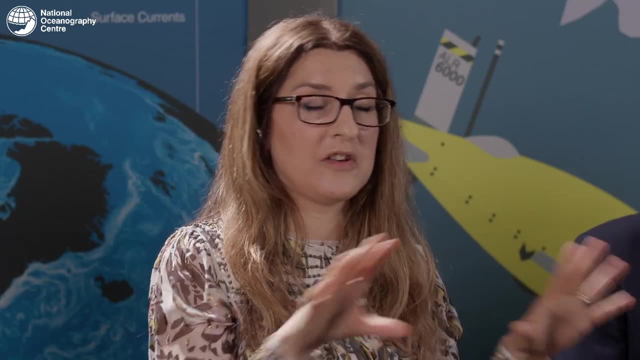 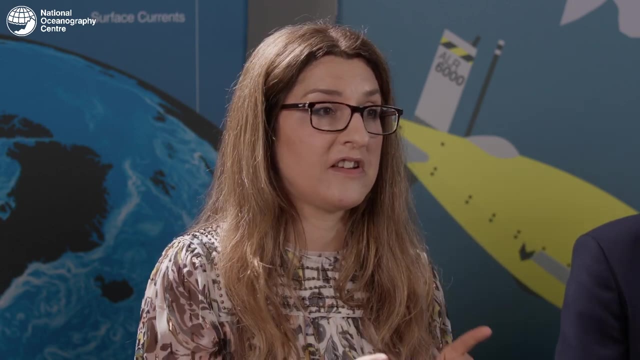 is that we are actually losing these ecosystems at the fastest rate of any ecosystem on the planet, and so I would say 101 of carbon sort of or managing this. this sort of carbon problem we have is stop that degradation. so that's kind of stage one, if you like, and then stage two would actually be to try and restore. 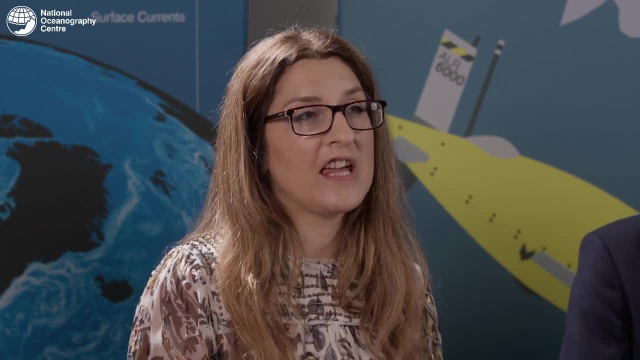 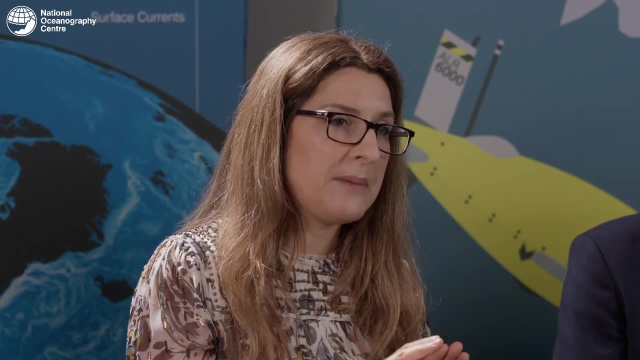 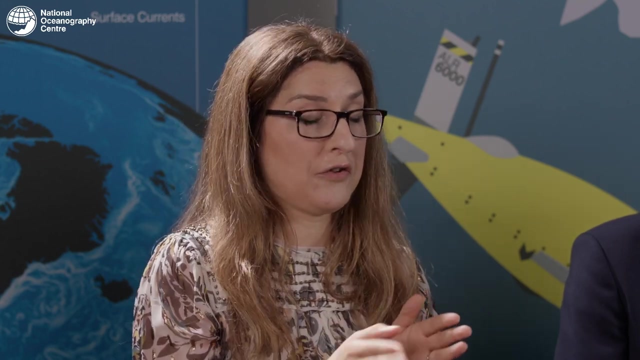 some of these habitats as well. so all together, sort of trying to manage better those coastal habitats, you could provide something like 3% of the total sort of solutions that we need to get us to the 30 sort of gigaton of carbon dioxide removal by 2030. so it's something in that order. 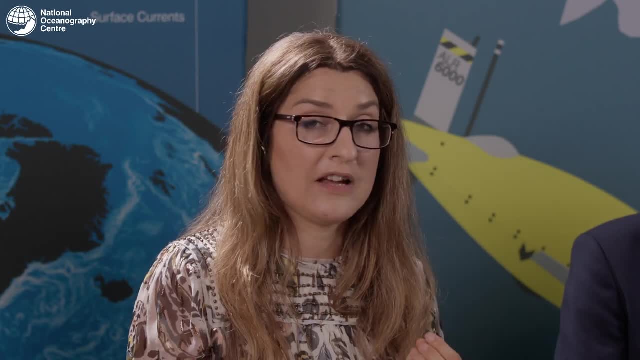 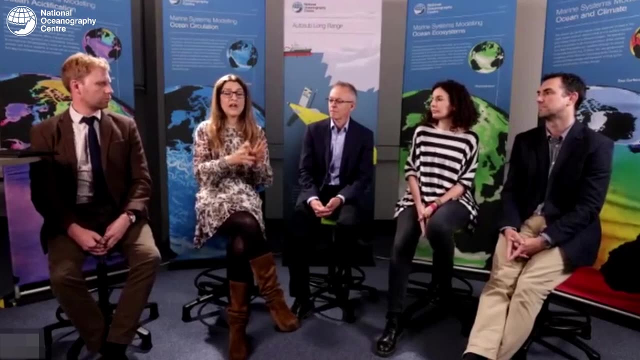 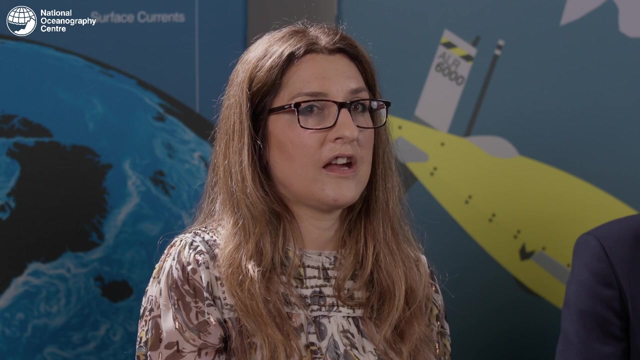 but also we need to consider when we think about the biological aspects of controlling carbon capture in the ocean. it goes beyond these coastal vegetated habitats, and so there's lots of other potential technologies or techniques that we can use, and I think we can't, at this point in time, discount anything, although some of them are more. 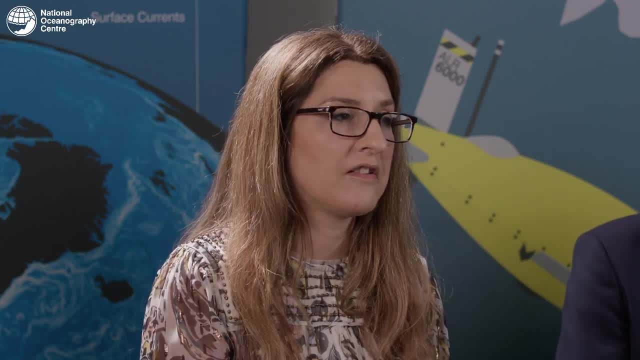 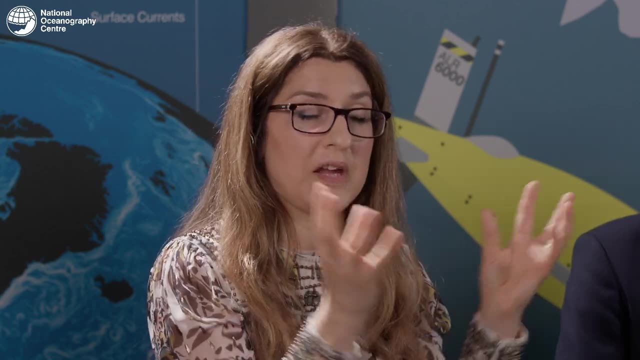 controversial than others. so, for example, I'm thinking of things like growing seaweed, because that, of course, also captures this carbon, and then there's there's some proposals that we could capture this carbon and then sink that seaweed down into the deep ocean, and there's other ideas. 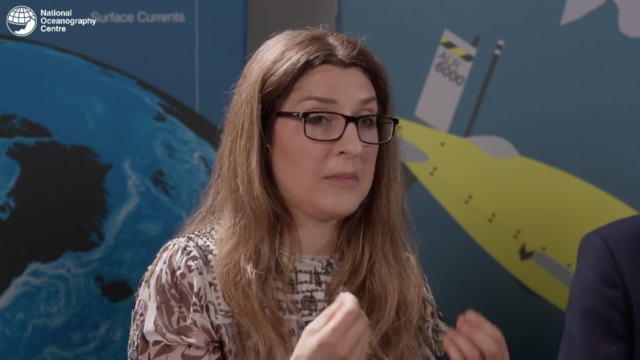 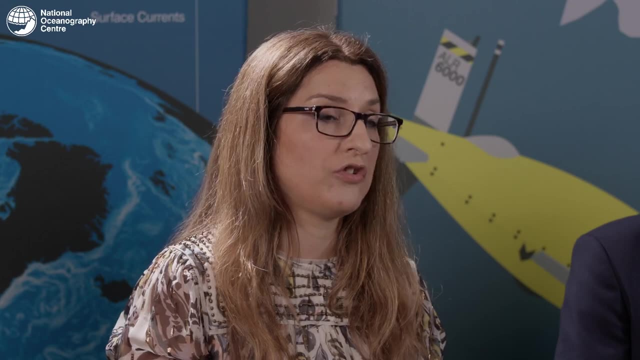 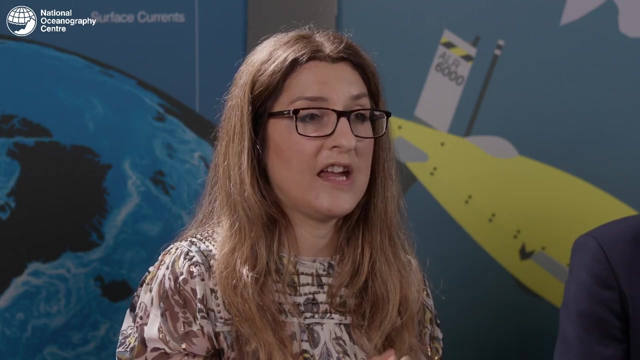 as well about things like fertilizing the ocean to stimulate phytoplankton growth, so this single cell organisms, the plants that grow in the ocean surface- so trying to stimulate those and get them to sort of sink out and capture the carbon that way. however, what I want to say is that 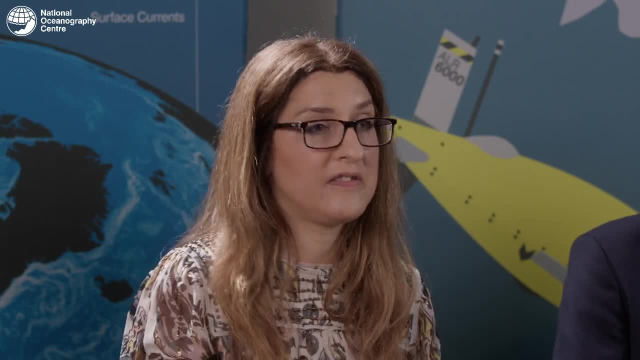 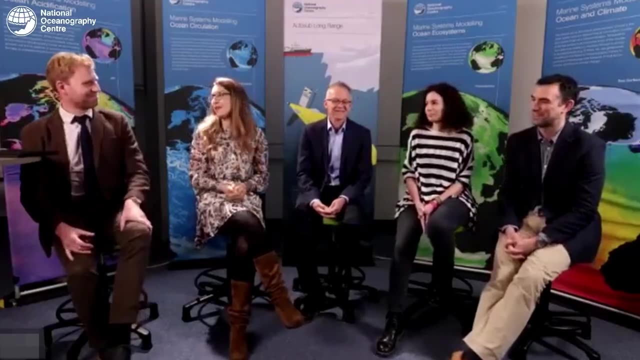 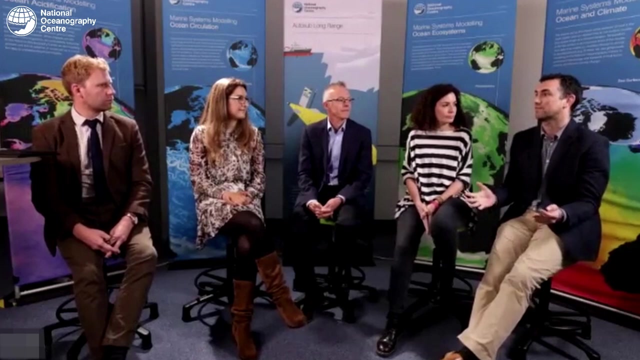 those solutions are far less well constrained, and so there's definitely a need for more research, but I don't know if Chris wants to come in as well. on the enhanced weathering, there's another ocean solution. yeah, absolutely. there's an awful lot of new techniques and technologies being explored in the ocean space for capturing and removing 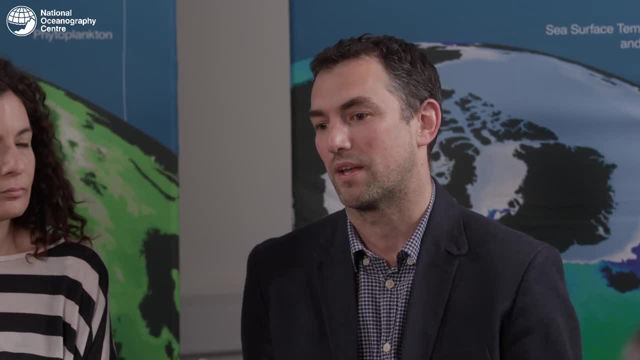 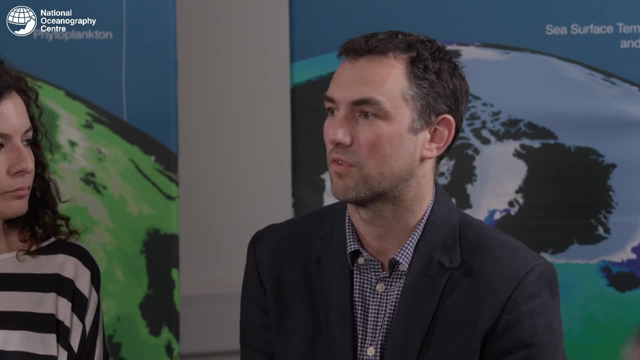 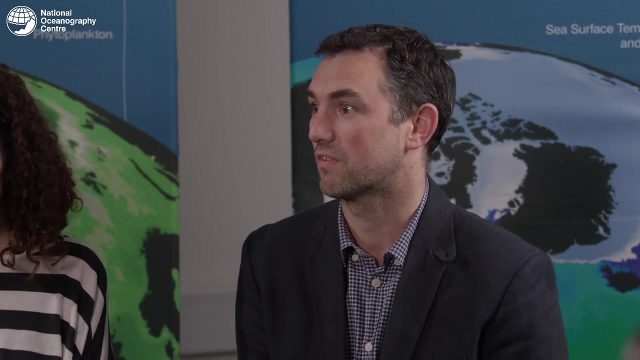 atmospheric co2, and I think it's worth remembering that the oceans are naturally absorbing co2 from the air constantly, and I think it's over 20 percent of all co2 reduced produced by human activities has been naturally sequestered into the ocean, so they're doing a fundamental job on their own. 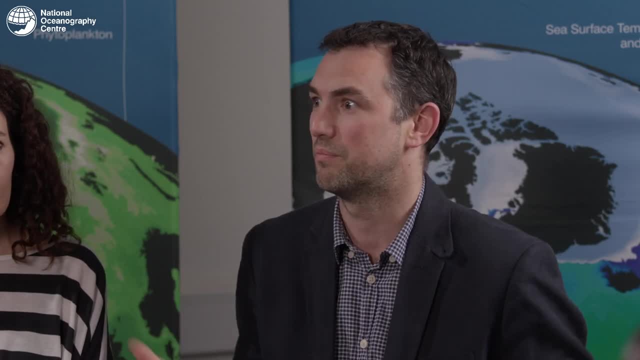 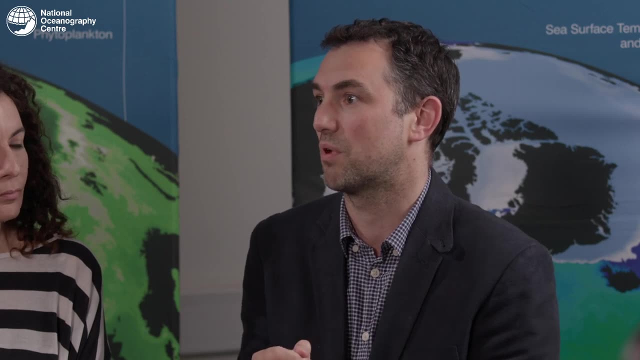 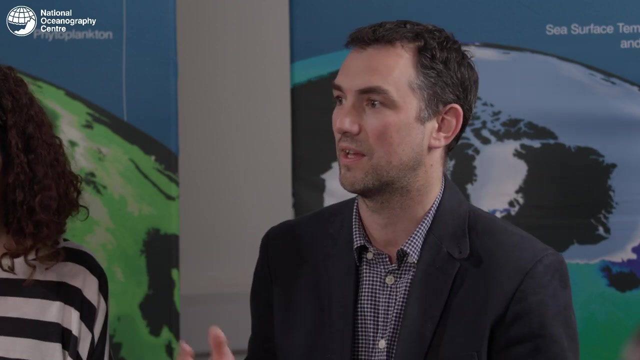 at capturing what we are emitting into the atmosphere over and beyond natural processes. so what we, what a lot of people are looking at, is a way to actually enhance those natural processes, of actually encouraging that atmospheric co2 into the oceans, where it can ultimately be sequestered in the types of air approaches that Claire's just alluded to. 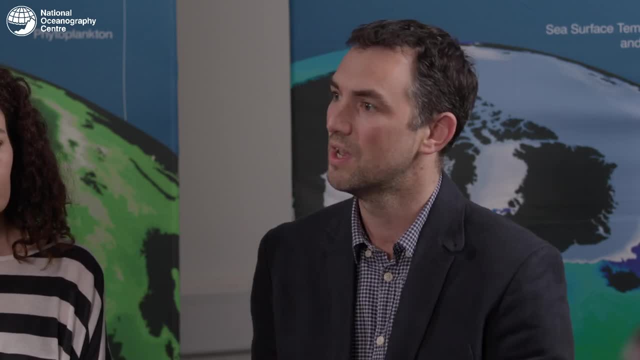 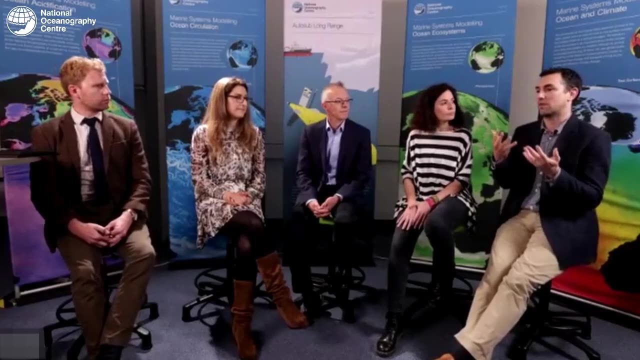 some of those are biologically driven through the productivity cycles and some of them are inorganically driven through natural processes and mineral formation, mineral dissolution processes, and so this uh distribution of rocks and minerals, either in beach environments or actually applied into open ocean settings, is one proposal to naturally enhance alkalinity. 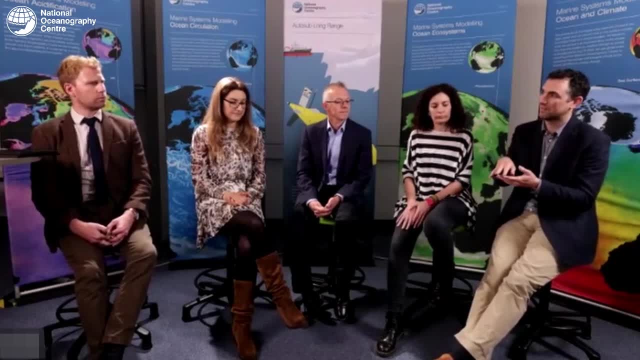 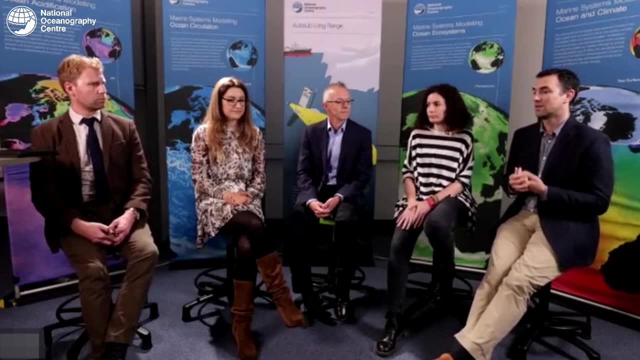 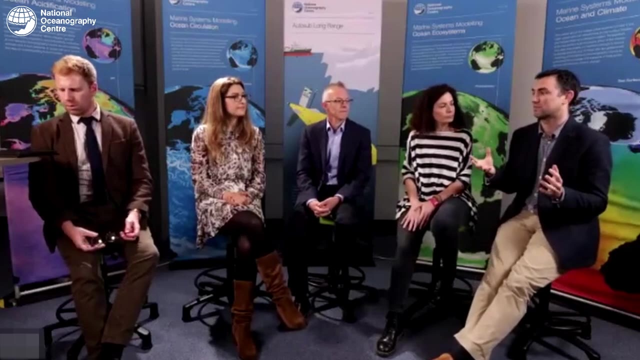 which would encourage this drawdown of co2 into the sea water and at the same time offset the potential ocean acidification as a consequence of that process. but again I echo what Claire said: there's a lot more research needed to be done into the environmental ecosystem impacts of those. 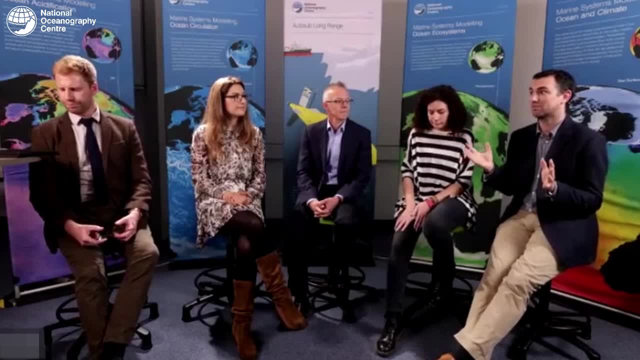 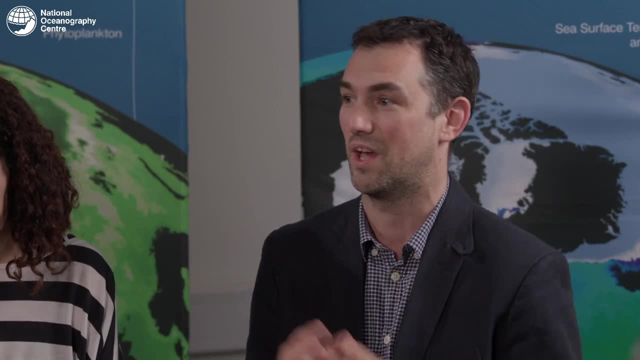 approaches, because these technologies are very new. they have potential to help, but not as much potential as reducing their emissions in the first place. so everything we've discussed there has to be an equivalent to the reduction of co2 in the ocean. so the next slide, please. 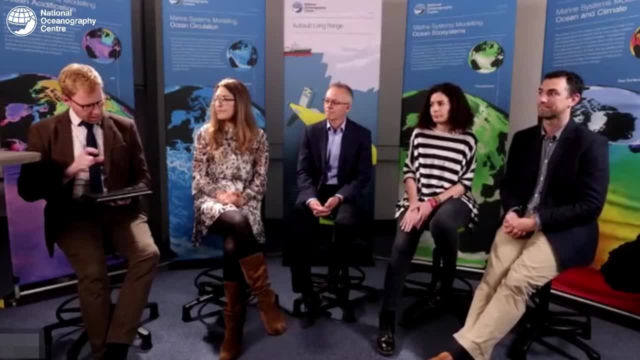 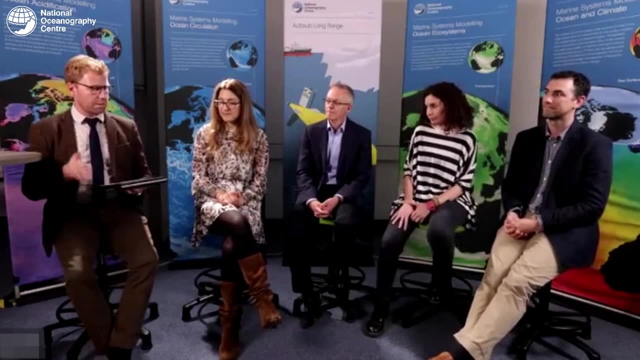 yeah, that that makes sense. you know, when I look at this sort of from a top level view, it's quite easy to see a range of these solutions and sort of put some in the kind of engineering pots and then the sort of natural based solutions. I guess I'll just 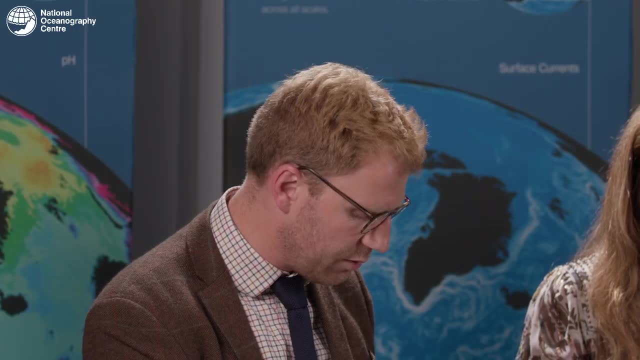 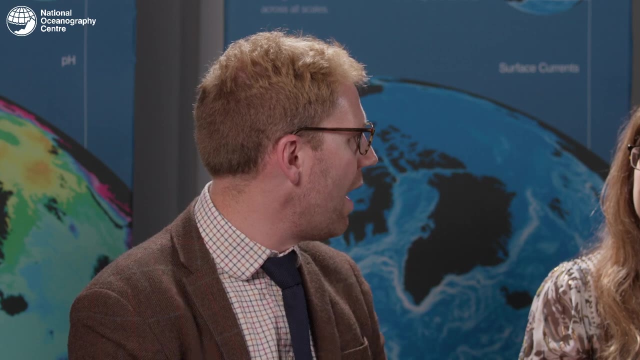 throw this out there, you know. thinking about it in that way, you know where, where, in your view, should we be putting the focus? the investment, the government horsepower? you know, if we were to pick, pick two, you know where would that focus be and how should that focus be directed. 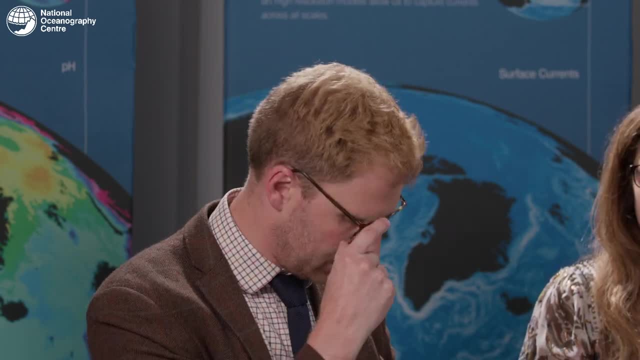 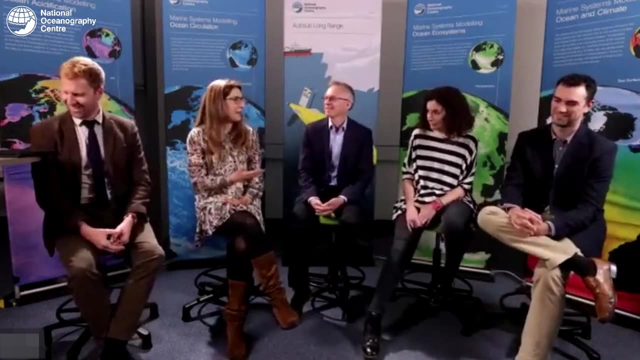 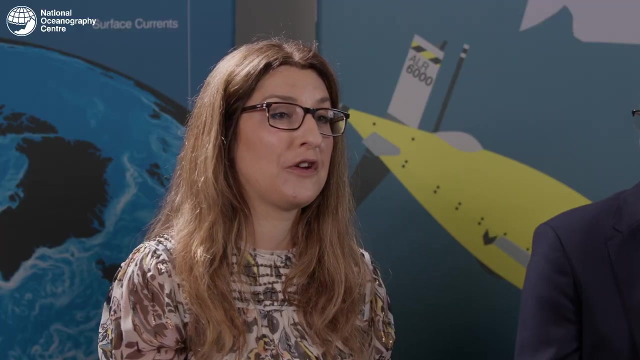 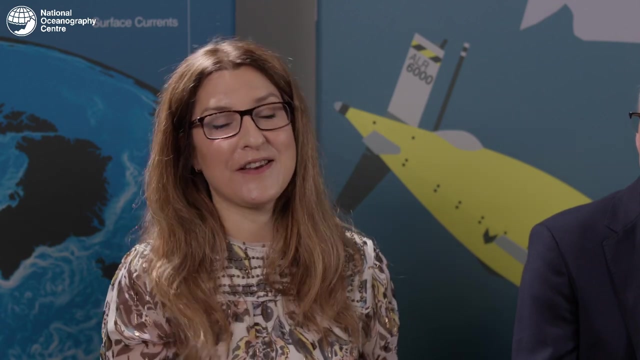 to really accelerate that, I guess, the rollout of some of these solutions. I can make a comment just to start, and I think so. my colleagues on the panel may not agree, but personally I would definitely make one of those two: restoration of our natural environment and the reason why some components of the panel might say, no, that's, that's not where I would go. 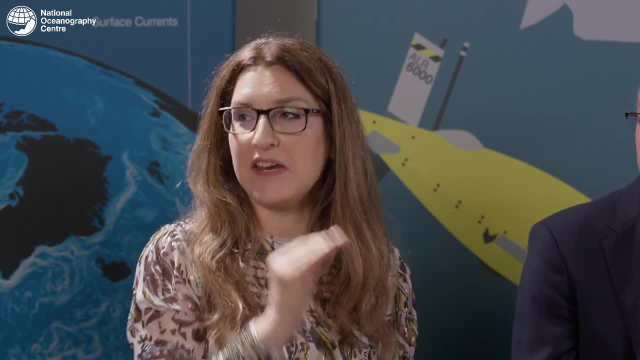 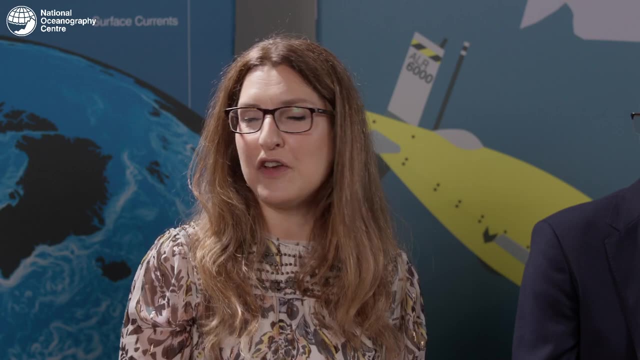 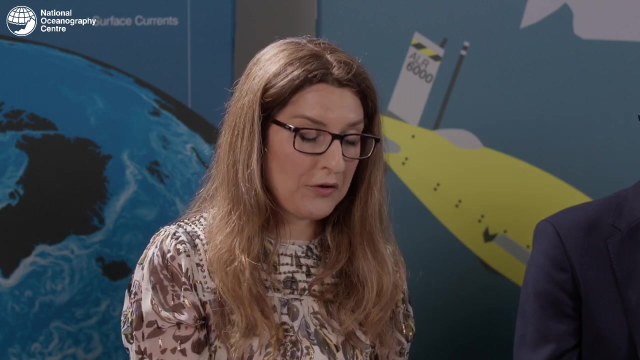 is because perhaps it you know, other technical technologies have greater potential to to capture carbon. however it's, it's known as a no regret scenario. you know you're restoring the natural functioning of the the marine environment, and this doesn't just come with the capture of carbon dioxide, it also comes with a host of other benefits. 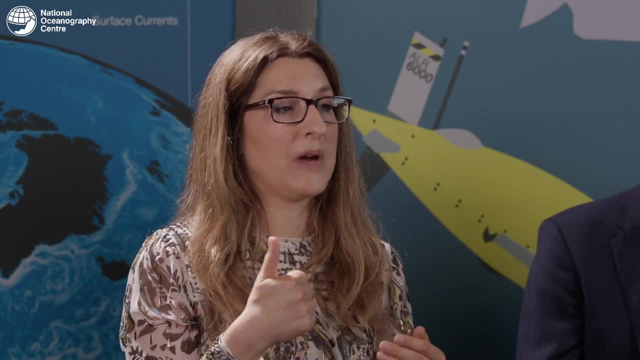 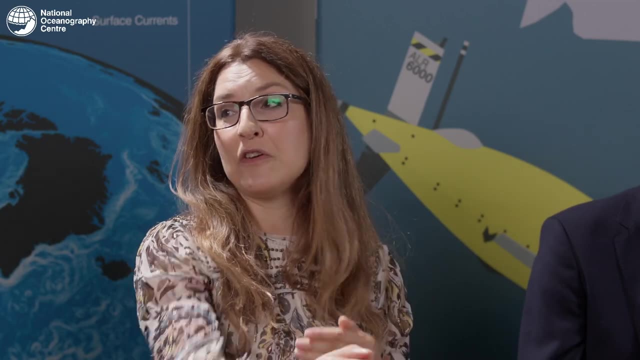 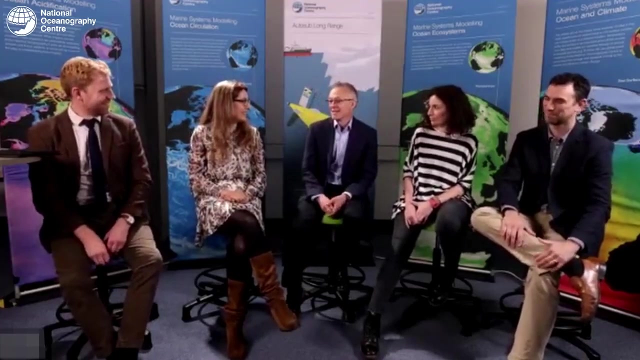 to society. so I think, just restoring those habitats and we get back gains on biodiversity, sediment stabilization, you know buffering pH, you know buffering pH, you know buffering pH. the list goes on and on and on. so but yeah, yeah, I thought you might go there. yeah, but no, it's true. and it's not just that, it's, it's storm. damage. you know classic ones in the sort of monsoon damage. in Pakistan they've restored 50,000 hectares of mangroves and it's in those areas we restored. the damage from the last monsoon was minimal compared to those areas where it was exposed, so there are those extra benefits for me. 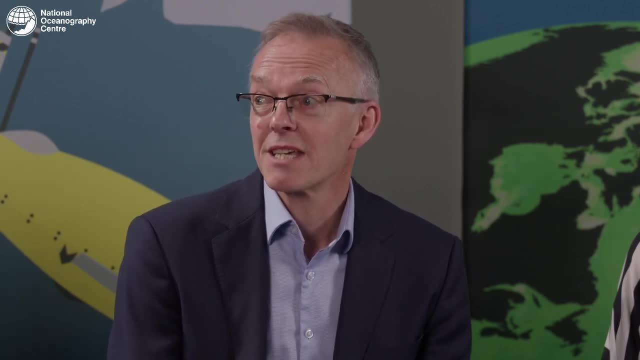 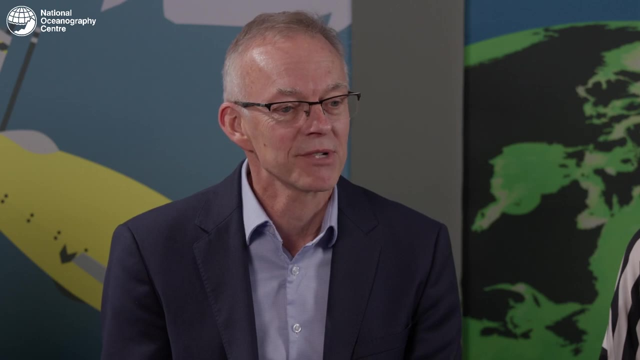 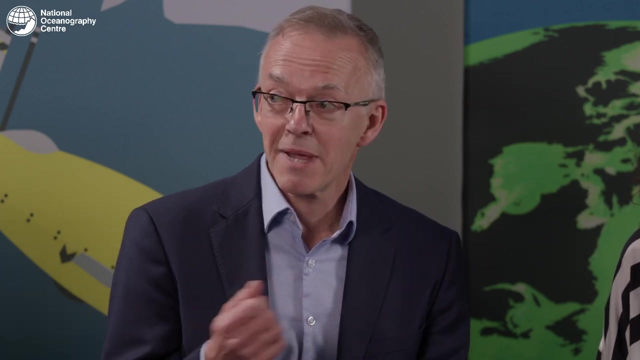 in terms of instant or a quick thing. it would be the rollout of CCS which we are seeing now. so the UK government and the US government have committed to this Norway's rolling out new programs around carbon capture and storage because technologically it's available now it's economically it's going to 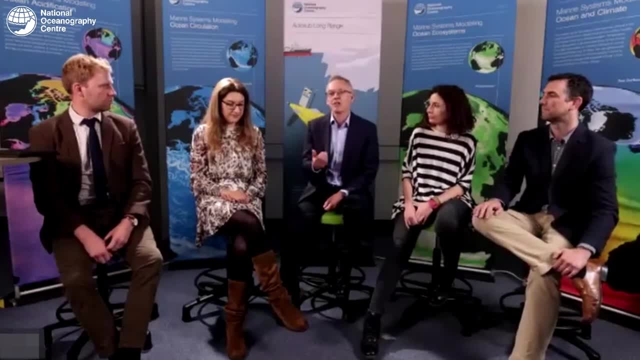 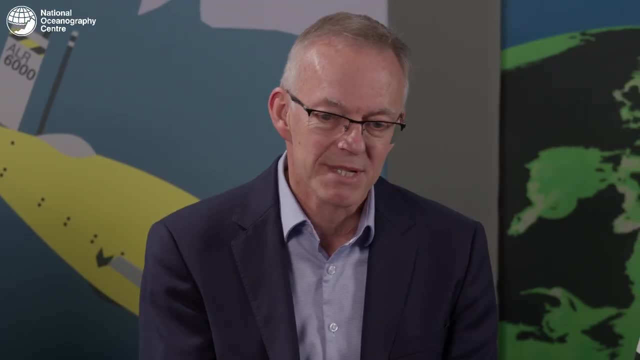 be quite interesting in terms of how it stimulates reuse of areas such as the areas of in north Scotland, because there's depleted oil and gas reservoirs. we're seeing a natural ramp down in hypercarbon production in the north sea area. you know, by using it, by developing a CCS industry. 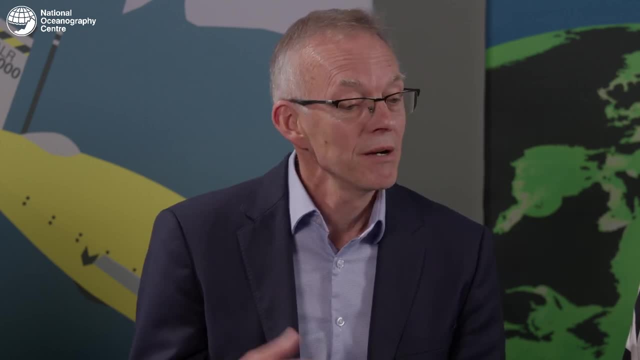 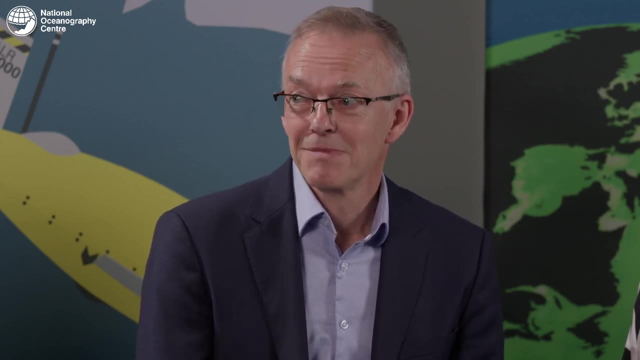 if we can bring jobs back to those areas. so, from an economic point of view, we're seeing it in the US. the US are now looking at using the bill for Mexico. so it's a proven technology. it has its, you know, proponents and and opponents. in as much as as Chris might be able to talk to is this: we. 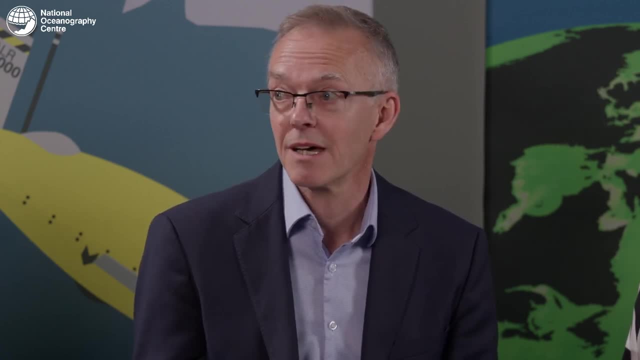 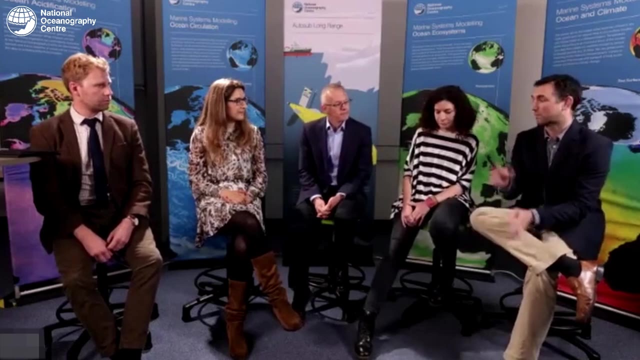 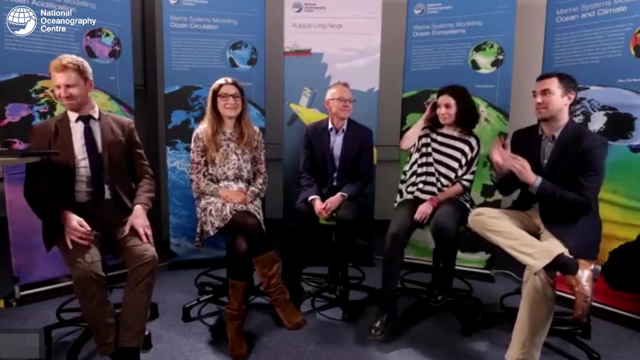 need to be able to demonstrate to the public it's safe. and you want to refer about how we've done the monitoring and verification. yeah, yeah, absolutely. I think. just before getting that done, I'm just going to say there are quick wins, there are win-wins, but there's no single win, and I think it's perhaps leading to say which. 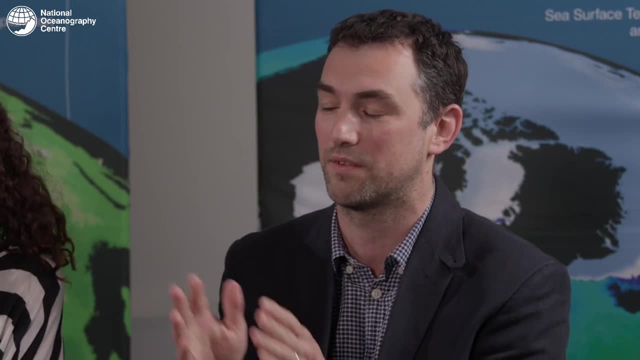 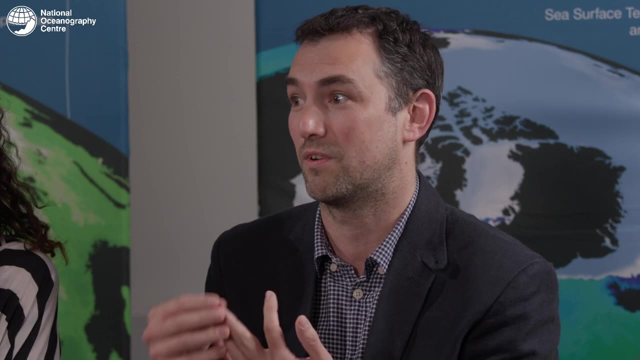 one or two would be achieved, because we need to look at them all. I think you can't identify a single approach, because we need everything. we need every strategy on the table. we need to be investigating these. which has the most potential, which has a long-term potential and which are 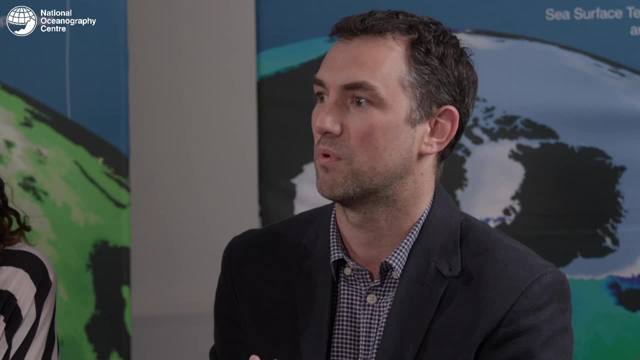 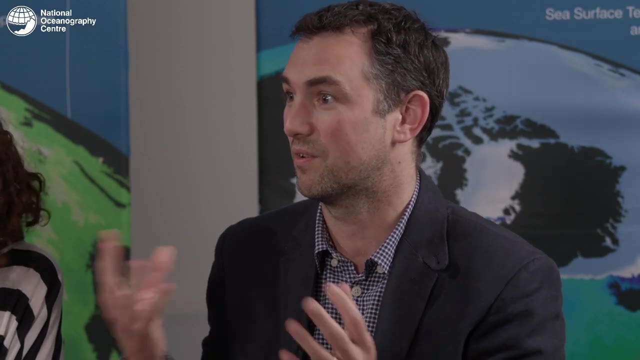 non-viable, and this is where this, this issue of reporting, monitoring and verification, comes into play, because we need to understand what the potential impacts could be in a long-term situation, but also to the ecosystems that surround them and as you alluded to in the opening. 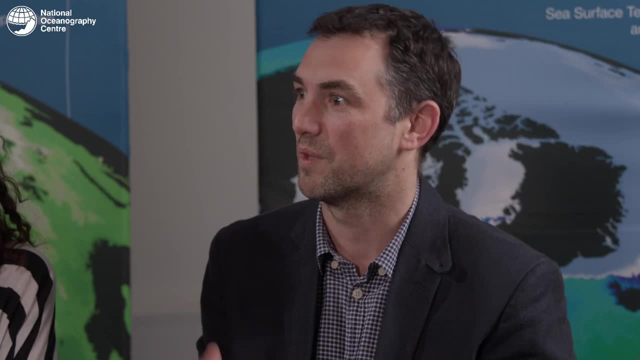 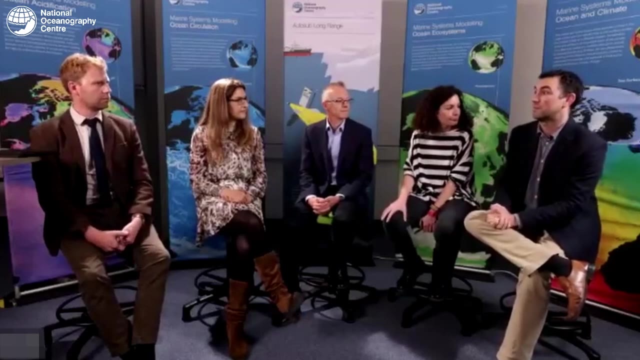 statements. you know, we need to know that these are, these solutions are not going to become the problems of tomorrow or even the problems of here and now for the organisms out in those environments. and to that end we have been developing here at the NSC in a whole array of sensor technologies. 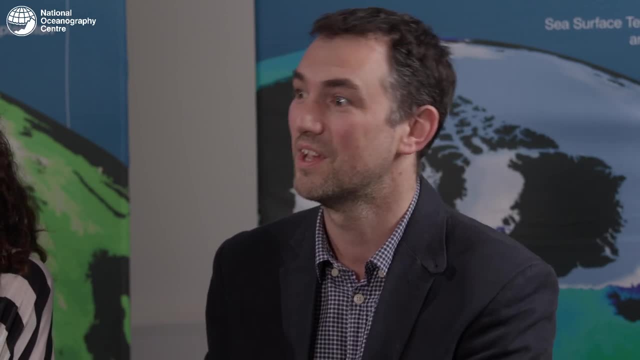 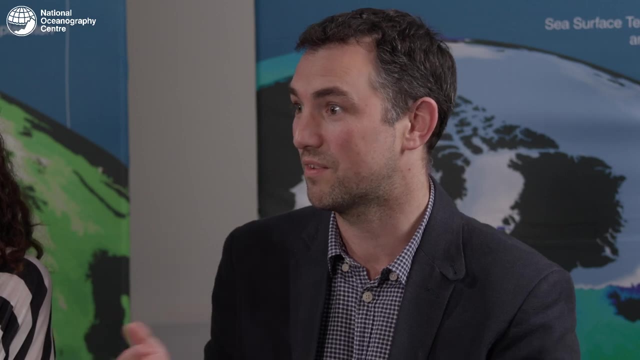 that can be deployed for very long periods of time in the bottom of the oceans, in the surface oceans, in a whole array of personal environments. so we need to get those technologies demonstrated. we're going to be enhancing them and actually deploy them in the settings that these techniques could. 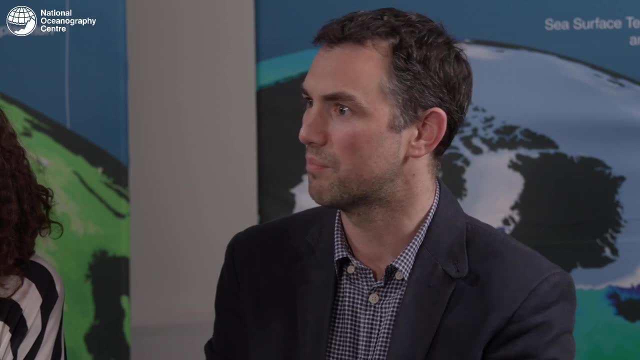 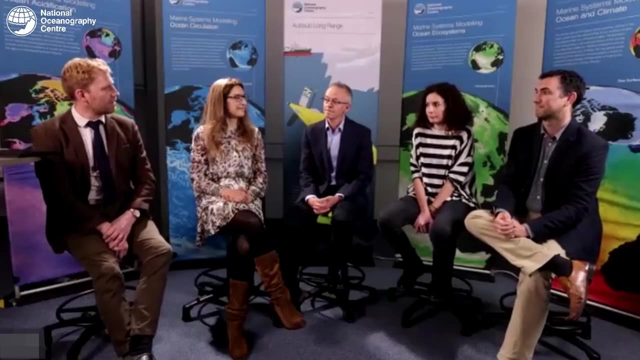 be actually applied to demonstrate their capability for long-term assessments, both ecologically and in the context of looking at the co2 sequestration potential? no, thank you. so, Michaela, you, I guess you're in the envious position here of looking at all these solutions and trying. 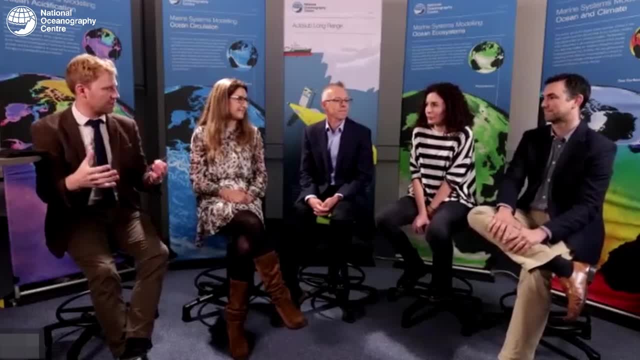 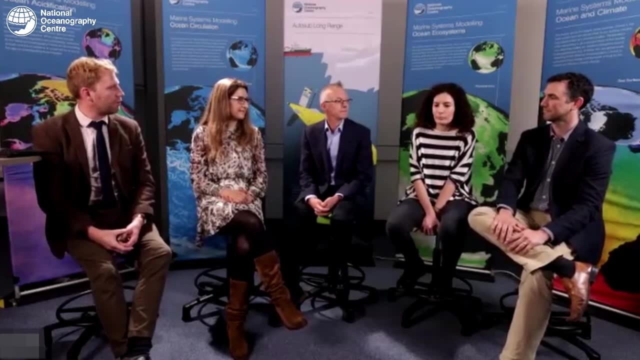 to take a view on the impact of these going forward on the entire ocean system? what's your take on on these different types of solutions and the potential impact that they may well have in the wider environment? I think we are missing one of the possible ocean solutions. 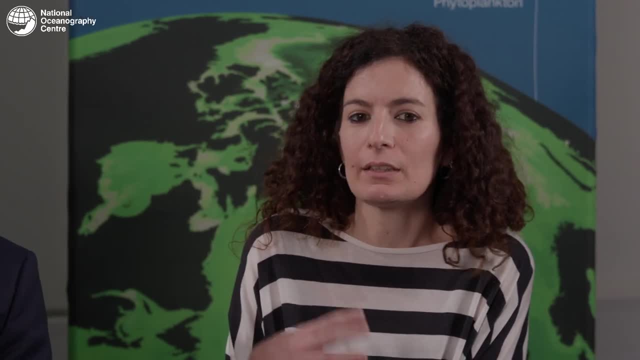 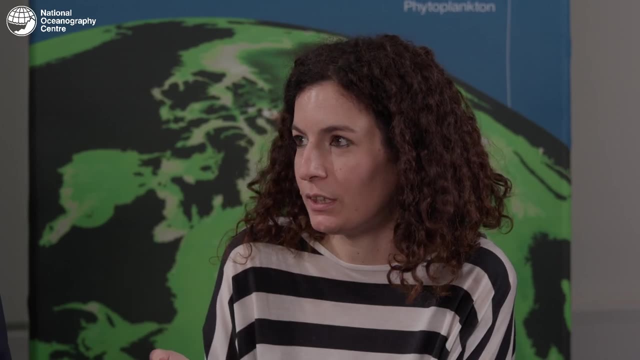 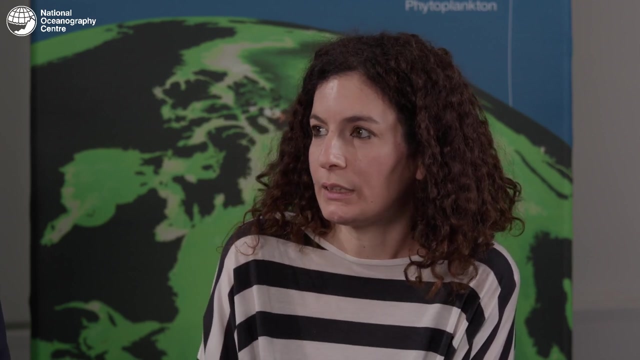 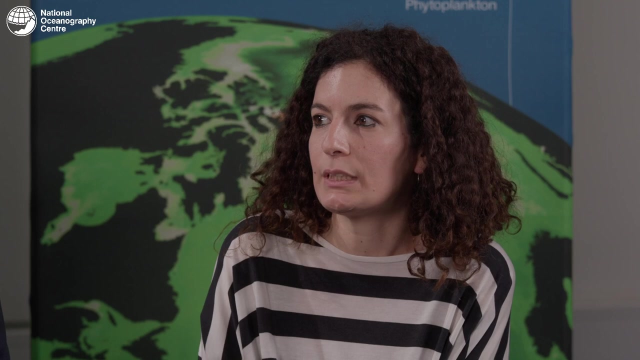 which is marine renewables, because it's we can mitigate, we can capture the co2, but we have to reduce the emissions in the first place. so and there are several different types of marine renewables that they are under development right now, from tidal stream turbines, tidal barrages. 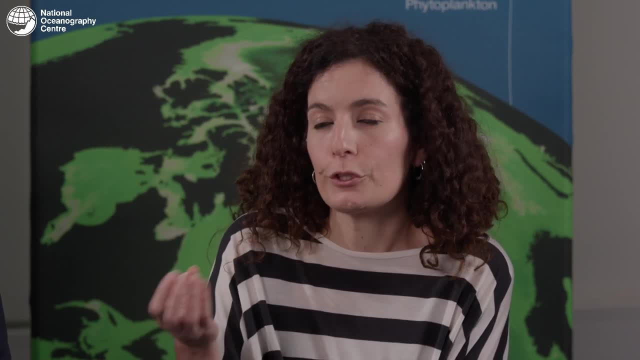 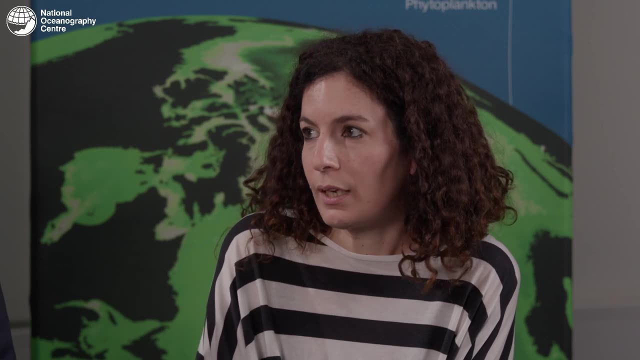 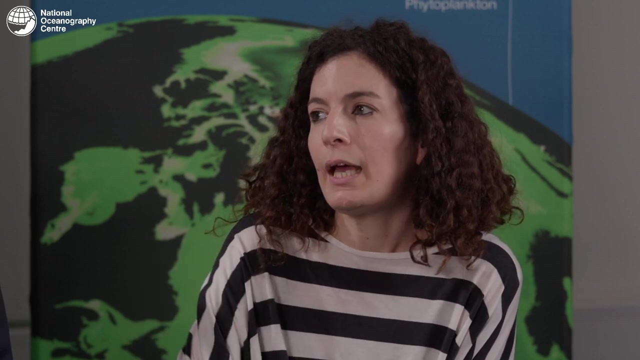 wave converters, and and then also offshore wind farms, which is probably the most mature one, and it's the one that we are gonna see in the next year. actually, we have already offshore wind farms, but they are gonna move further offshore, they're gonna become floating, and I think 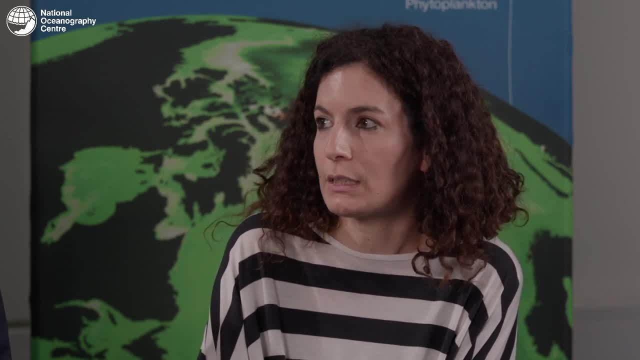 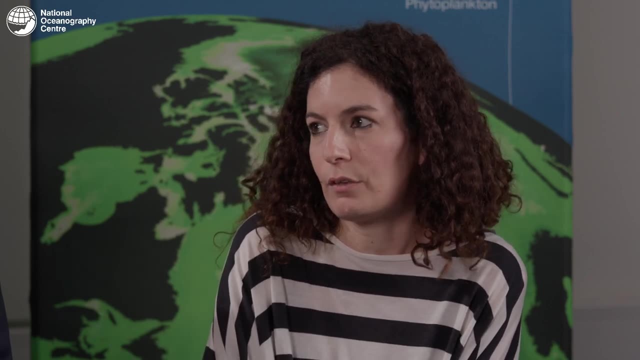 that in the next few years we are gonna see a big expansion of this and then probably after that, maybe tidal stream turbines and so on, because we need all the possible technology that are out there. just following off that, I'll stick with you, if I may, Michaela. you know you could take a really 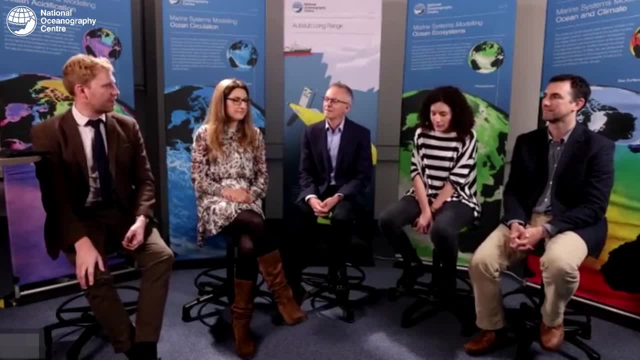 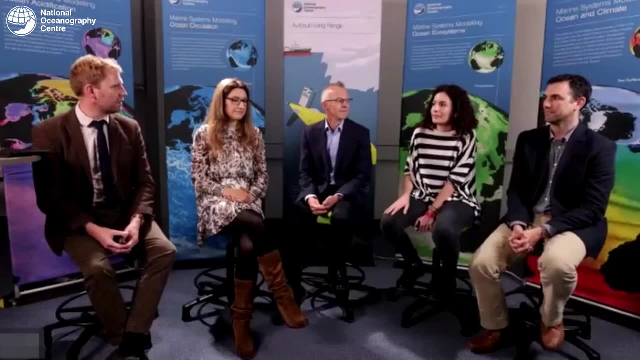 cynical view of this and say: you know, we've built 60 years of oil and gas infrastructure all over the place and, you know, whilst that might sort of decommission and drop off, we're going to go and stick a load more metal in the, in the sea and all the vessels that need to go. 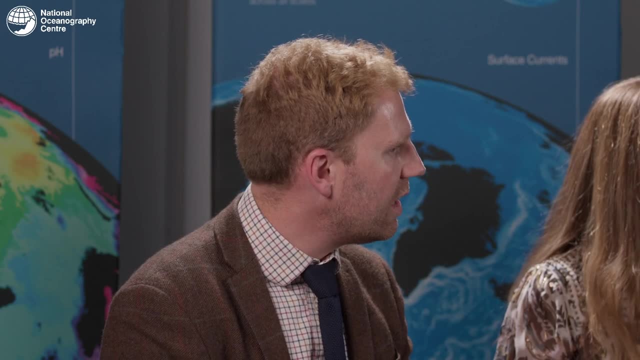 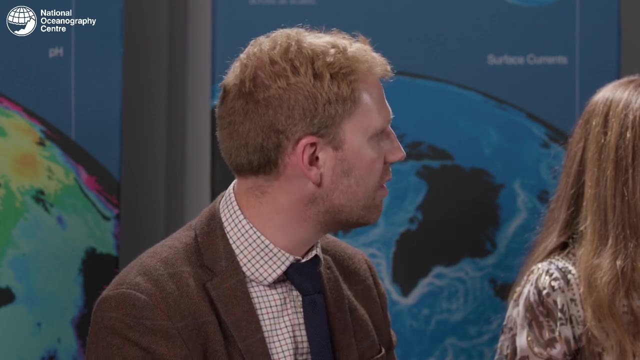 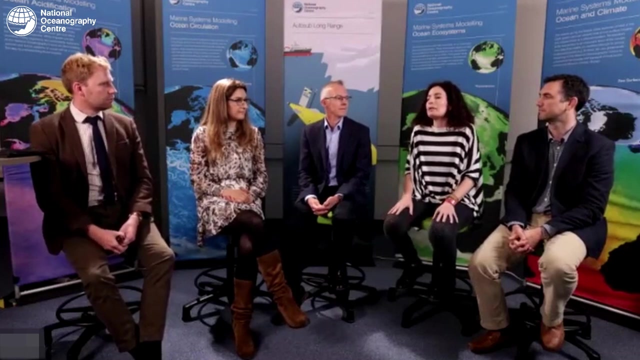 out and all the noise and cable arrays you know in. in your view, what do we need to be really conscious of when we do that, just from an environmental impact perspective? yeah, so I think that the problem of the oil and gas energy industry- I mean the main problem- was not the 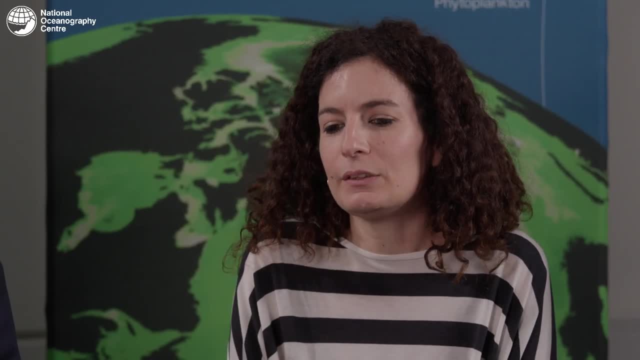 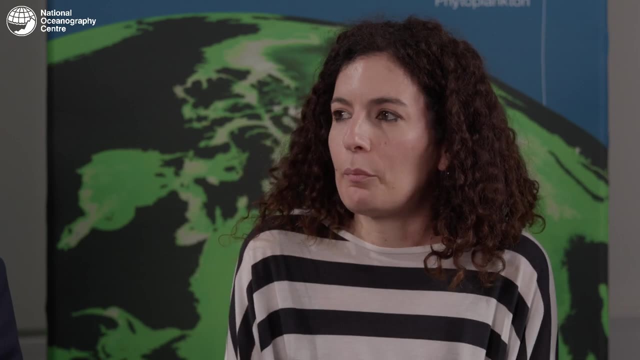 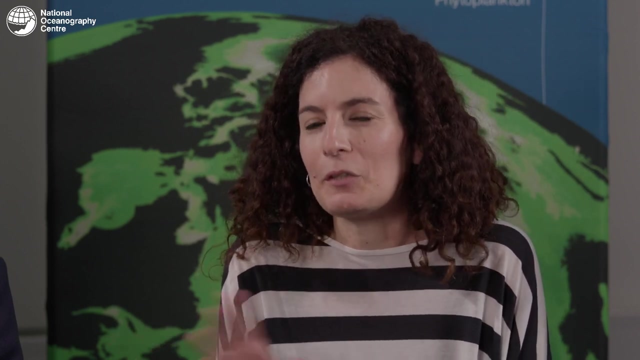 infrastructure that is at sea. the problem is that we need to move away from that because of the greenhouse gases emissions, basically, and with muddy renewables we don't have that. at the same time, if we have an accident in a wind farm, something breaks- we don't risk having any. 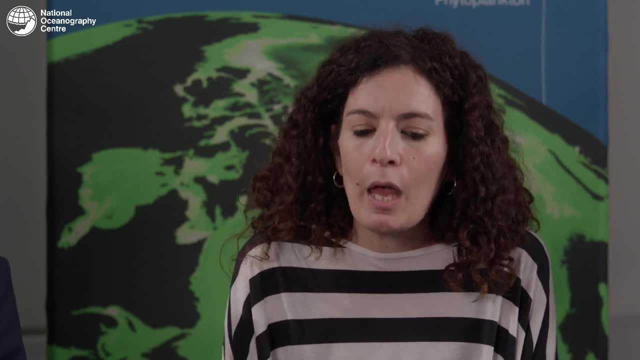 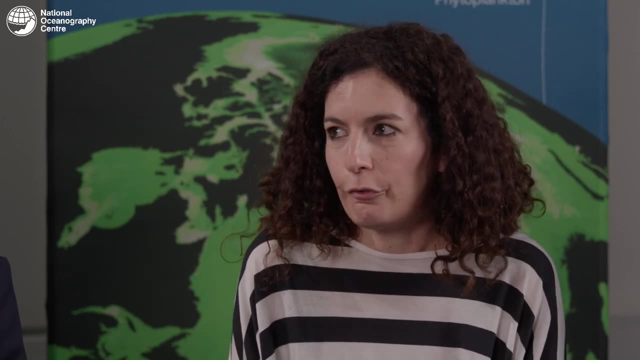 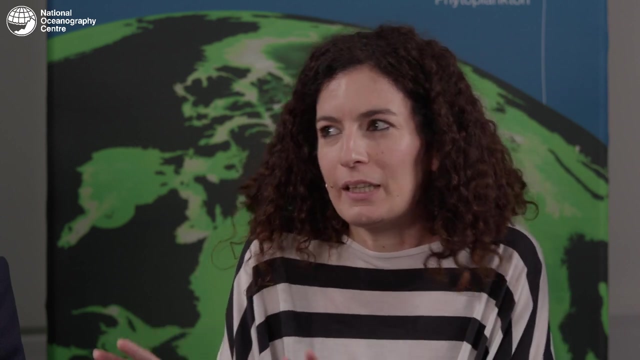 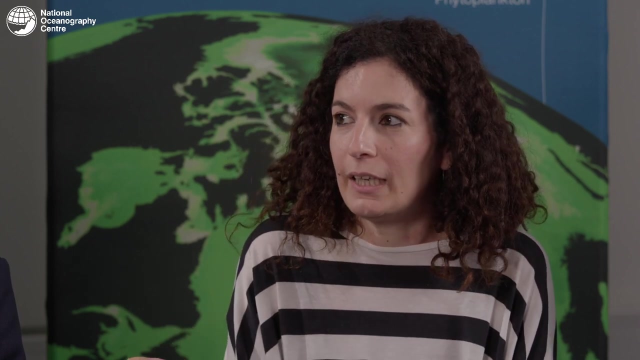 oil spill pollution, chemical contamination and so on. but going back to the infrastructure itself, it's true that we want to be extra careful and we don't want to exchange one environmental crisis with another one. so I think it's it's a problem of of the scale of the development, because 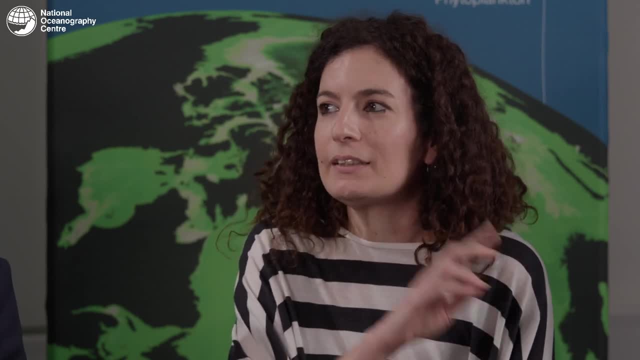 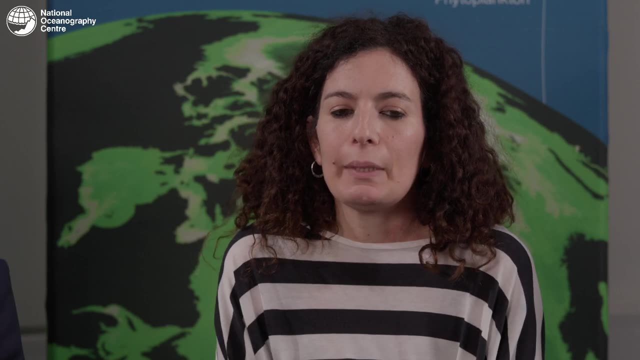 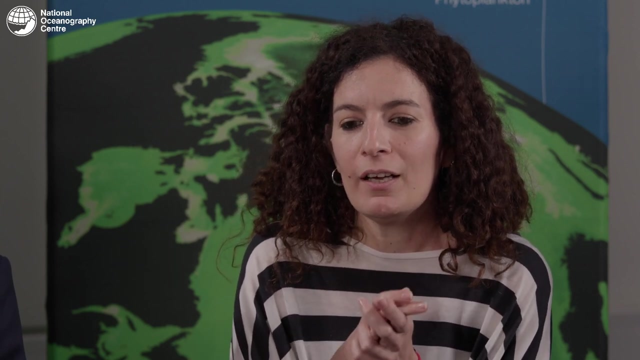 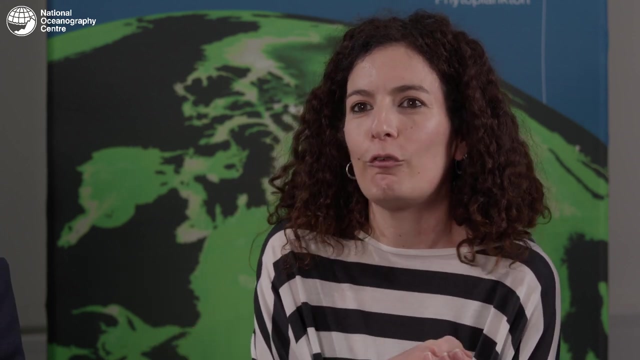 if we are going to put one wind turbine, one tidal stream turbine, the environmental impacts are going to be small, negligible. the problem is that the future plants are to have like 40 gigawatts of wind from, of energy from offshore wind. 40 gigawatts is the equivalent of 10 big, very big. 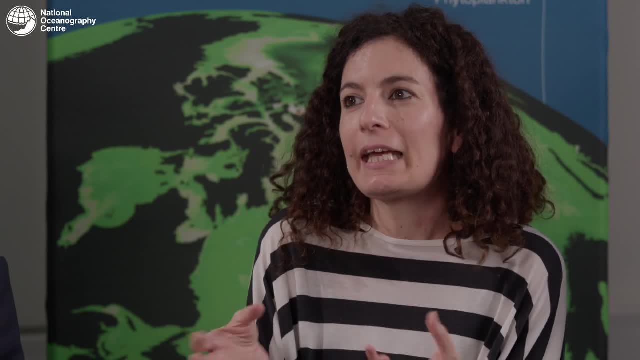 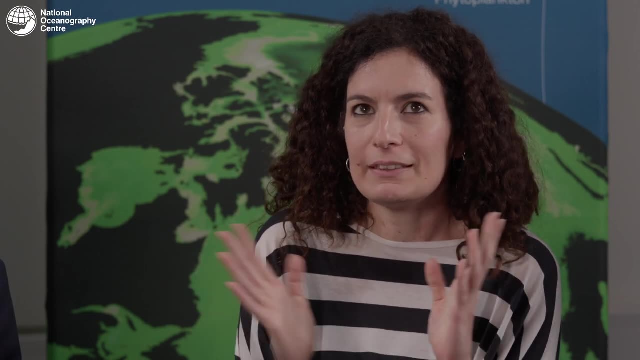 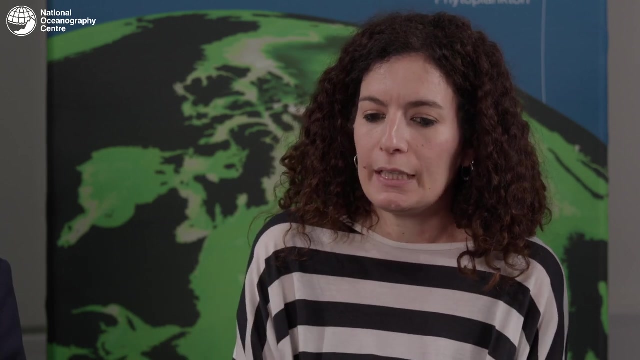 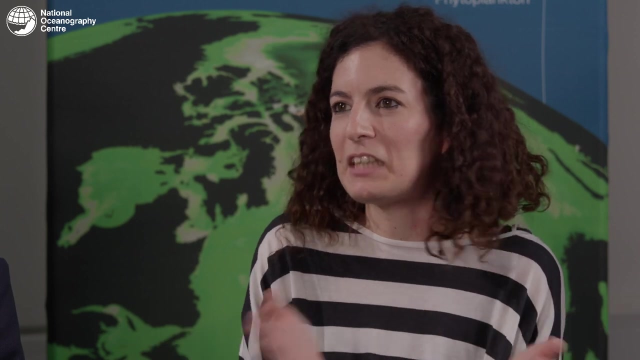 power plants. so extracting that from the north sea can have an impact. it means putting to the north sea 7 000 turbines, something like that, and the difference with the, the structure of the oil and gas platforms is that in the- I think in the old world- we have like 7 000 platforms. 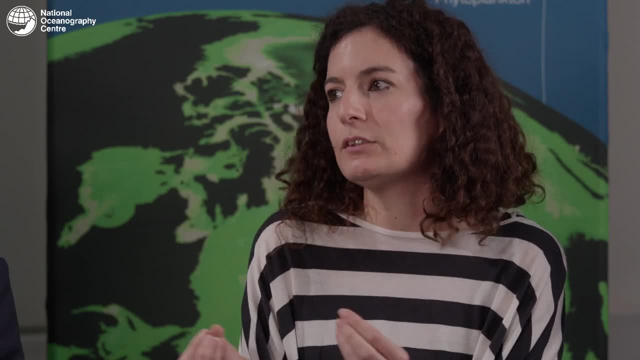 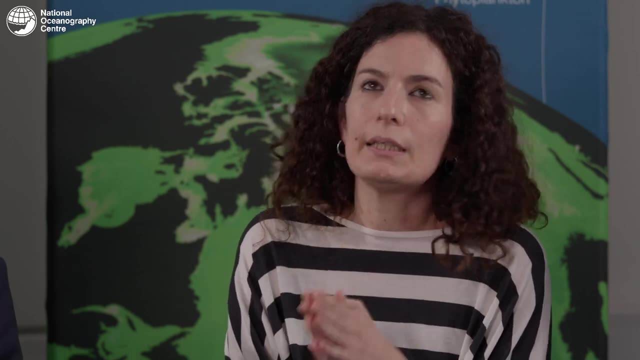 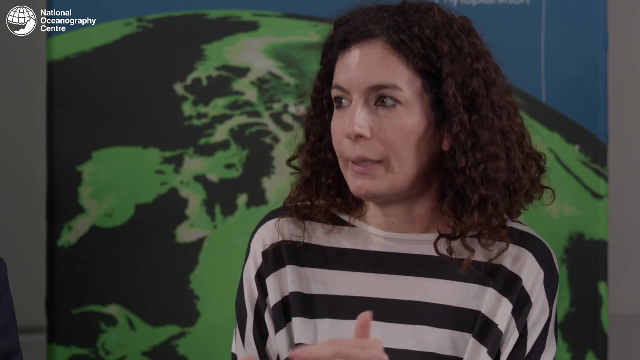 and instead we are putting 7 000 wind turbines in the north sea, or at least this is the plant. so what? I'm not saying that this is gonna be, it's gonna be wrong or it's gonna have a negative effect, but we need to understand what is going to happen in advance, and we can do that because, I mean, we are. 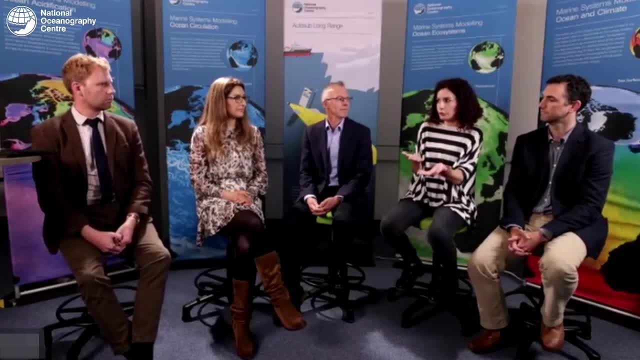 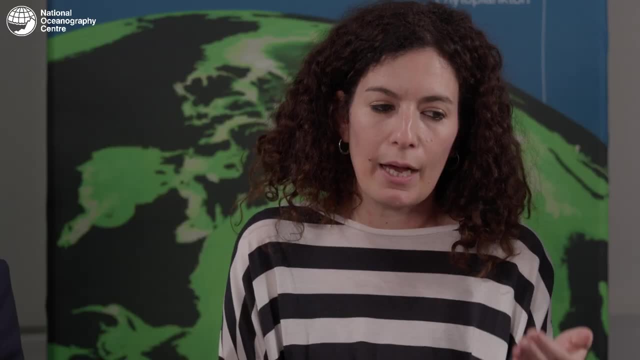 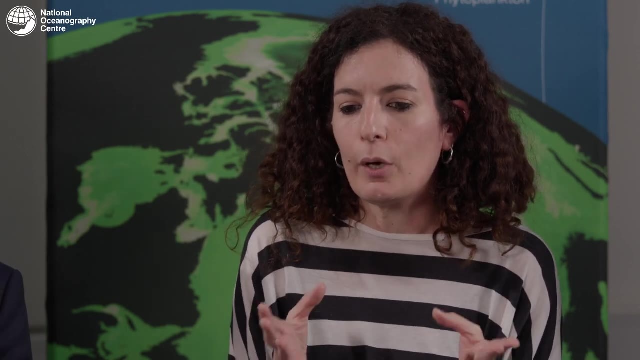 not able to measure what is going to happen in the future because we can't. but we can use ocean models to predict what is going to happen. I don't know if people are familiar with computer simulations, but an ocean model and a computer simulation simulating what is going to happen in 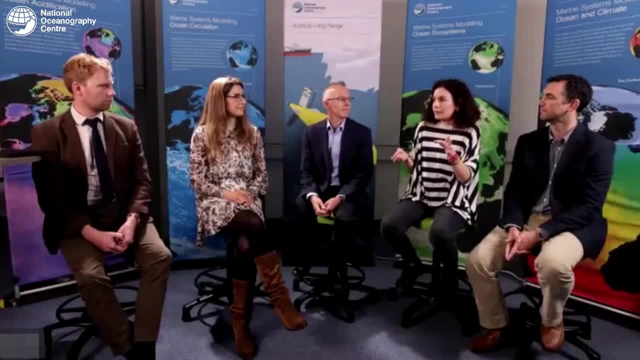 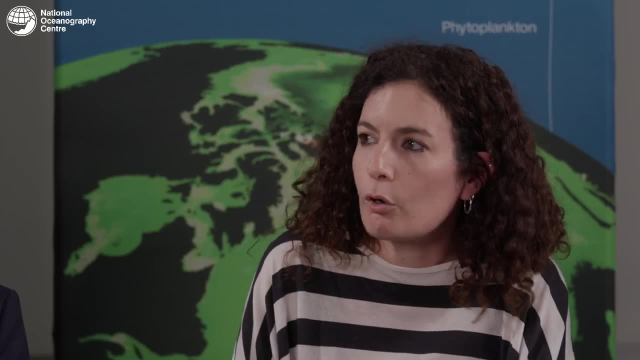 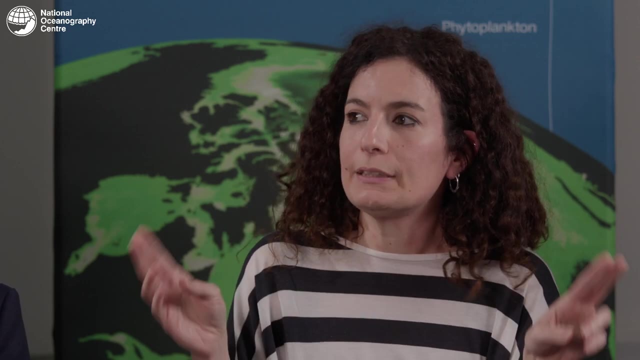 the future is similar to what we do for the weather forecast. we do the weather forecast for tomorrow and we can use a similar system to predict what is going to happen tomorrow, but also in the next decades, in the ocean, and we can do that for different scenarios. so, for example, what is going? 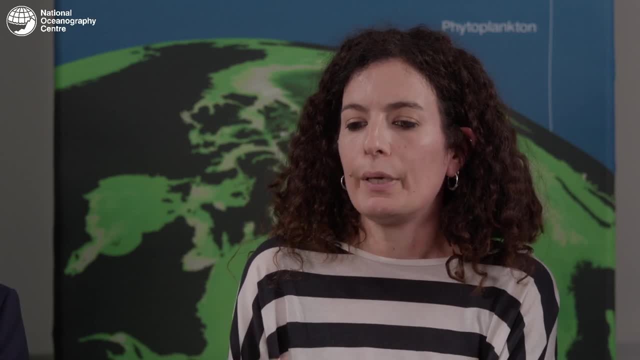 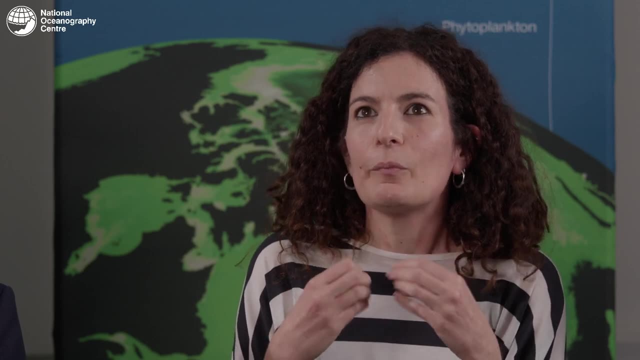 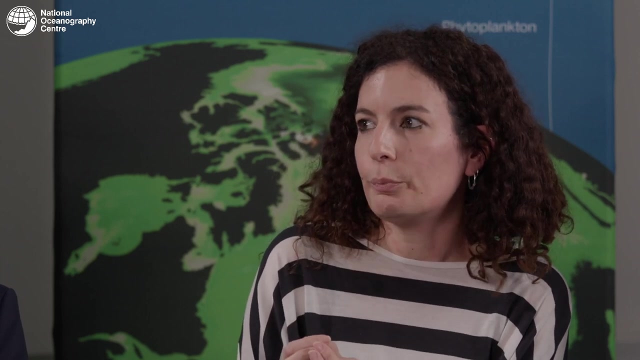 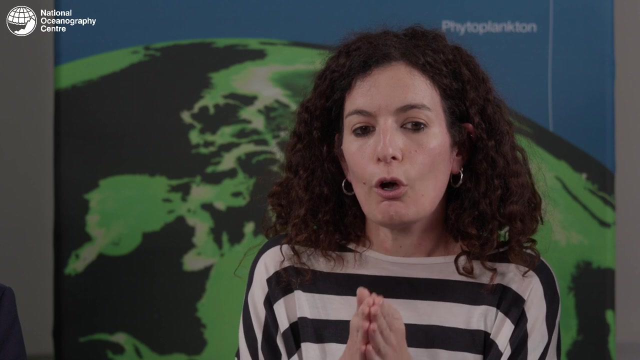 to happen with climate change, or what is going to happen if we put 7 000 turbines in the water. I mean, we don't have those models yet. actually we are working on how to tune, how to modify our models to be able to predict that, but it's something that it will allow us to know if 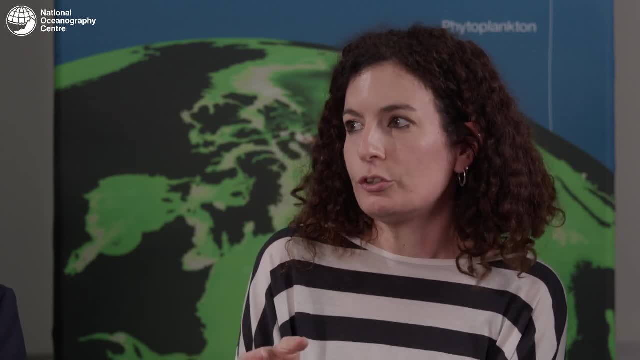 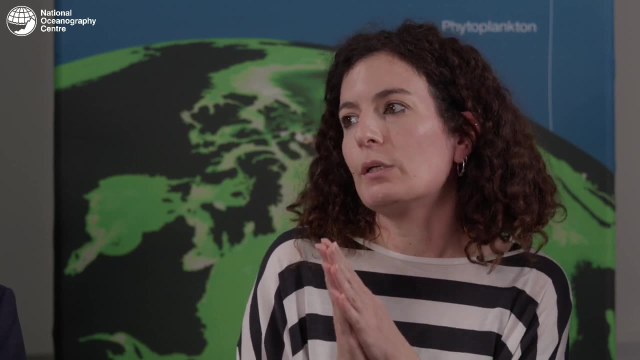 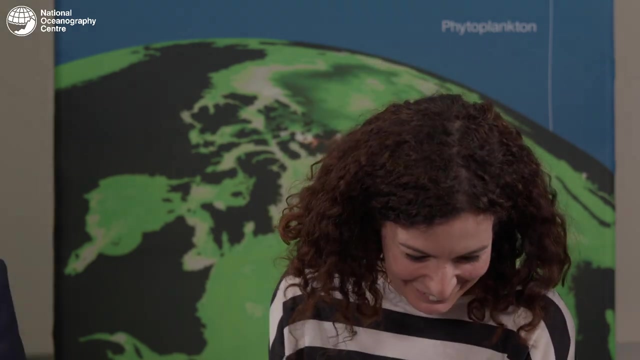 those changes are acceptable or not, or which are the locations that are best for that technology, or the ones that we should avoid, for example. I was going to ask you what is the answer in 10 years time, but I won't. I'll save that. thanks, that's great. so, Chris, I'm just going to direct this one to you for me, so obviously. 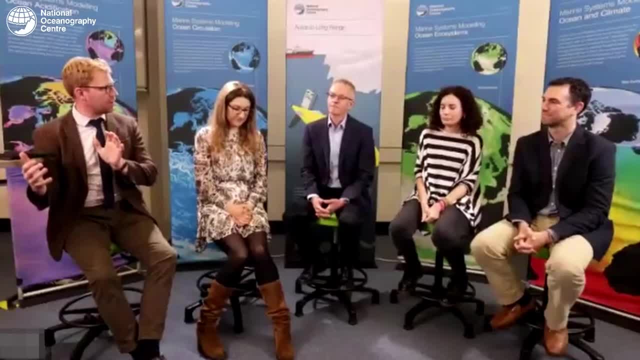 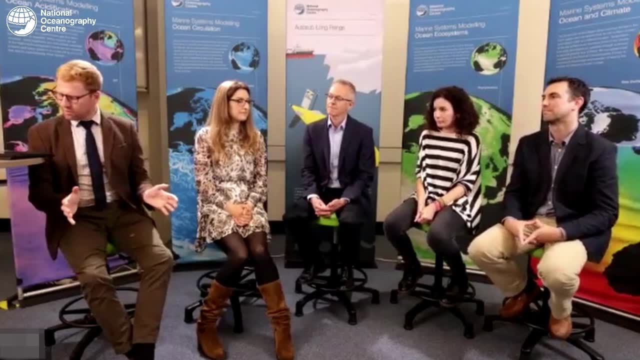 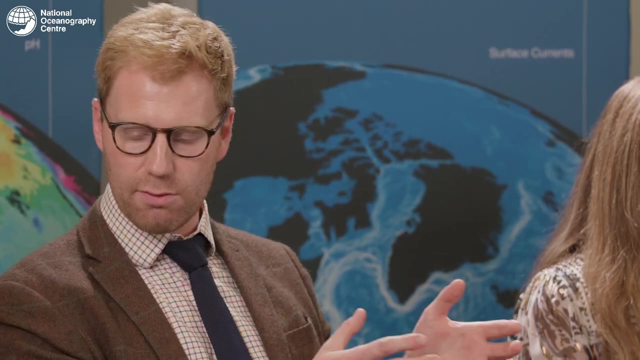 you know you've worked quite a lot with big commercial organizations in the research that you do really to provide that sort of scientific advice and guidance. do you get the sense that industry understands that we need to understand our wider ocean environment from a scientific perspective, sort of in relation to the solutions? 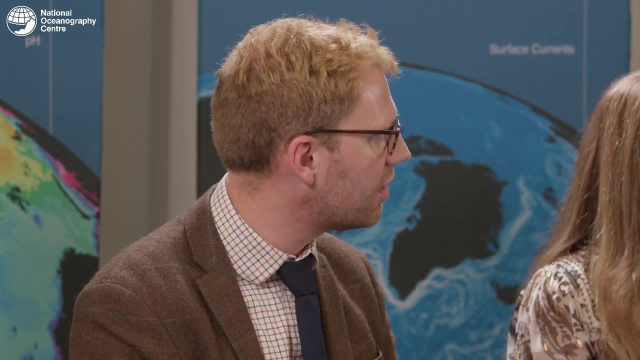 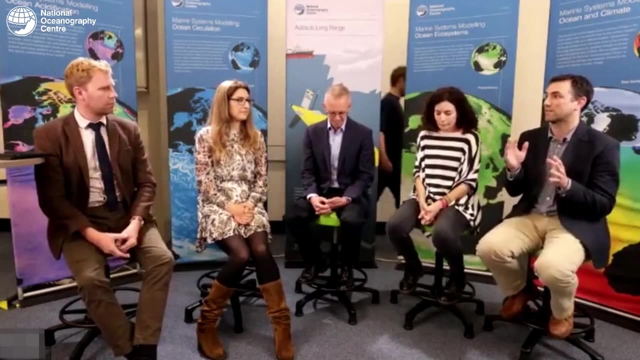 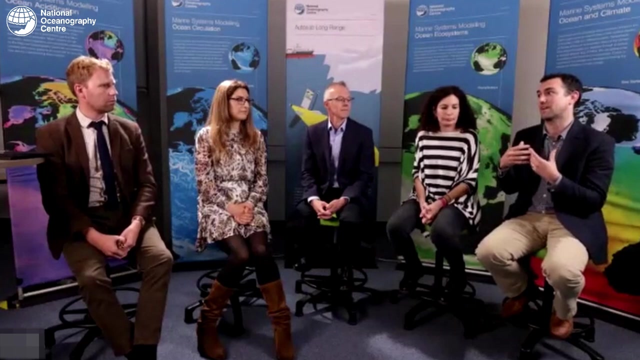 that they're developing, be it, you know, CCS or anything else. have they made that link yet? absolutely, and I have to say that everyone I've ever engaged with is absolutely starting from the fundamentals, starting that the nature-based solutions. they're closing the name, they are driven by natural processes, so understanding how those processes work, how they are varying. 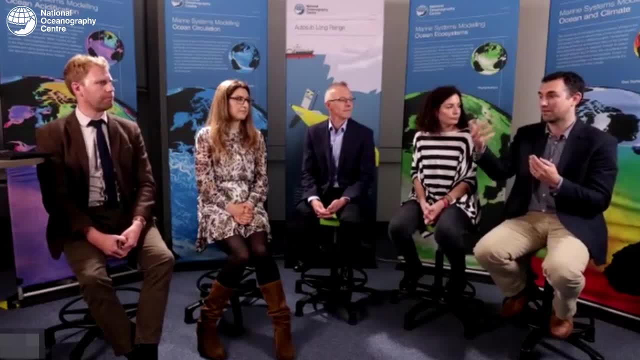 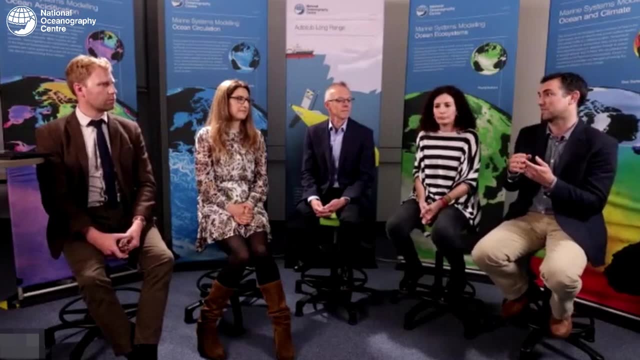 how they will be impacted by climate change. now this is an ongoing event is going to happen, so we can start to predict how those processes will naturally vary, and then how we can adjust to those processes in either a geo-engineering context or just utilize them to our advantage. 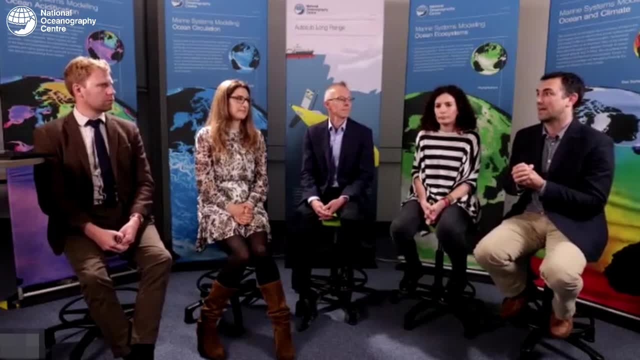 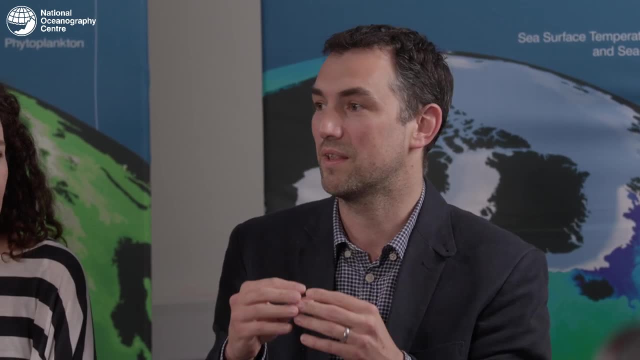 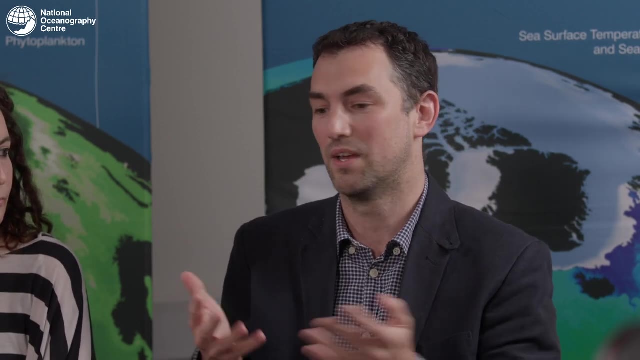 in terms of better understanding protecting areas which are naturally excellent at sequestering carbon. so a lot of companies approaches are naturally looking at this to underpin the basis of those approaches being put forward. from a more industrial approach, when you're looking at companies who are looking at re-utilizing old decommissioned oil and gas platforms, 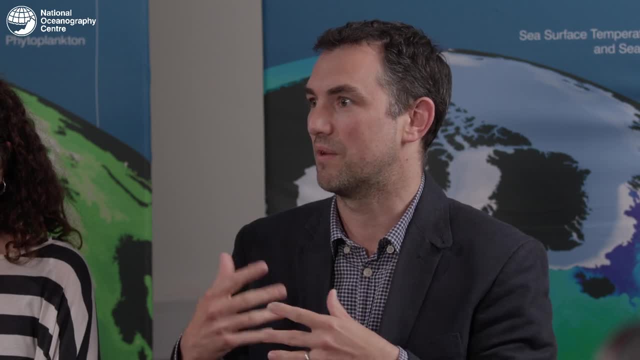 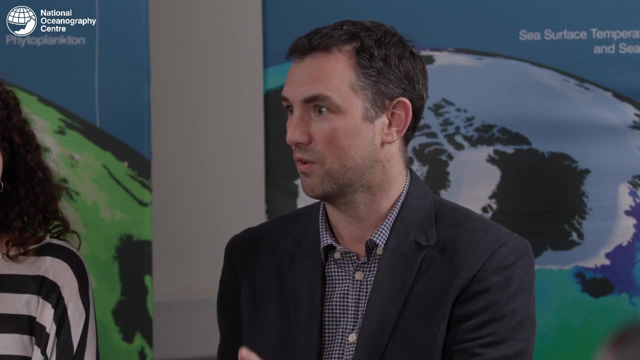 then there's a critical need to understand how any marine environments could potentially be impacted by these processes. and this is where this ocean modeling comes into context, because we can combine ocean models, which are constantly being developed and updated in terms of our computing power, but combine that with the increasing 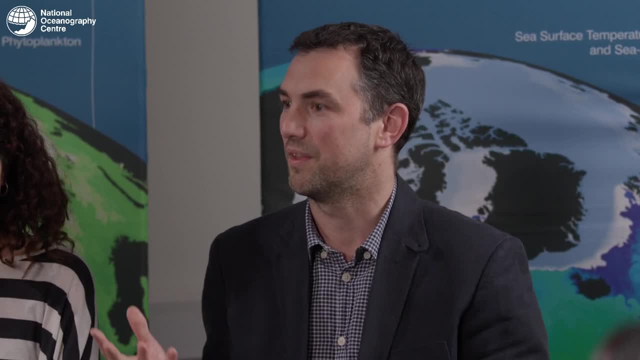 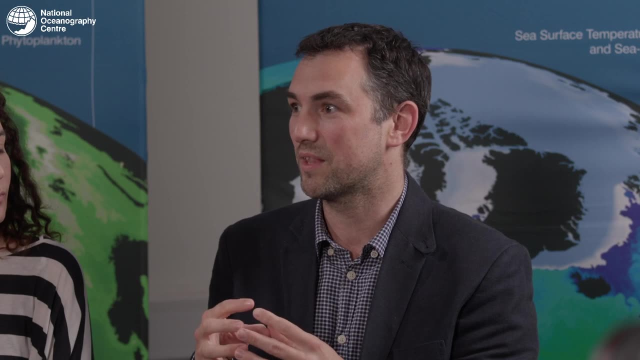 evidence that we're collecting through the deployment of our in-situ sensors and through the marine surveys that are being conducted, and we're getting more and more data all the time around the world, and combining the two enables us to better understand and predict how those environments are responding and may respond to food. 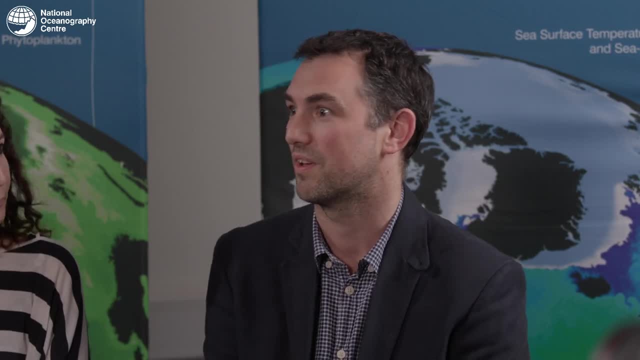 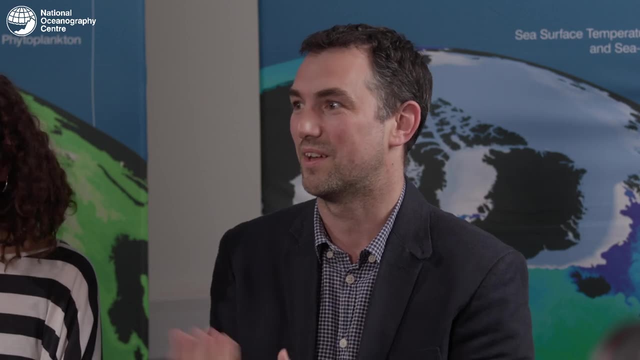 changes in climate and and as a function of those uh ccs strategies. so i think that they're absolutely working with the scientists where they have their own scientific teams. they're working with us, my colleagues, to really best understand how to protect and utilize something that's. 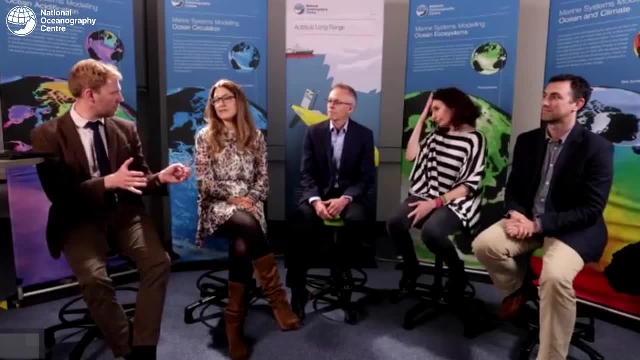 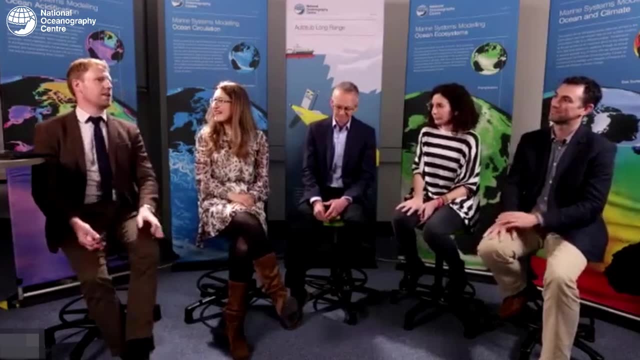 interesting. so i mean claire, anything from your experience, more, i guess, more on the kind of nature-based side that you're, you're seeing um in terms of so well, in terms of, you know, industry, you know having a desire not, not just to sort of engineer the solution necessarily, but 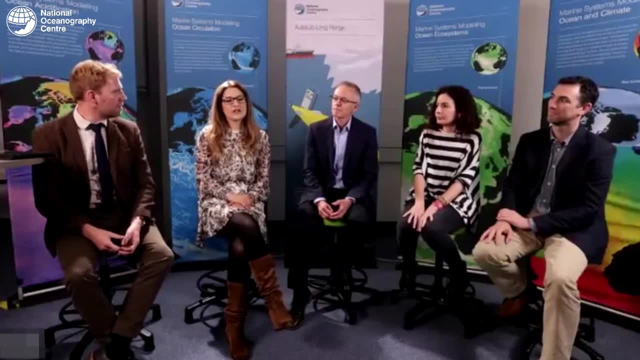 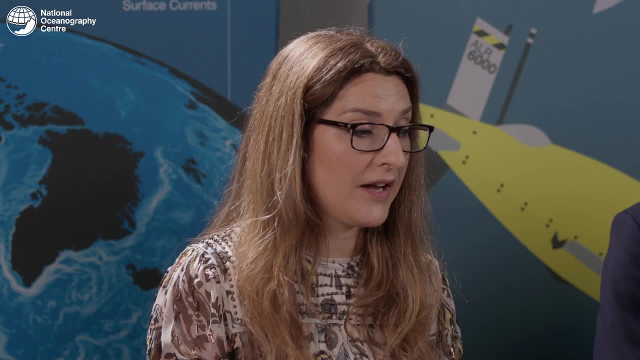 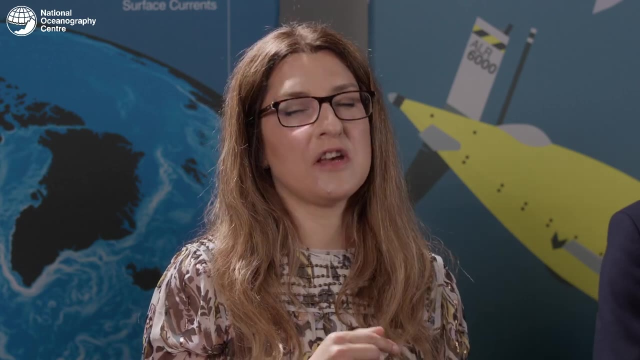 to understand the, the ocean environment, they would put that solution in sure. definitely. i think um that is coming through, um lots of companies are becoming aware of their environmental impact, and so that is um a factor in how they conduct their business and one of the very interesting phenomena. 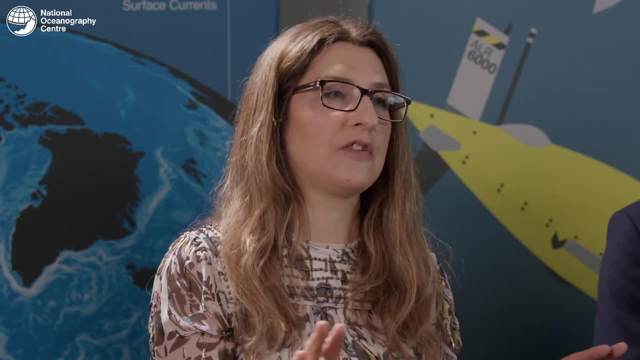 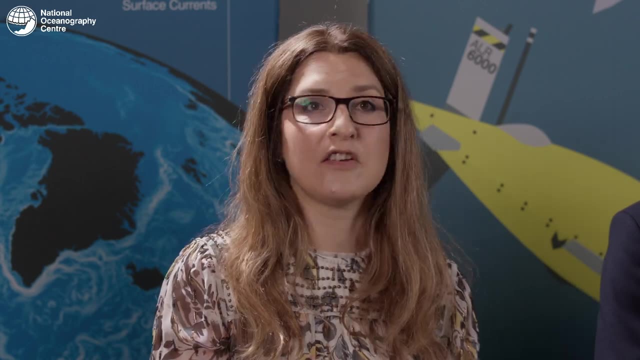 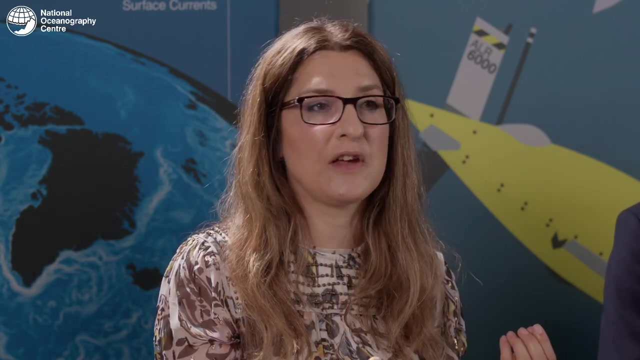 that we see in terms of um, managing the coast and these sort of charismatic environments, if you like, is that a lot of people want to invest in that, you know, and obviously there's sort of the voluntary aspect of investing in that, in terms of it's just good business to take care of the. 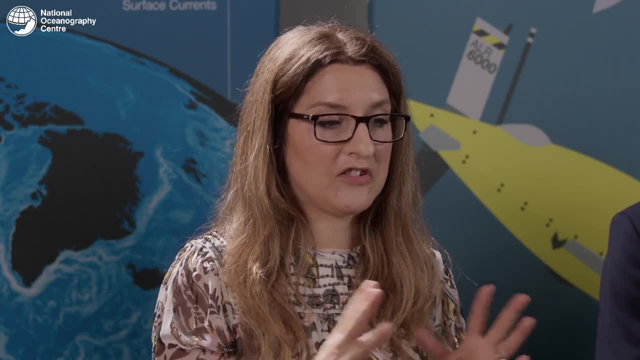 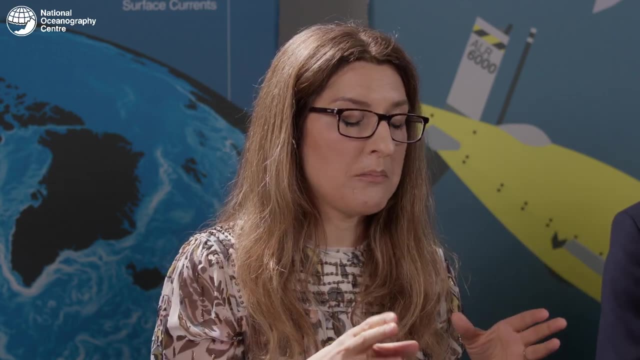 environment, but also we're moving towards uh legislation which will limit people's or companies emissions. you know the amount of uh greenhouse gases they can emit and, of course, one of the the potential ways to deal with that if in the short term they can't decarbonize fast. 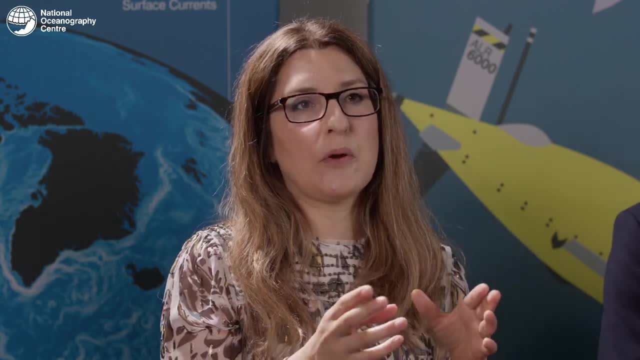 enough is to offset those emissions, and so, in terms of these kind of nature-based solutions, there's a big interest in the environmental impact that we're seeing in terms of the environmental impact that we're seeing in terms of the environmental impact that we're seeing in. 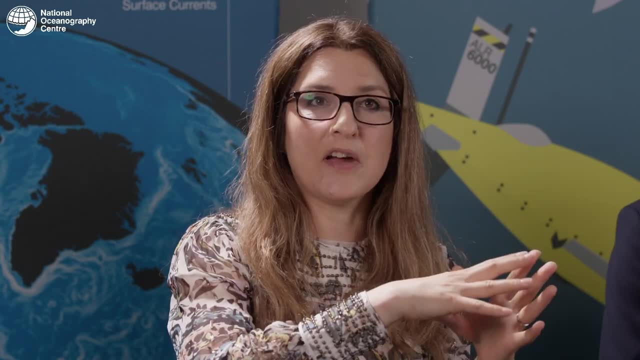 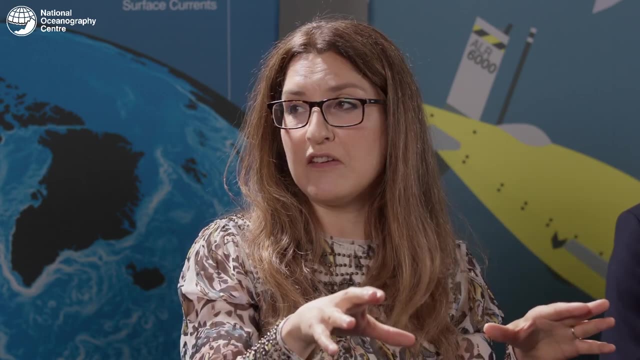 in in the the potential to using those carbon credits whereby you you purchase some kind of scheme or you buy in some kind of scheme that actually manages the marine environment in some way and reduces, uh, those missions and thereby offsets the emissions of the company. so i think 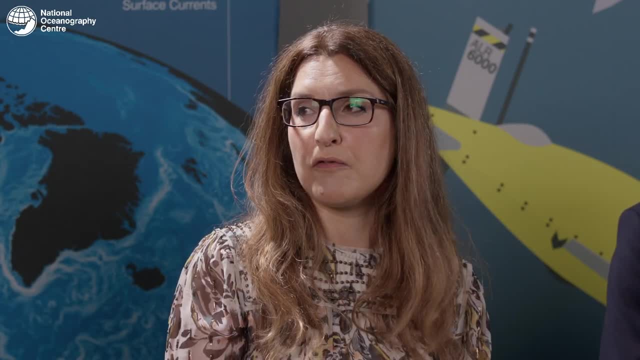 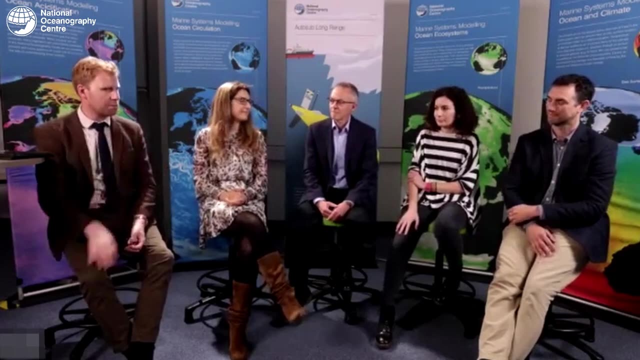 that is something that's very prevalent in the minds of lots of commercial enterprises at the moment. um, i'm going to go right back to basics here. doug, i'm going to throw this one at you. um, we talked loads about solutions, solutions, different aspects of industries, perception and involvement. 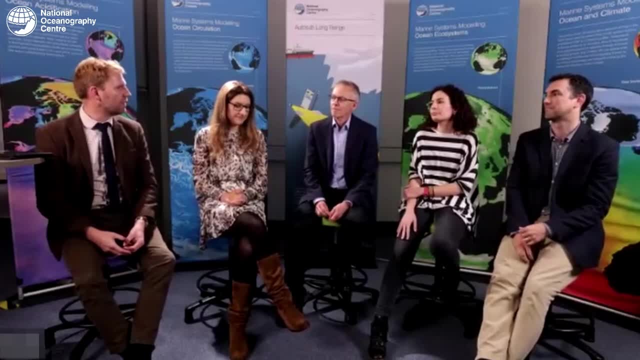 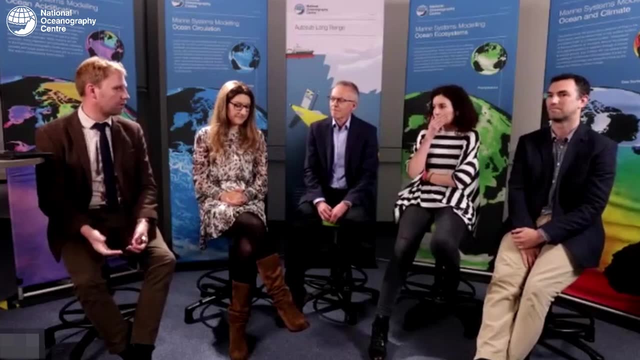 a basic question: what, why is the ocean so important in, in climate change? you know, thinking over the next 30, 40 years, what is it that is so special about? about the ocean that will will ultimately be at the core of, you know, the solutions that we develop? uh, as chris alluded, 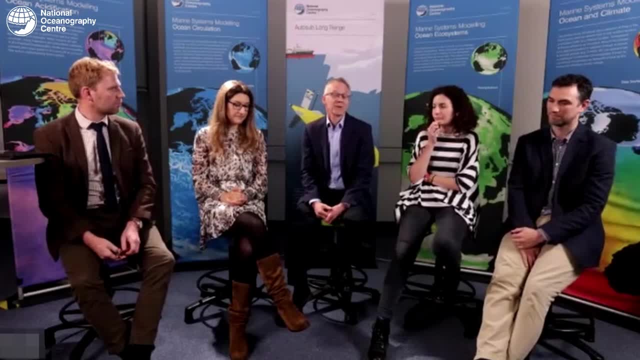 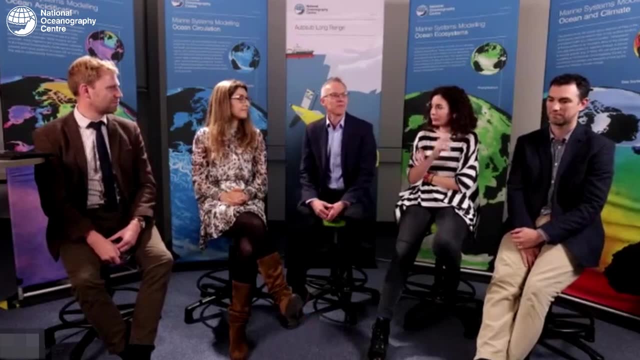 to earlier on. at the moment, the oceans are still absorbing most of its pollution, that's, the carbon dioxide pollutants and everything other pollutants. see, you know, the deep sea sediment sources refer to was the ultimate sink. you know, nearly everything we produce ends up in the deep sea. so you saw that. 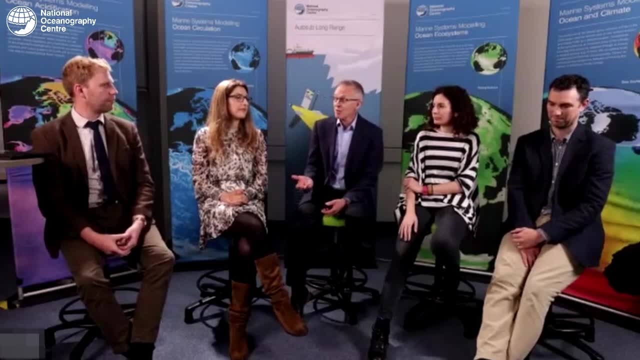 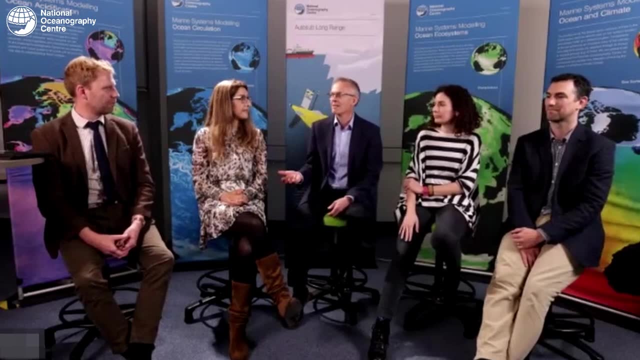 in the. you know the very large press concerns around plastics into the oceans, etc. whereas the solutions plastics in the ocean, probably isn't in the ocean. it's actually stopping the plastics in the first place, in the same way that the climate is stopping the co2 emissions in the first place. 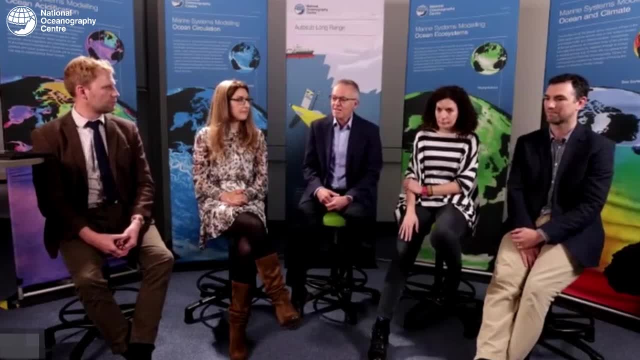 that are going to help the climate. but the oceans- you're seeing a recognition with sort of cop- last year's cop in glasgow you saw the recognition of the oceans have been one of the most important components of the environmental system in terms of our management of climate change. 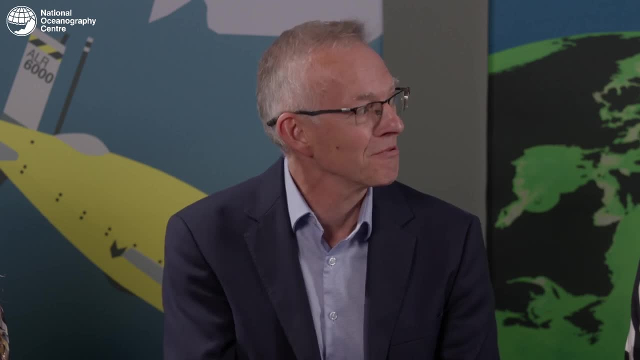 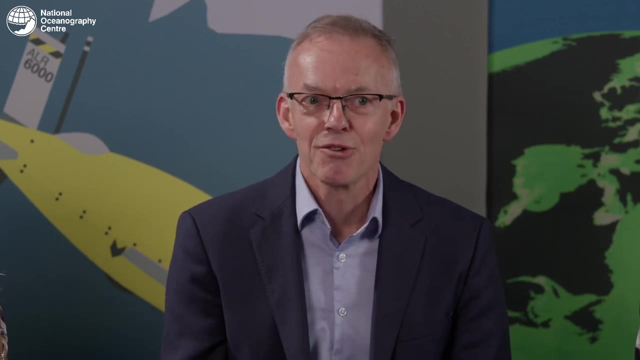 and our understanding of the way climate change. i think that's your commercial comment earlier on. we get good engagement now from commercial organizations because they're recognizing the leverage. by talking to one group of scientists, you're actually bringing a global scientific knowledge because scientists work together, particularly in ocean science. it's 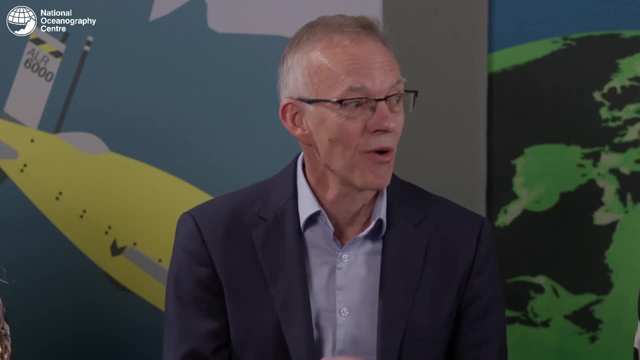 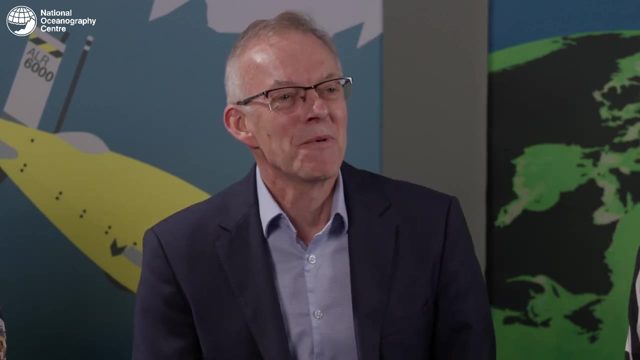 big, it's broad scale, it's wide ranging. we can't do it alone. no one nation, never mind no one institute. you know we do a good job, give a good crack at knock in trying to do most of the planet um, but we do all work internationally. it's big, it's expensive- science to look at the oceans and 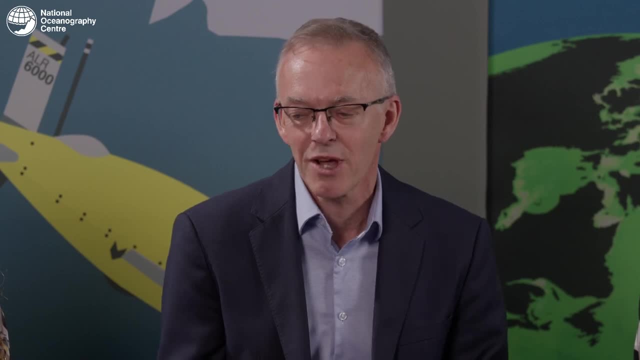 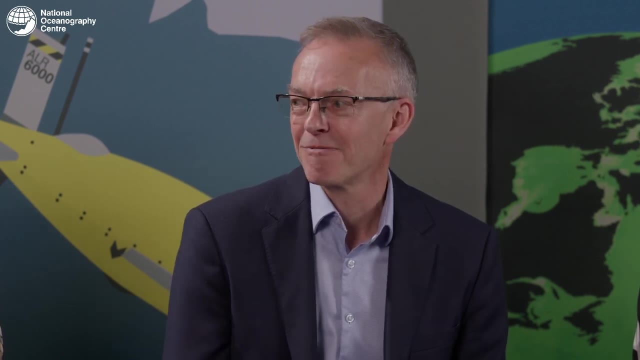 so by working you know that that nexus, you're seeing a much, much better work between commercial and scientists- is that they're getting the whole world of scientists actually involved really, so a phenomenal amount of you know that we're not in competition, really, scientists, uh so they're. 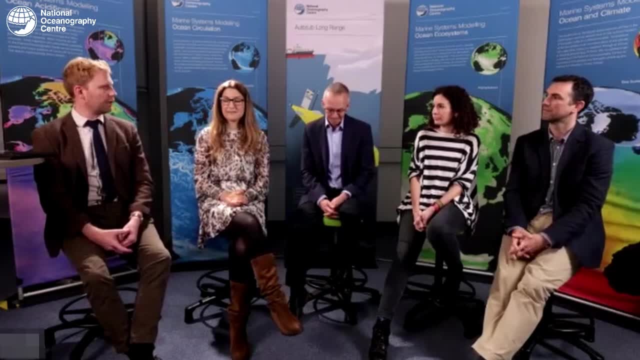 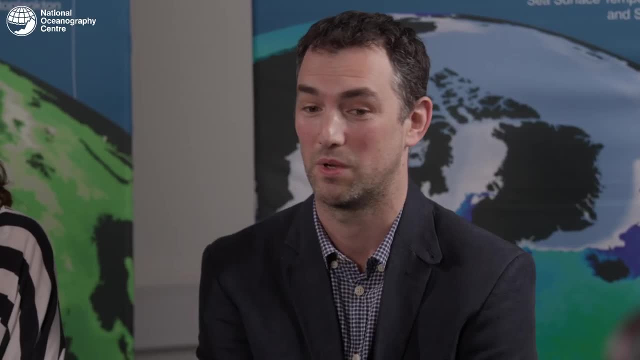 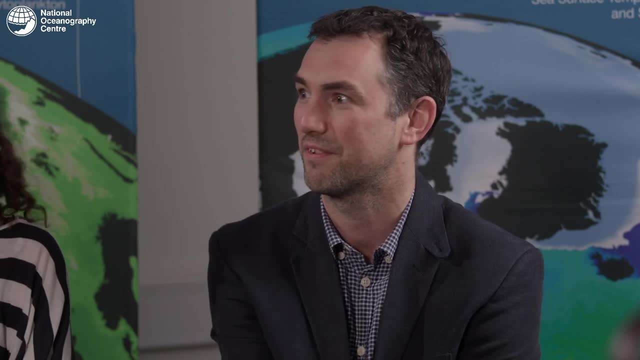 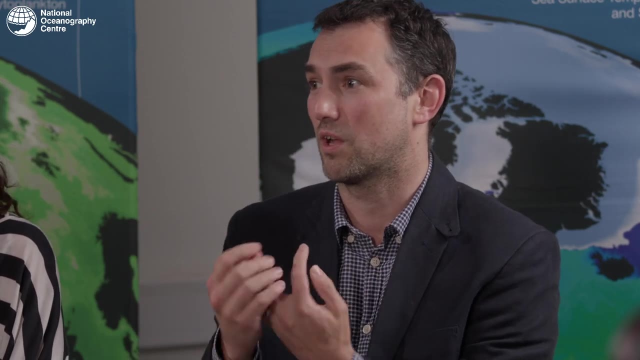 we are living in the blue planet. the asians cover 70 of our surface, so i think you know, we need to recognize that they have. they're not just the impacts, they're not, you know, asian acidification, sea level rise. you know global warming, sea warming, uh, deoxygenation. there's lots of things to be. 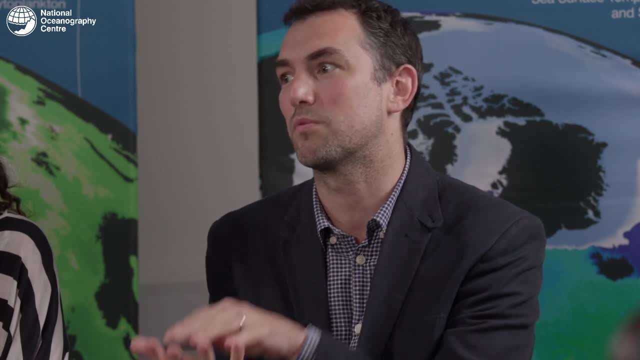 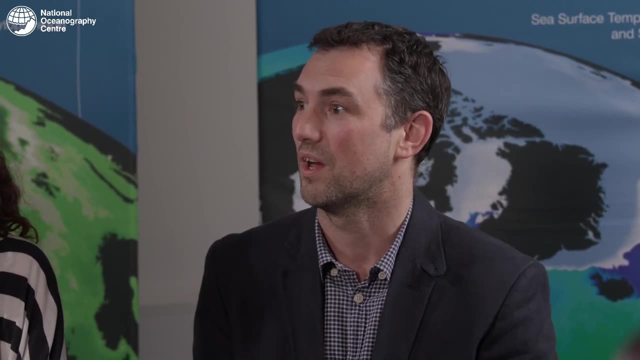 concerned about the impacts of future climate change in the oceans, but they can also be part of the solution to it, and i think understanding where, when and how we can best optimize the stations is what we're trying to work and support um companies in terms of achieving that, but you 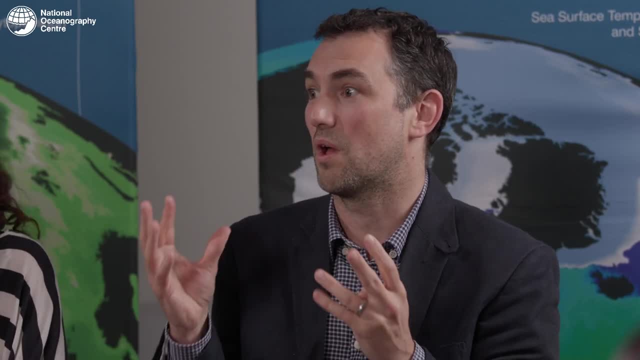 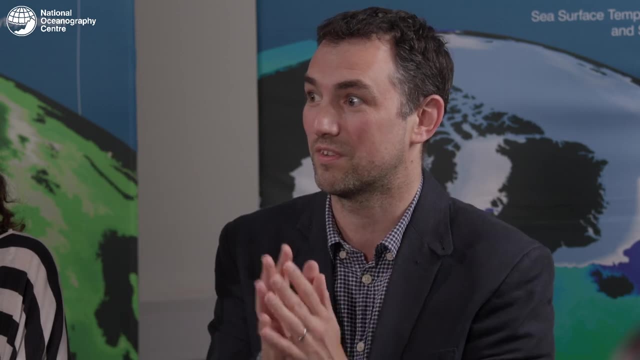 know the. the oceans have a lot of potential and i think that's what we're trying to work and support. oceans have that scalability potential. you know, um, we have to recognize it's related to that. it's an international problem. you know every country, you have their international waters, um, but you 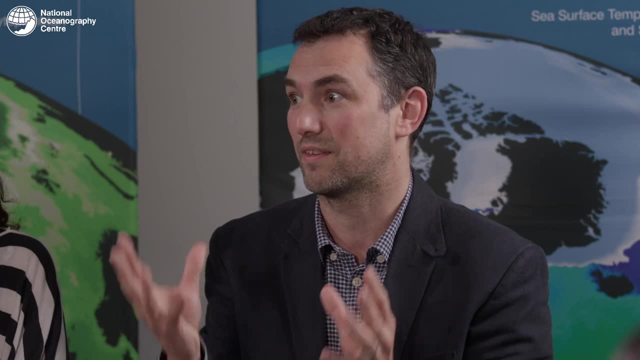 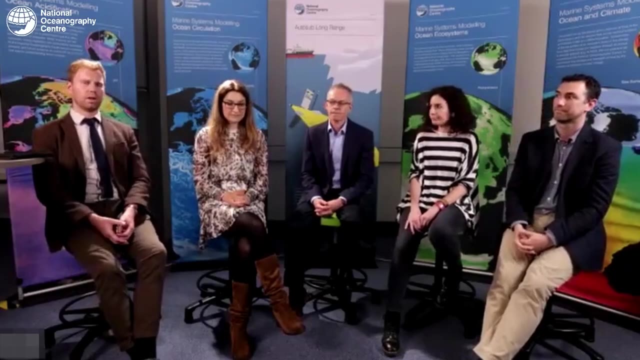 know, in international space, you know we need to work together collectively, both as a scientific community as commercial companies, to ensure that this is done in the right way. okay, that's great. i i suspect this is a topic that people want to get involved in, so i'm going to just hand over now to 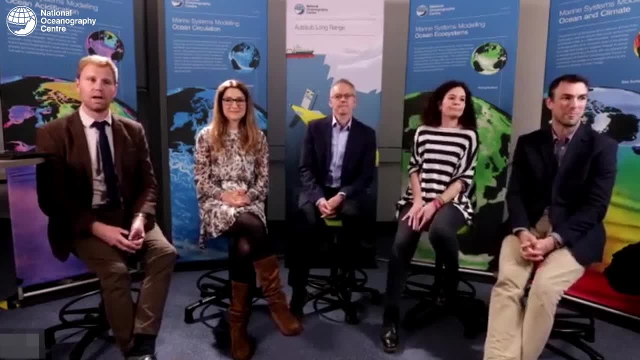 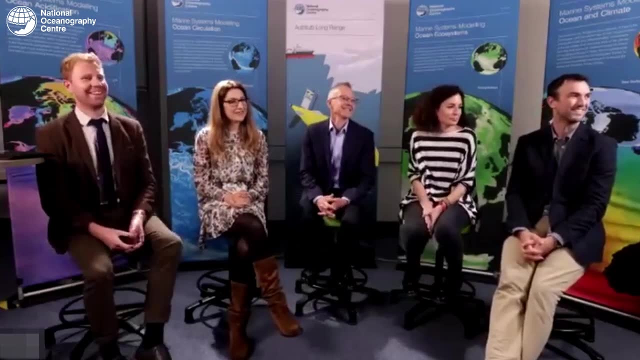 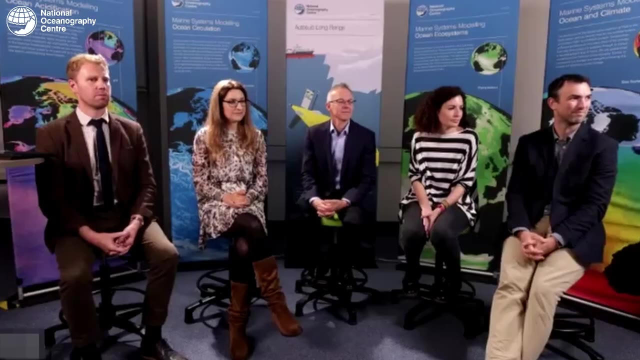 um audience and uh questions and online as well. um, so i'm looking to the audience and hoping for no silence when i do excellent. we've got a hand brilliant. um, so, as scientists, you know what has to be done. um, and the problems faced by climate change and why the oceans are important, but often 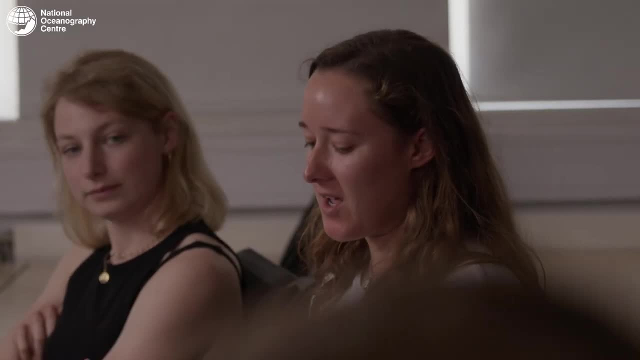 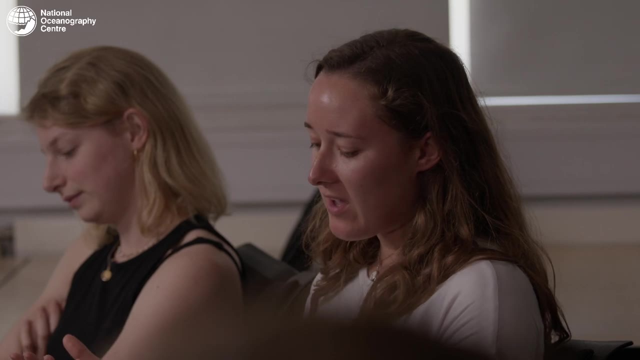 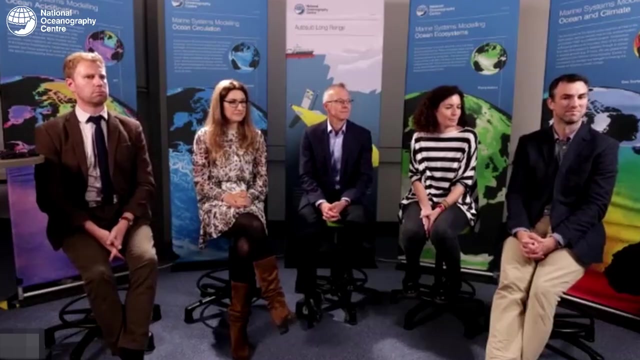 the decisions are made by policy makers and the public that vote in companies, policy makers, but they may get a lot of touch with the ocean. so, taking all that into account, um, how can ocean health, climate change solutions and what can scientists do to adjust? so i can start that one. 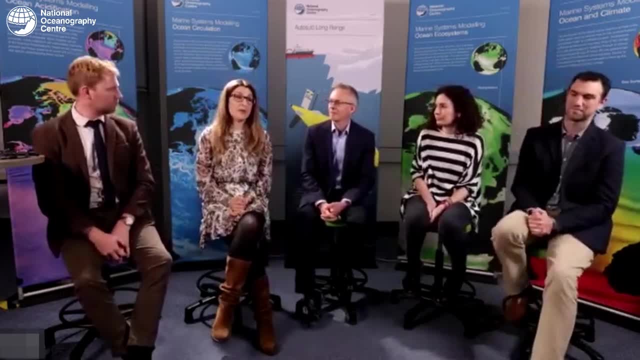 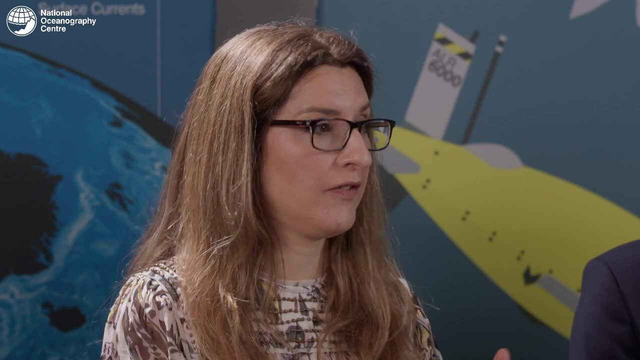 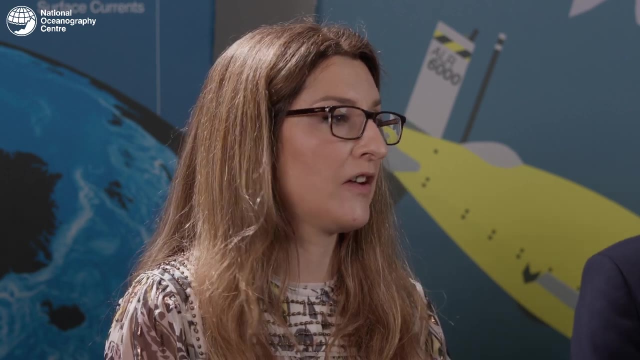 if you like so. so i think, um, your question is an excellent one and it's really, really important and, as the panel have alluded to, no one sector can solve this problem. it has to be everybody's on board or it's not going to work, and so one of the big projects that i'm running, um is looking at. 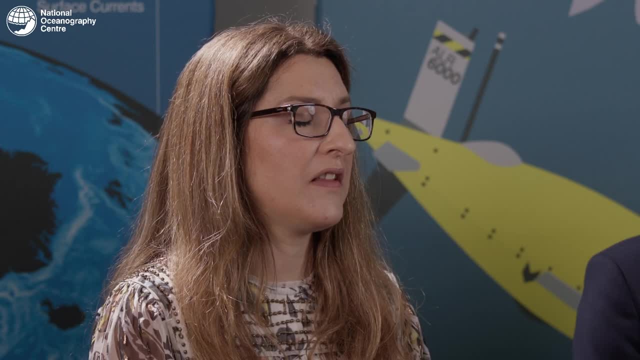 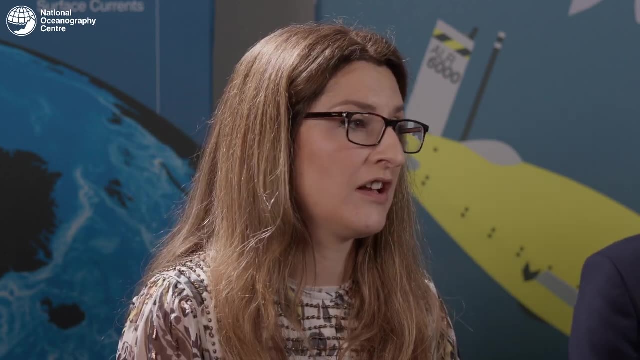 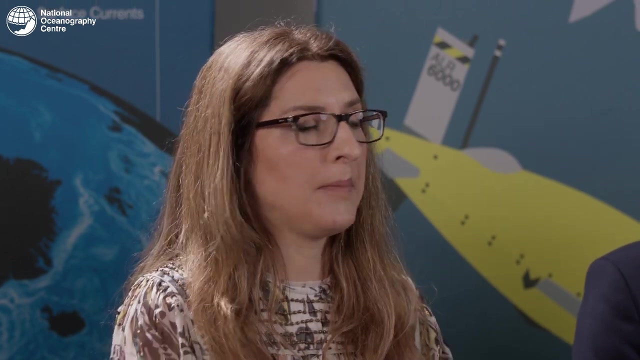 seagrasses around the uk and actually what we're trying to do in that is understand the social and political barriers to restoration and preservation efforts and um, you'll find there's a lot of. so you spoke about ocean literacy and a lot of the problem is people just don't know. 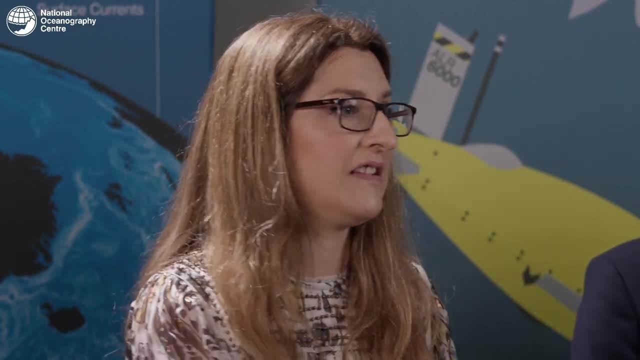 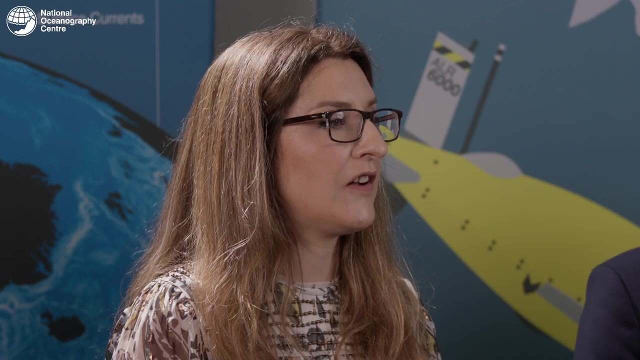 what's beneath the waves you can't see. you know you can't see seagrass most of the time, so why would you know about it? you know. so there's that piece about what's our responsibility, scientists. well, we have to make sure we communicate what we're doing, so events such as these, you know, are. 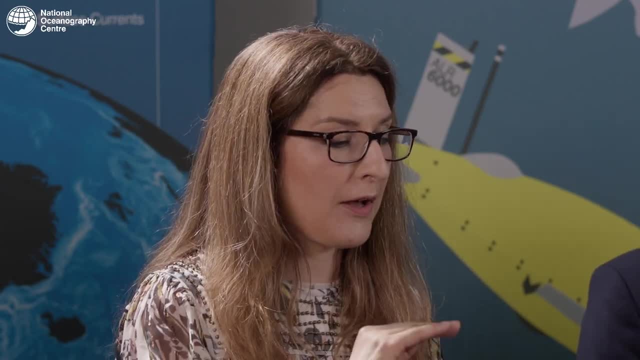 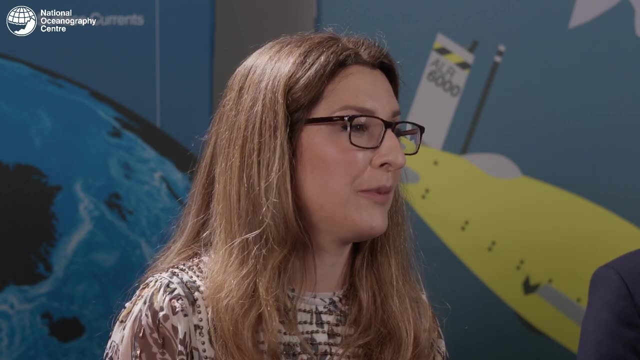 the biggest thing in the world and i'm a big sickid for that um but um once uh, people have that information. we can make more informed decisions when, when someone's going going to the polling booth, you know if they're aware of what's going on and what what potentially their oceans can do. 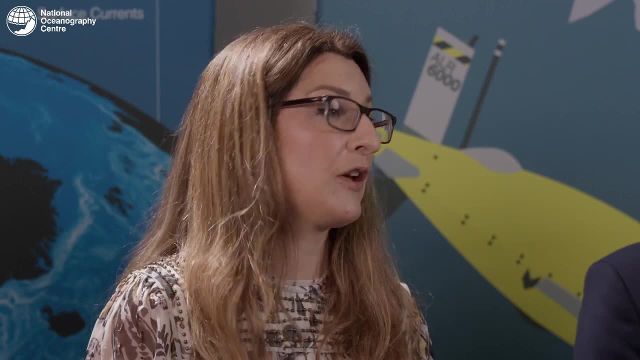 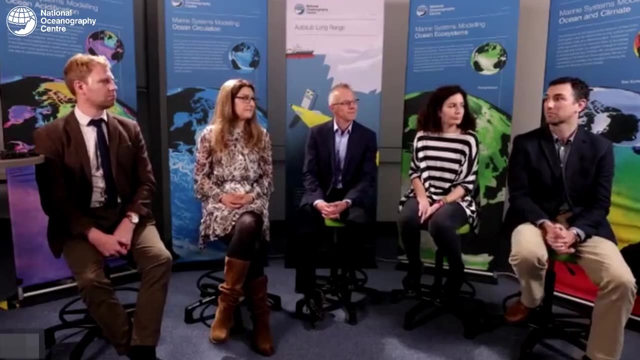 for them, then hopefully they'll vote for the, the people who are um planning the most responsible uh legislation to safeguard our future. yeah, just to add on that, a lot of work has been done to actually make sure um is going to be a living space for people who are going to be. that, i think. so, yeah, that's, that's what we're working on. for the most part, um, and i just want to make sure we have the support of the health care approach because, um, i'm sure we have the support of health care professionals who are working on that, but we're gonna make sure we have a more local health care system and we'll also have the support of health care professionals who are working on the health care pelo, and 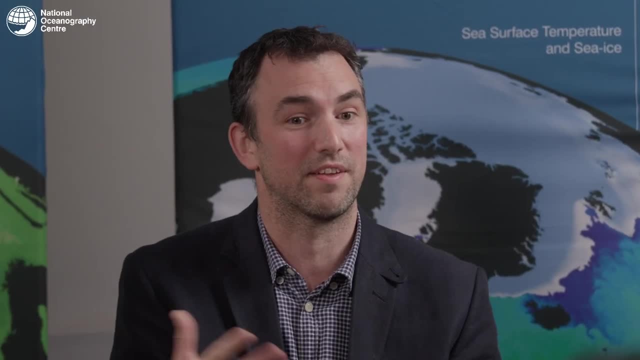 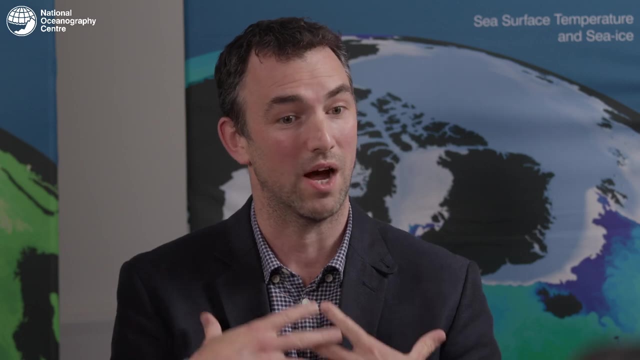 understand how best to engage, uh, and facilitate these types of solutions that we've been talking to, because it is a highly emotive topic for everyone. understandably, i think, a lot of people feel either direct or associated connection to the oceans. it's something we naturally want to. 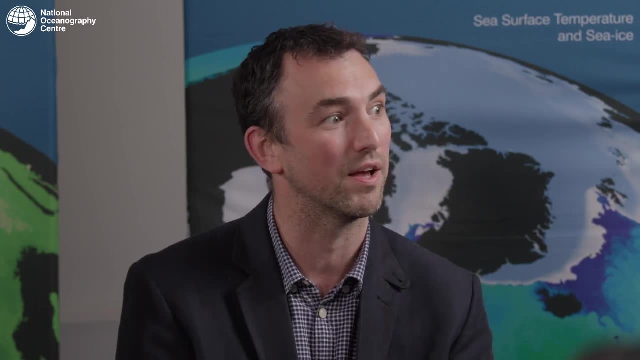 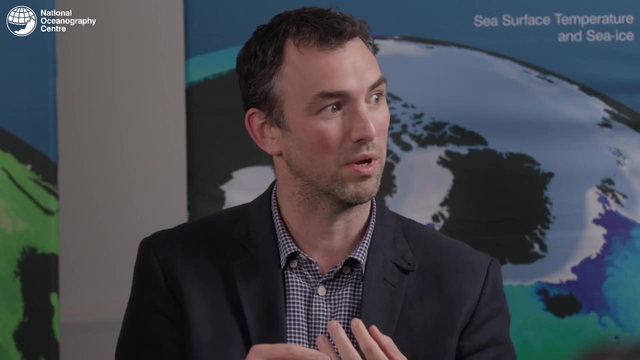 protect because of, uh, you know, many people's existence and sustenance relies on the oceans. however, as alluded to, you know, there's this recognition that you know they're going to be impacted by climate change anyway and so we know we, if we don't do anything, then they're going to. 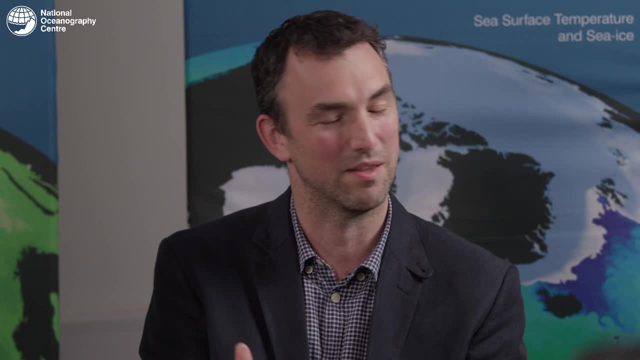 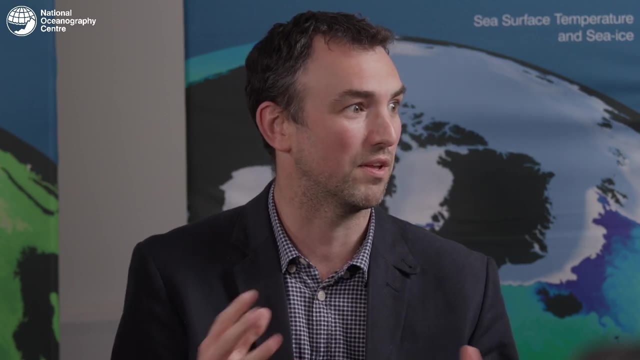 be changing. if we do see something, then how can we best achieve that in the best practical and effective and safe way? so, um, there's lots of consultations ongoing. this is you know. there's a number of projects actually starting to reach out to people to see where you know, what are you. 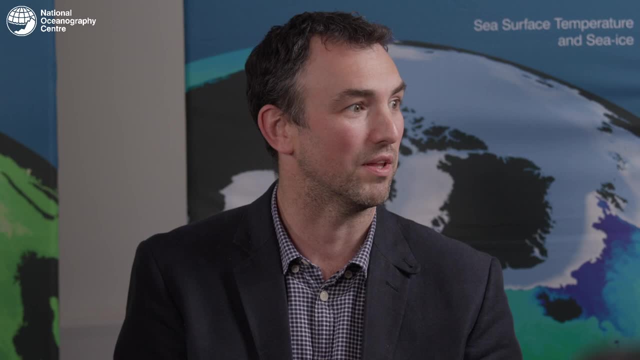 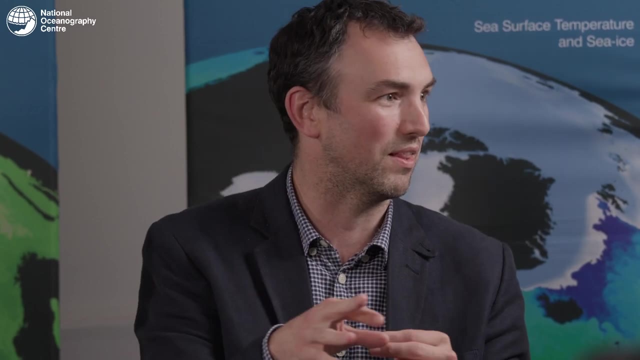 comfortable with what can be done and, equally, coming up with the scientific knowledge of you know. what are those impacts? you know or you know? are they actually significant? we have a fear that, oh, you do anything. the ocean said it's going to perturb it. well, this perturbation is happening. 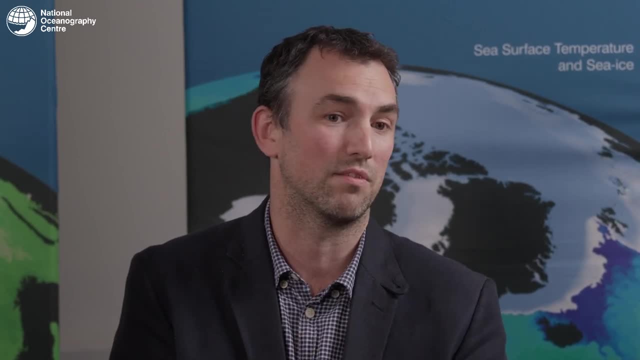 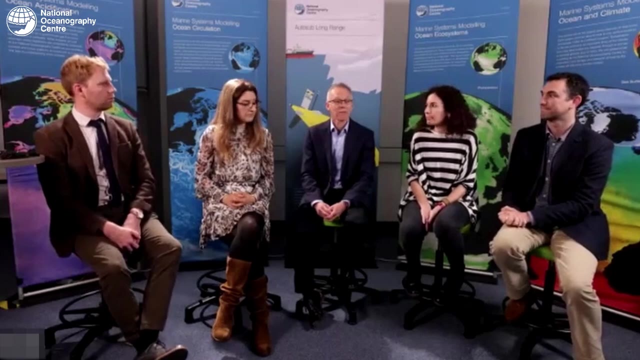 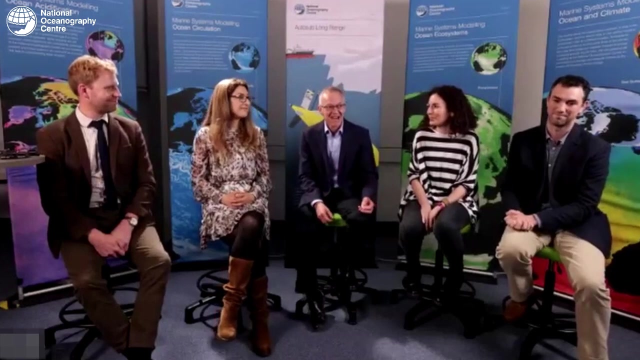 anyway. so you know, can we actually offset some of that in an effective way and actually support the ecosystems in a way that's going to be beneficial for the long term? i have one more thing on the ocean literacy. one of the key things is actually translating science into a language that can be understood. i mean, i think before the blue planet, i mean we've 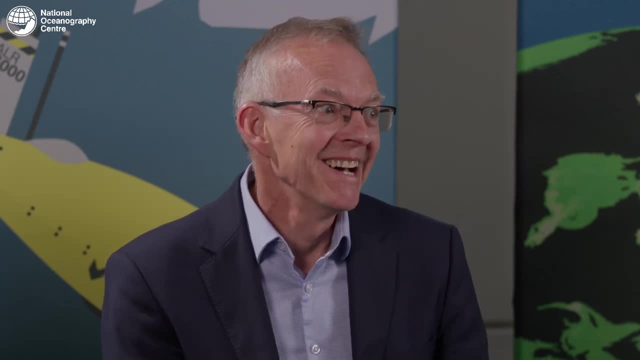 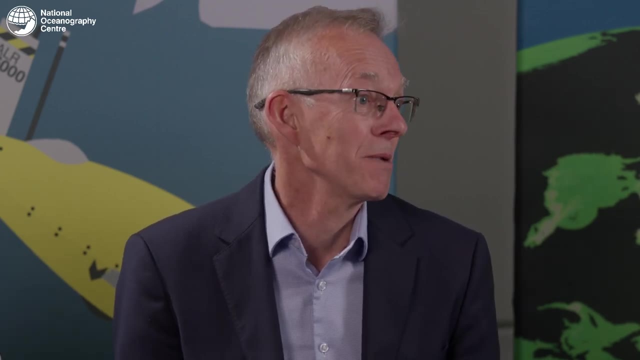 got to acknowledge the blue planet. it's probably what brought the oceans to cop. um, you know we were pretty- we have been in the past- scientific scientists pretty poor at communicating with the general public. um, and it's now we're at that. you know the general public is suffering from things that are happening. 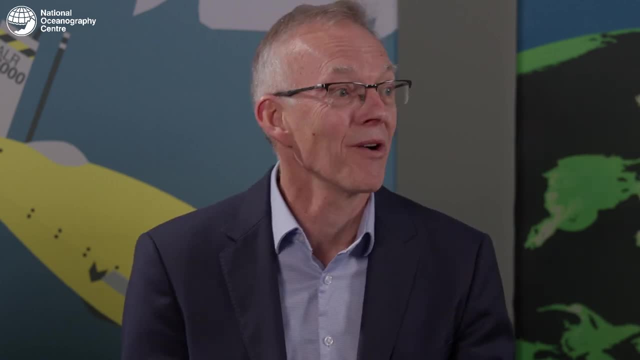 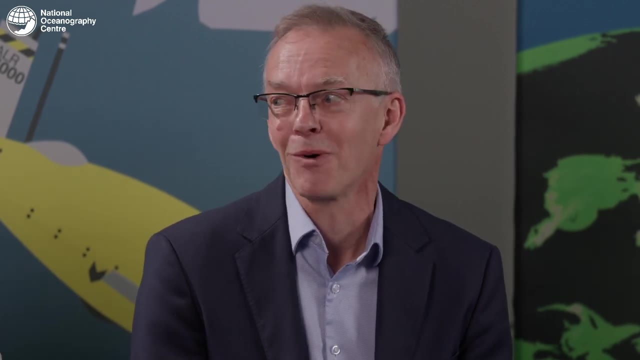 in the environment we've got, we know how, why, what is going to happen, what might happen in the future, based on models, etc. communicating that in a way that the public understand, then guides policy and because you know you're going to vote for someone that wants to do some good. 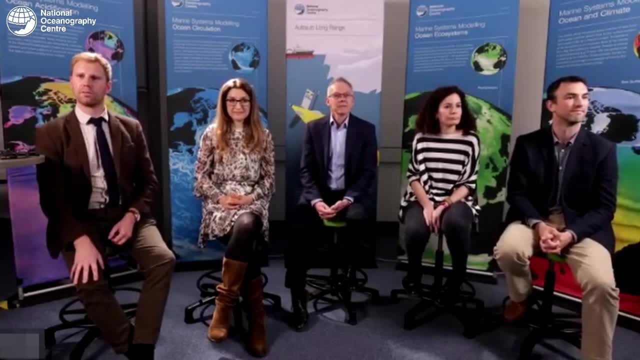 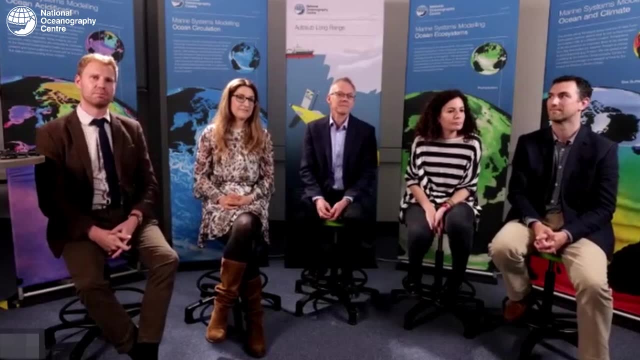 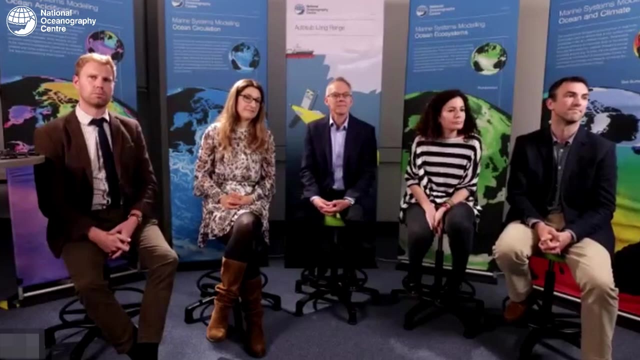 brilliant thanks, thanks i. um. we got any more questions from me? yeah, we've got on here. yeah, excellent. um, we've got a question about success stories and symptoms um mitigating, uh, life that's impact. but how? how frequent are these success stories, or is it quite a duplicated? 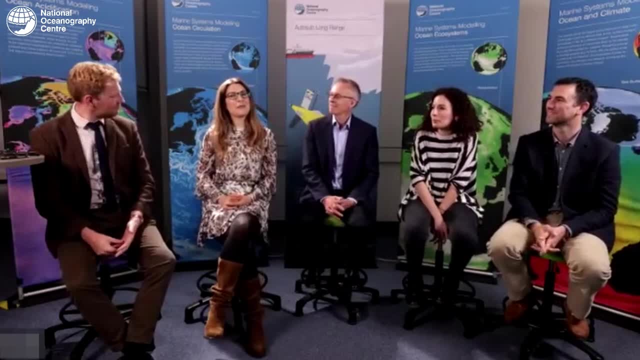 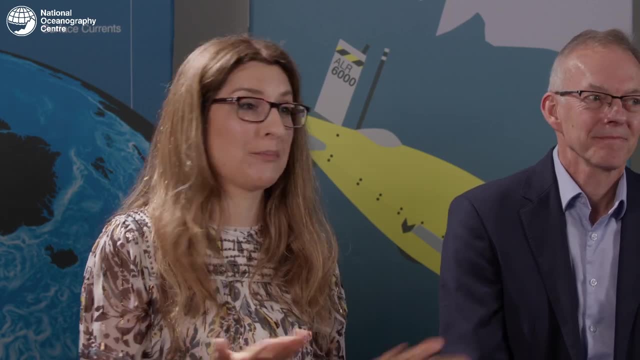 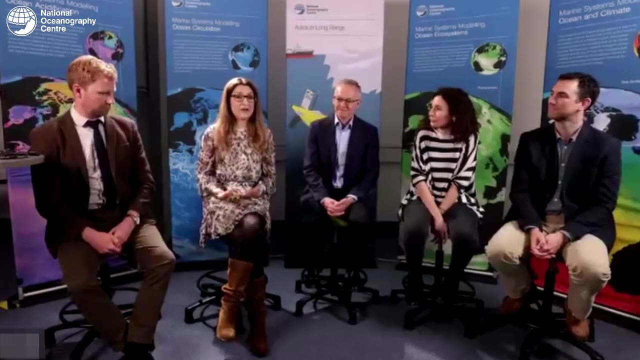 uh well, i think at the moment, um, once you have a look at the, the evidence it's, it would be quite easy to become quite afraid, actually to put it bluntly. i mean, i will not say what's going on, but i will say we're in a situation where we can. 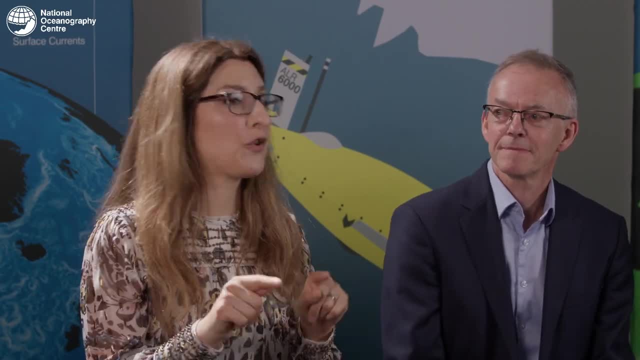 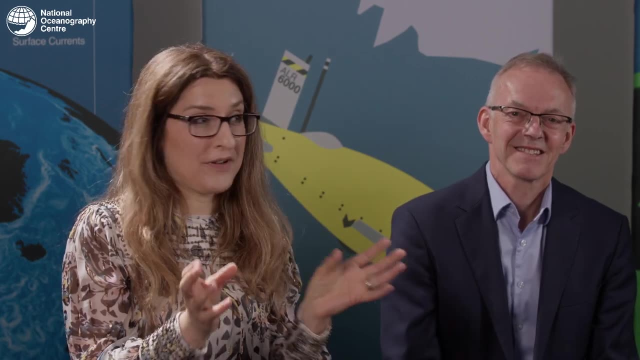 we can be a bit more optimistic, or a little bit more optimistic in terms of what we do responsibly, or maybe a little bit more and, um, you know, i don't know how many people are in the world that are in that situation, and i think people are probably going to be in that. 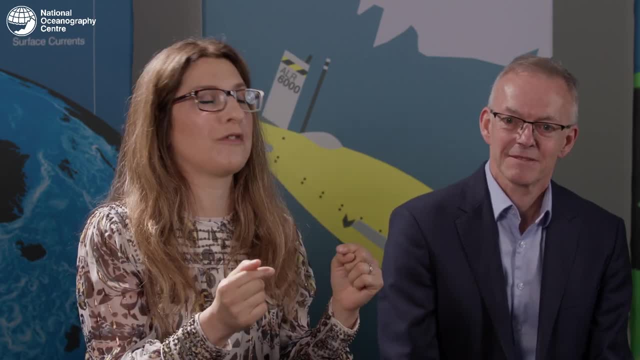 situation when they see the, the, the, uh, the, the media, they're not going to be as sociable or as kind of- as you know how to put it. um, and- and i'm not going to say that it's not the way it is, but i think it's been a great deal of improvement for people to have, um, you know, an active and you know. 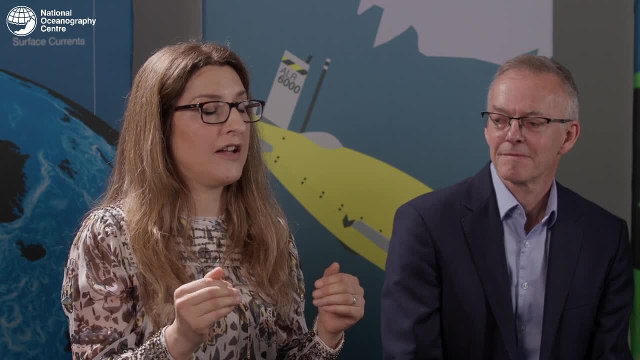 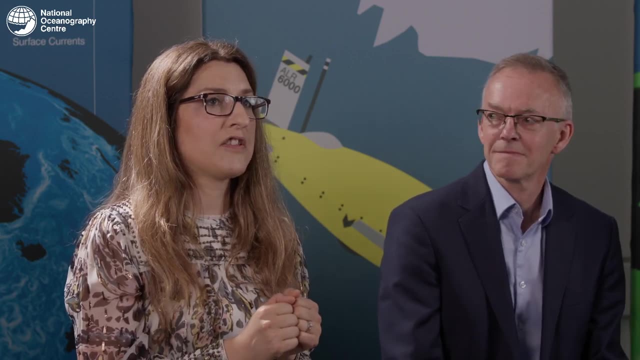 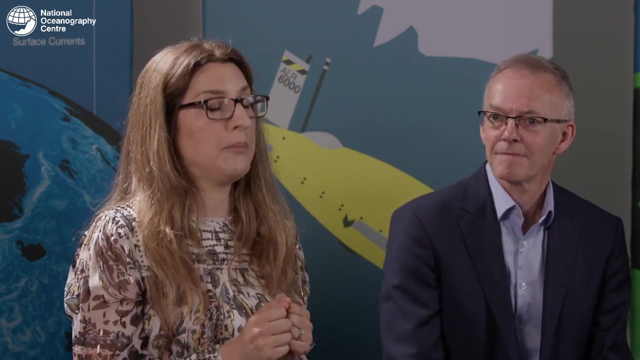 now an acceptance that, yes, this is happening and we need to do something about it. so you, you know, you're interested in specific examples and I think at the moment it is in its infancy. so when we think about the kind of biological solutions we might implement, there are certainly coastal vegetative. 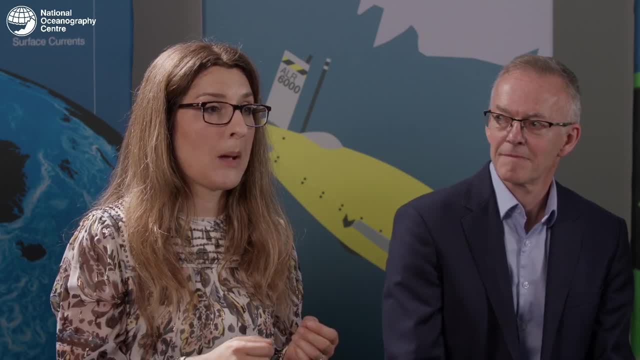 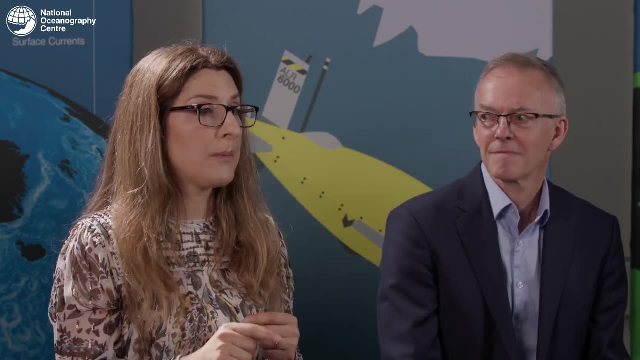 systems that have been restored around the world. but that needs to speed up and, more than that, we need to stop destroying them in the first place. and we're destroying them in pretty basic ways. you know. we're still discharging sewerage into the solar now and then. this is terrible, you know. 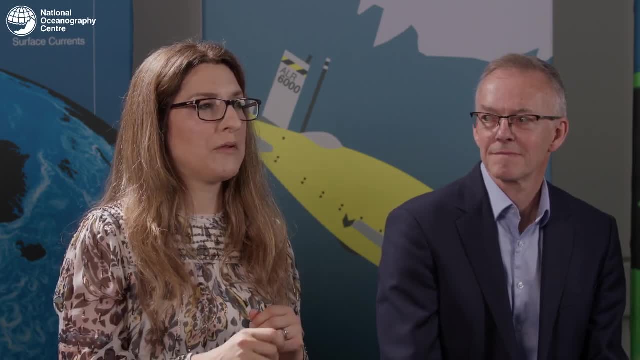 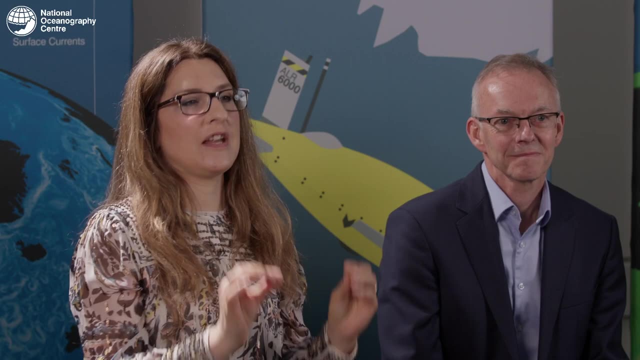 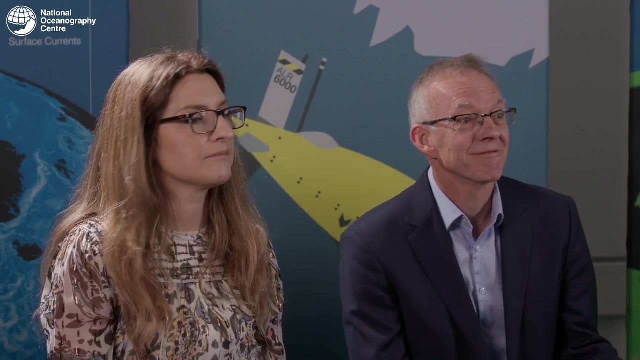 this is really not good for marine habitats. so so, yeah, but I feel, I feel like we can pull together, we can do this. so we're, we're in the infancy, but it's, it's starting to build momentum. I really think, and we have done this: the Montreal convention, removing freons, and you know. 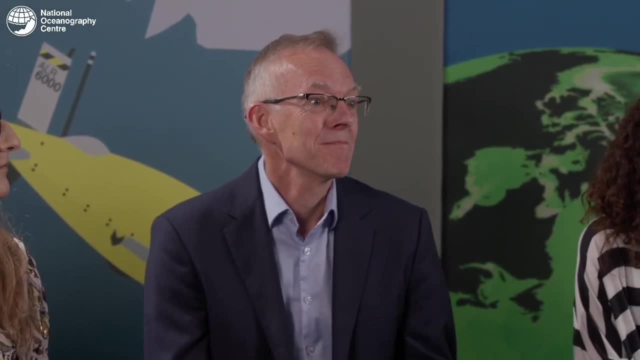 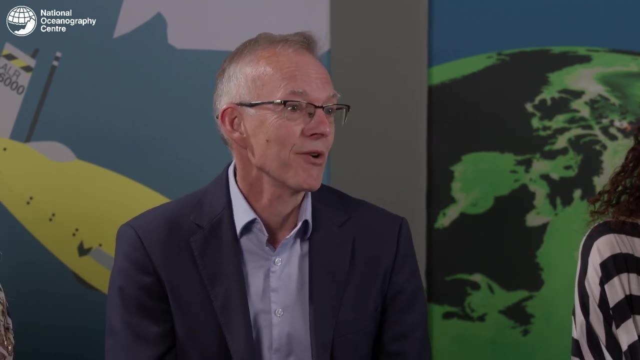 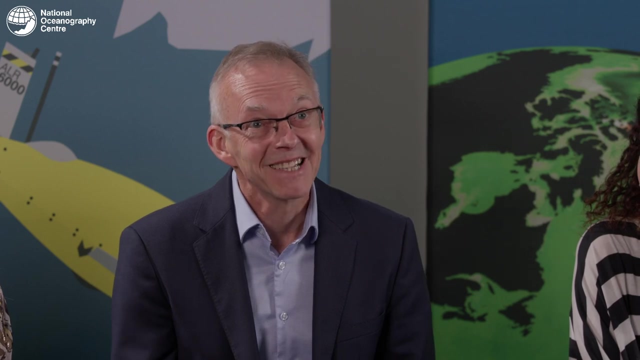 depreciation you the reduction in sulfur dioxide emissions which stopped acid rain and stopped just destroying the black forest. we can do this, we can work together and we've got these training examples of actually how we've come together in the past at a global level to make these changes. it's that sort of 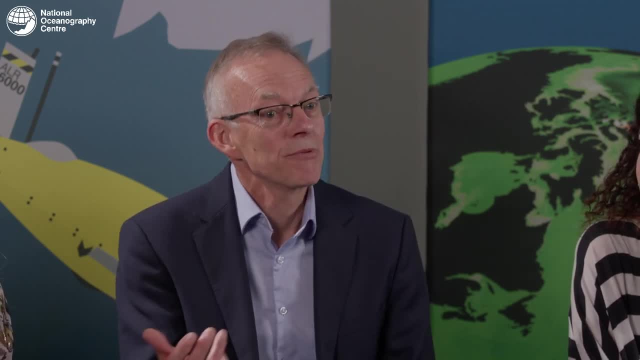 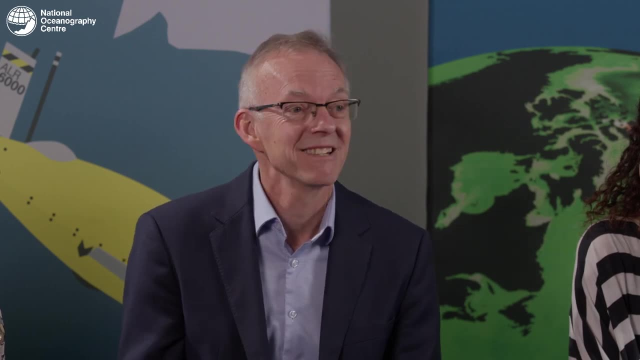 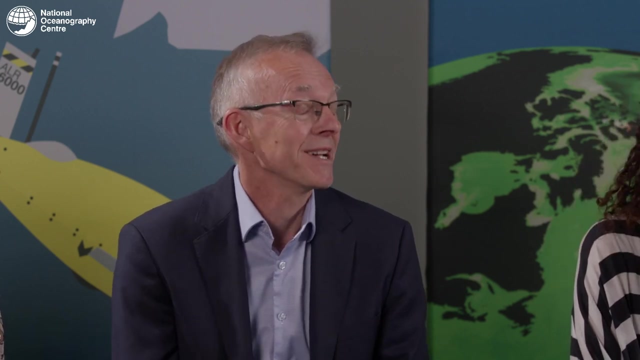 balance of paying now for benefit later. I mean, we did away with freons over what five, six years rich body knows. over five, six years we literally did away with the whole freon industry in refrigeration and changed how we do things to stop the ozone depletion depletion. so, yeah, we can do it. so I'm reasonably optimistic and yeah, technology will save. 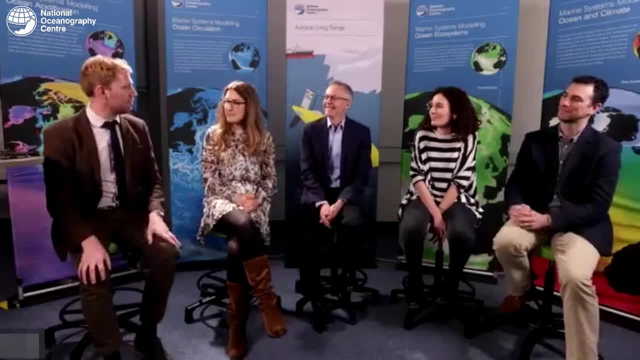 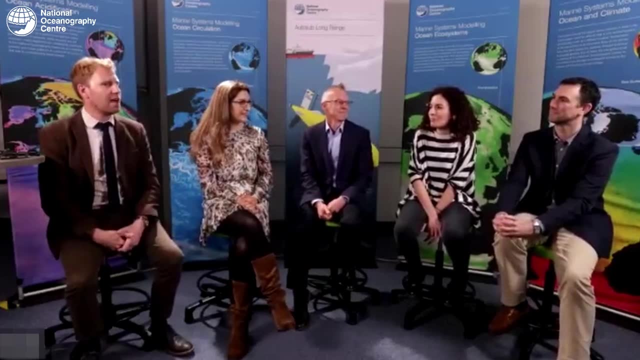 us. I don't want to burst the high energy and the motivation around this because I'm I'm infused mкая. there is someone who's got the end position, this foresight from a modeling perspective. how do you? you know what's your research and what's your science telling you in this, in this space? 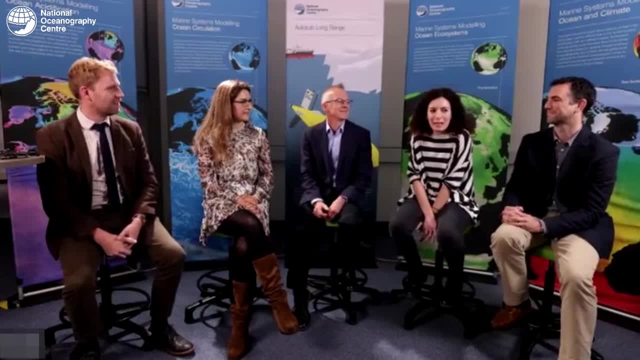 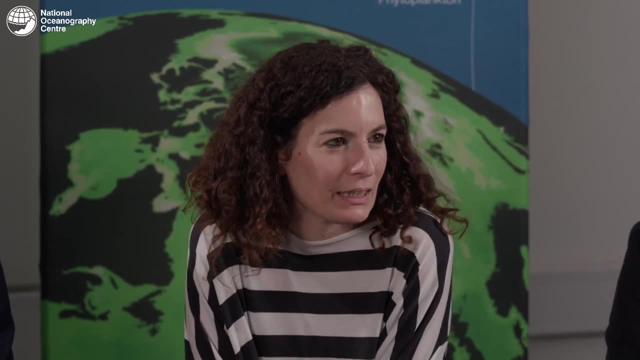 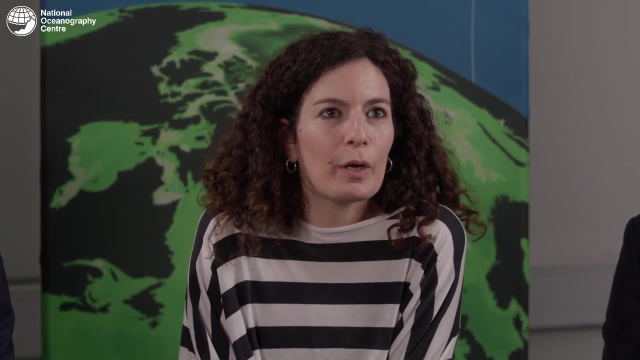 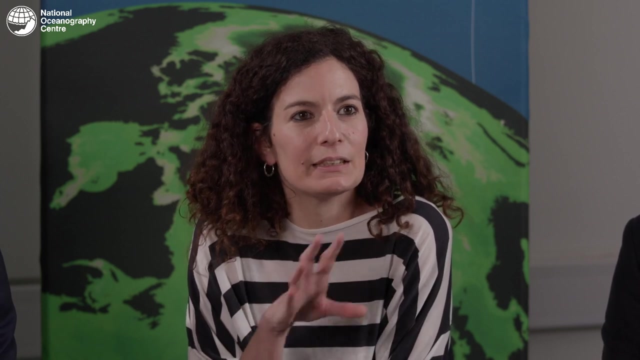 I'm pretty optimistic too, actually, because I think that's the. the technology is there and it's just a matter of implementing at a real scale. and so when i was talking before about the possible negative aspects and the fact that we need to know them in advance, it doesn't mean that then we we are not going to put the 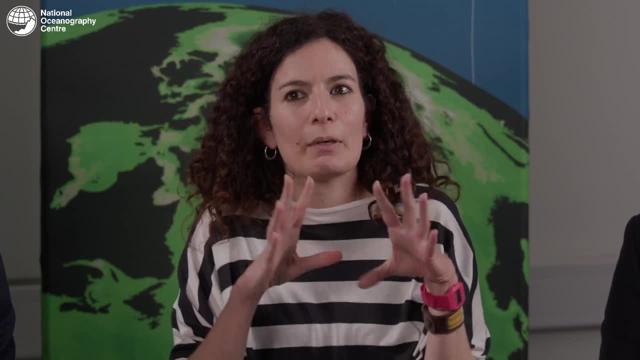 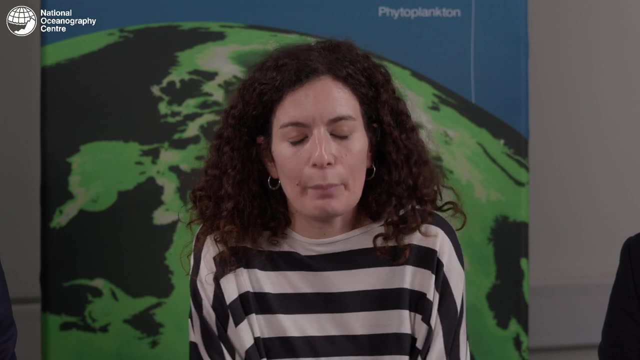 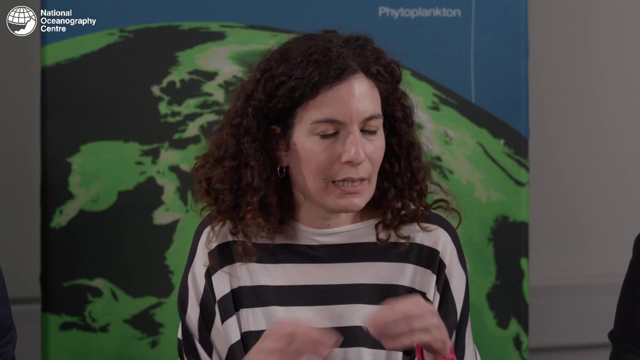 wind turbines or the other string turbines. it's just a matter of understanding what is acceptable and, for example, i've been in the past. i've been studying what was going to happen if we were going to put a lot of tidal stream turbines. tidal stream turbines are like wind turbines, but underwater. 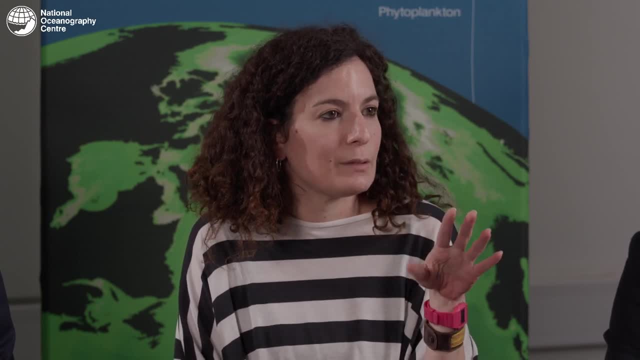 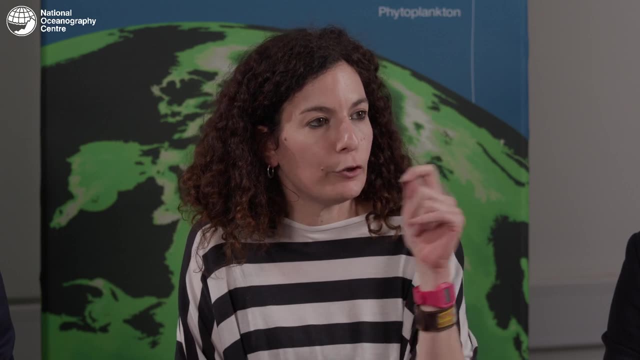 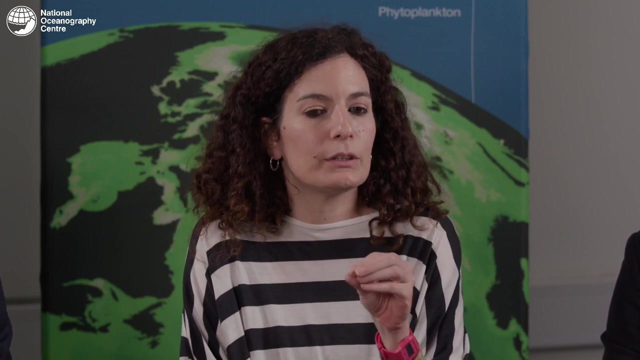 and actually the uk, scotland, is a very good place because there are very strong tidal currents and there are some tidal turbines being tested in the pentalford and i was simulating what was going to, what will happen if we put thousands of turbines and perturbing actually the tidal currents. 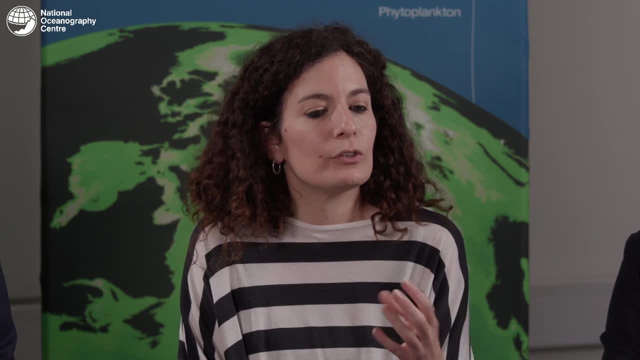 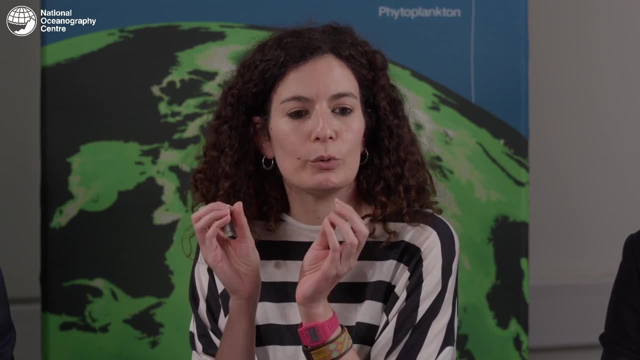 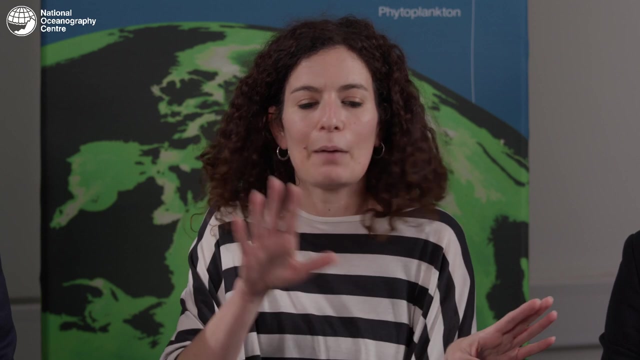 the tidal dynamics, and then i was comparing those changes due to so many turbines with the, with the changes that we are going to have with climate change and the, and comparing them. i mean the comparison is like that and climate change is going to be 10 times bigger than the effort of 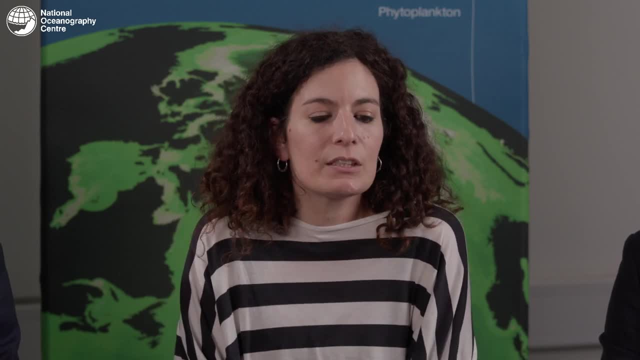 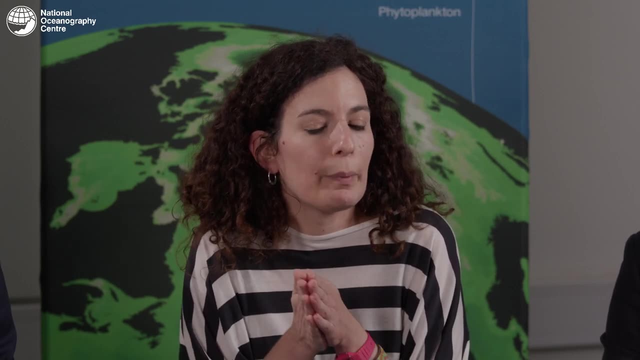 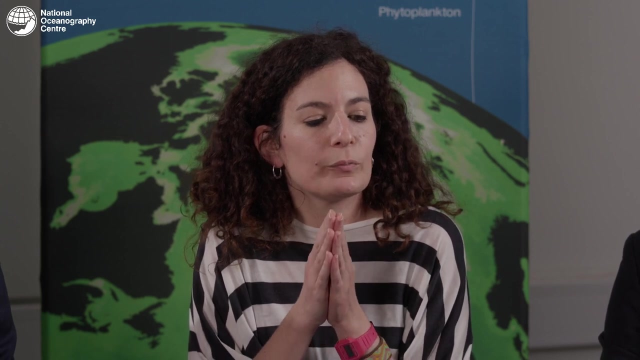 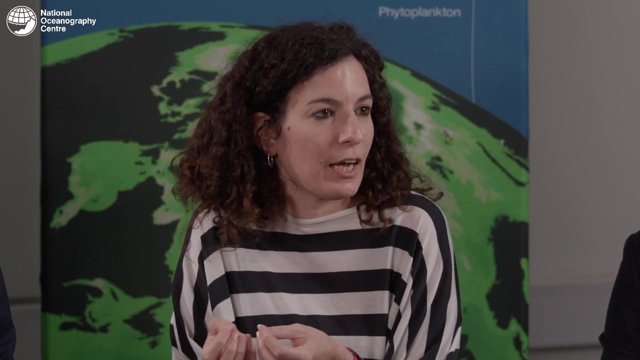 stream energy extraction at such a big scale. so the take-home message of this is that even if there are going to be some negative effects, they are acceptable because we are going to, because in that way we are not going to see much larger effects. that are the efforts of climate change. 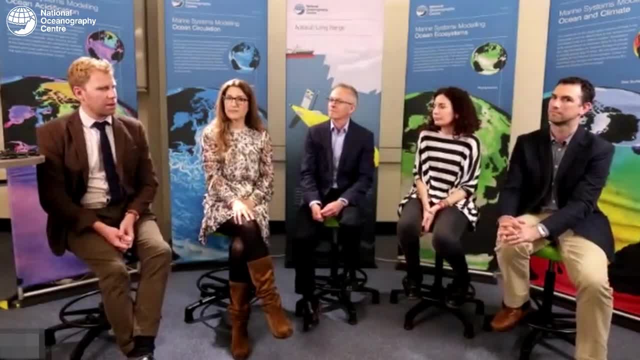 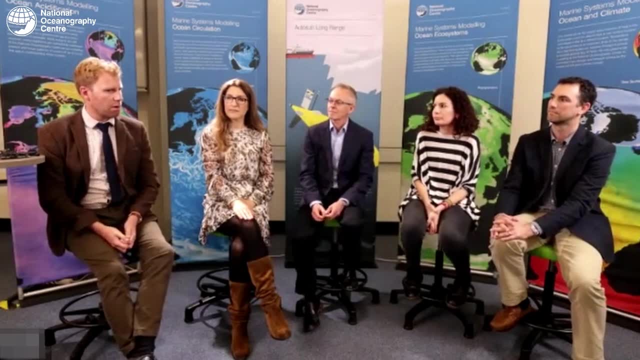 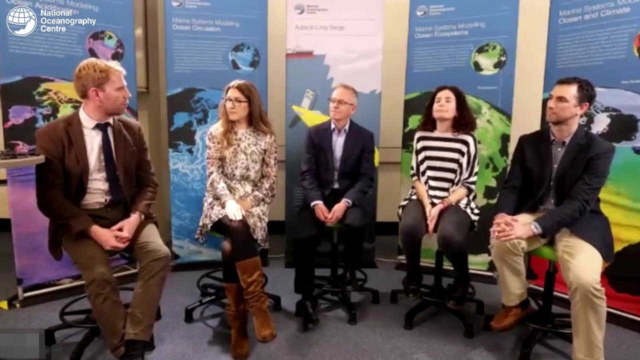 so i guess, um, just just thinking about, um, i guess, the the potential impacts on on our ocean from some of these solutions, um, i think what i'm hearing is that the oceans are pretty tolerant, pretty tolerant beasts. you know, it can deal with quite a lot thrown at it, be it engineered solutions. 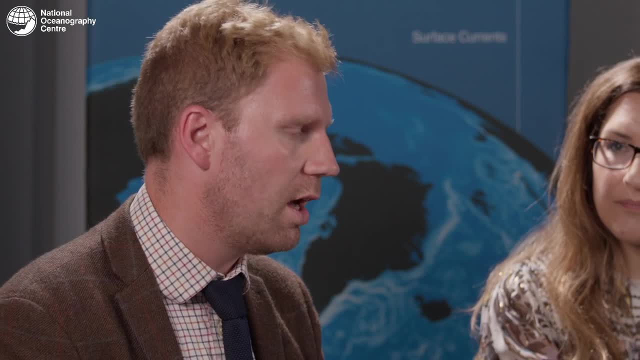 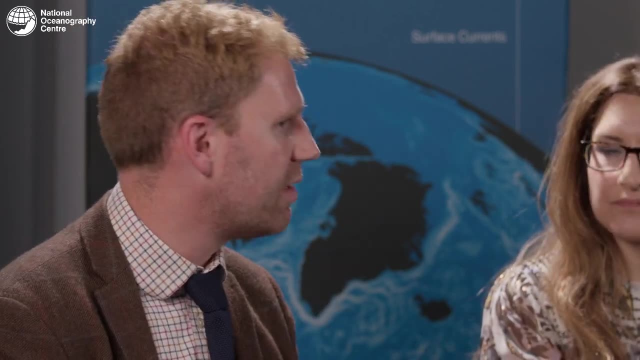 clearly nature-based solutions are the win-win, as you alluded to, um chris. is there anything that we shouldn't be doing? you know if, when, if we're in solution mode, where, where's the line where something does become a problem problematic in your view, either from a scientific perspective or 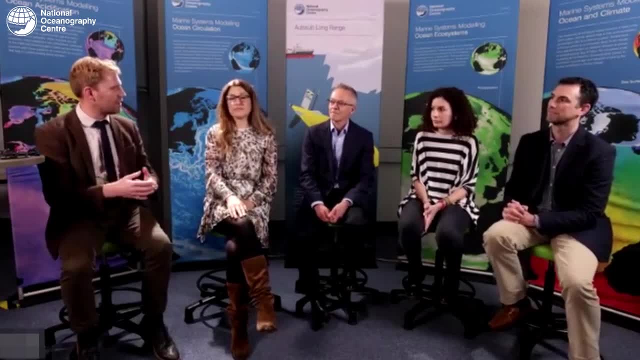 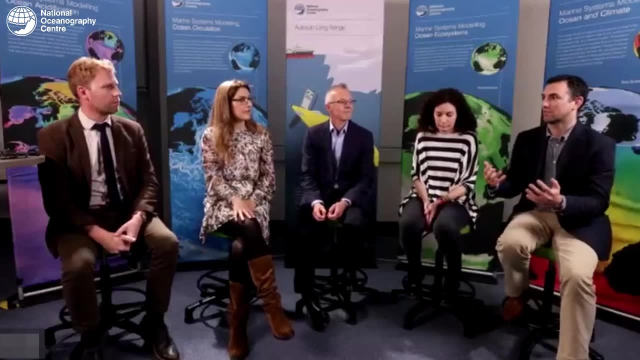 from a, from a real life, you know, coastal hazard for someone living there. is there anything? is there a line that we should not cross when we're in solution mode? well, there are examples of people conducting trials and experiments when, in terms of iron fertilization, that haven't been well conceived and well planned out and 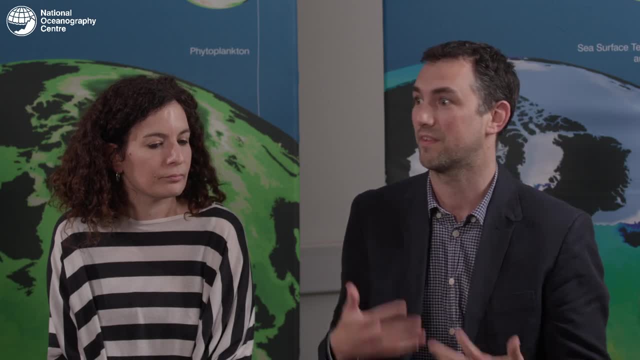 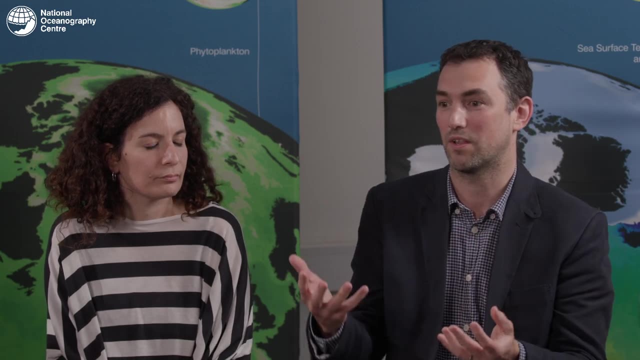 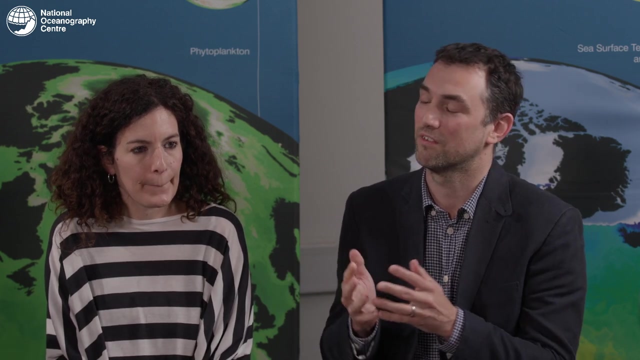 well conducted and they have automatically created lots of negative press, negative negative attention and- and i think it's that- that jumping in with two feet, so to speak, uh, with the, without really considering the broad implications of what's being done. and that's the risk. Now, it's not to say that iron solution, iron fertilization, can't be part of the pool of 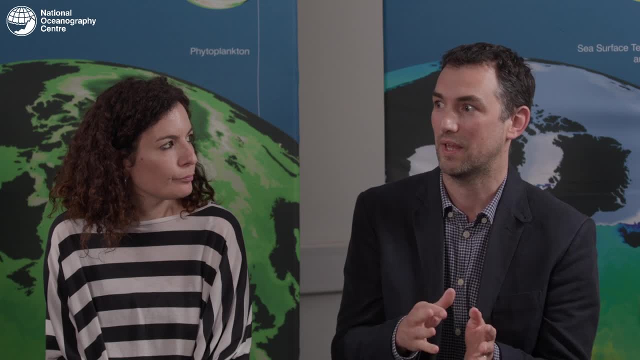 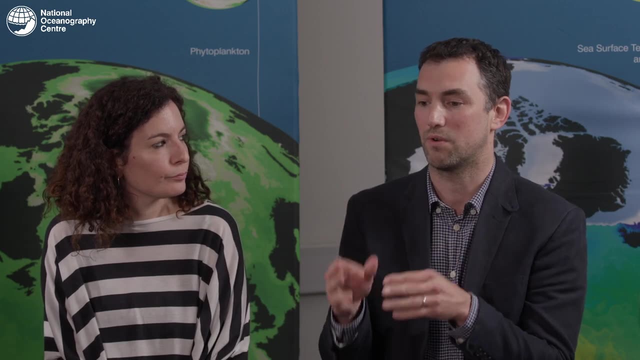 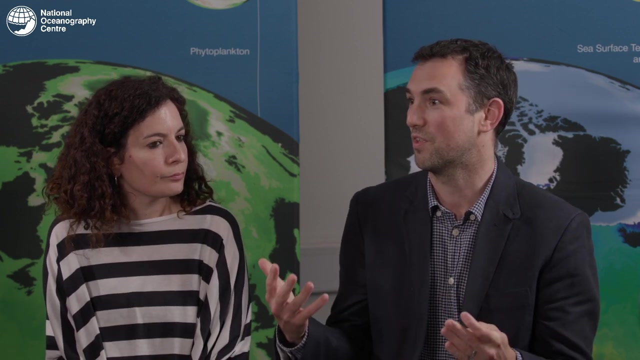 activities, but it needs to be assessed thoroughly and properly, scientifically, with rigor, before it's actually conducted, because it may not be applicable in all circumstances and having that knowledge and understanding is essential. So I think there's lots of techniques out there and I think we just need to pursue them. 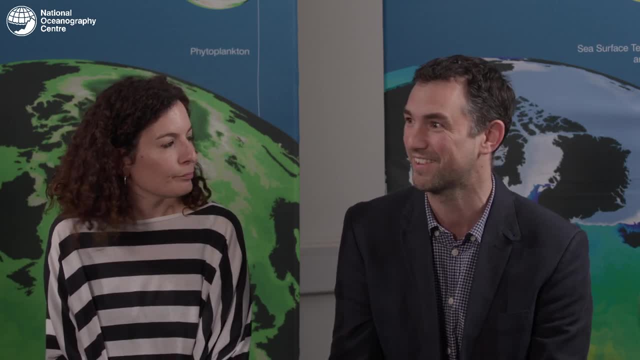 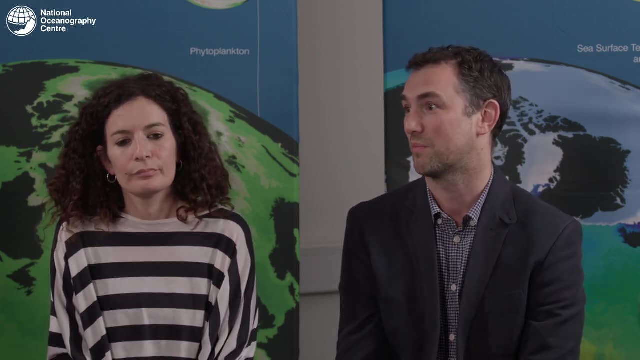 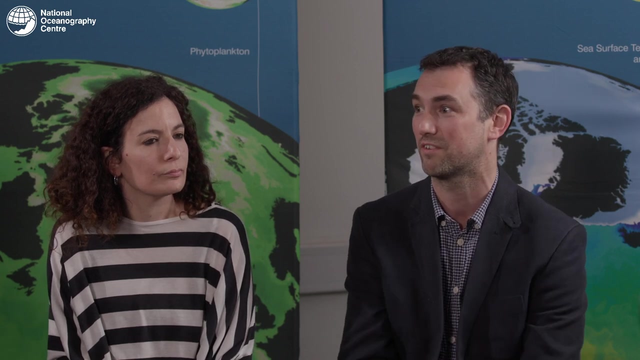 As scientists on this panel, we will naturally be hesitant. We know we want to get it right and ensure 100% safety. but on the other end of the spectrum there's the commercial implications. There are net zero deadlines. they are coming closer. We have to achieve them for our future generation's sake, so we need to be pulled out of our comfort. 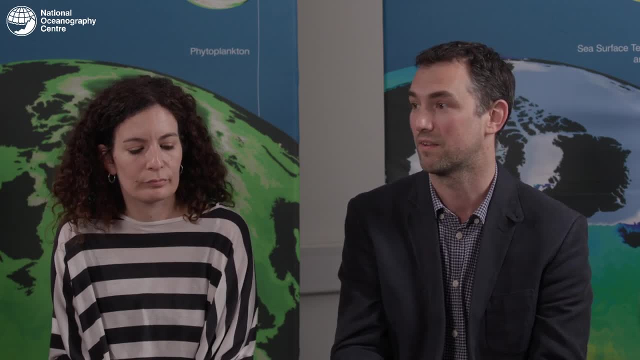 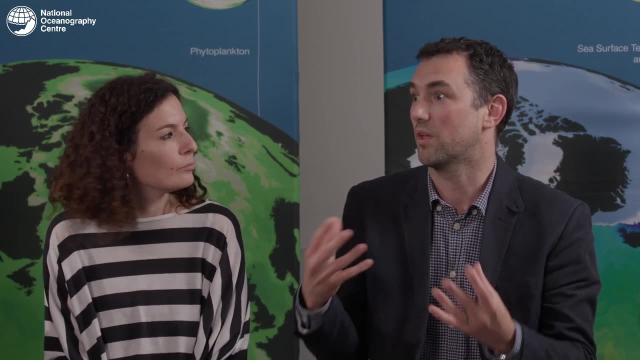 zone in order to enable companies to meet those target deadlines, and we, as a global population, have to be comfortable with like. well, what are we going to offset? You know, What are the? what level of impact are we happy with, in either the oceans or at land? 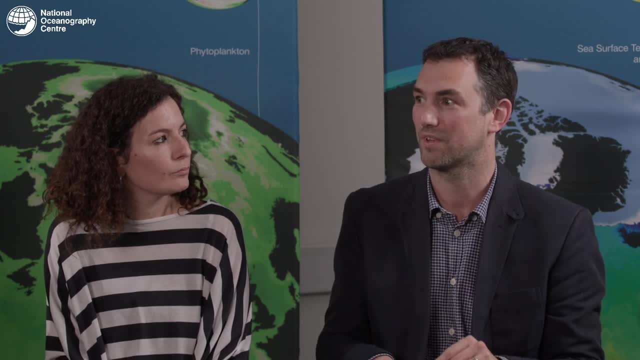 You know CO2 has got to go somewhere. If it's not going to be in our terrestrial reservoirs, then it's got to be at sea. So you know we have to make decisions as a global community to say this is where we're. 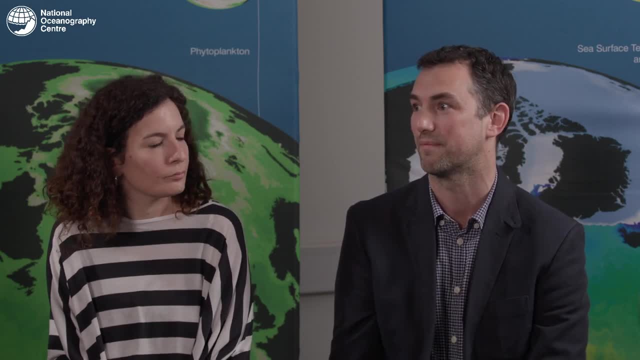 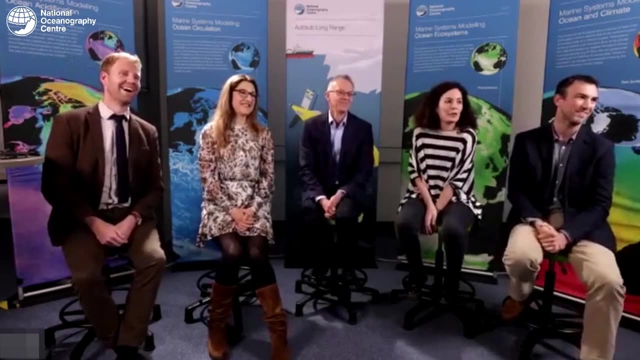 heading what we're going to do if not, and how can we best get that? I've got a couple of hands up here. They're both at the same time, I'm afraid, so Sure, Kind of going on and off with some. 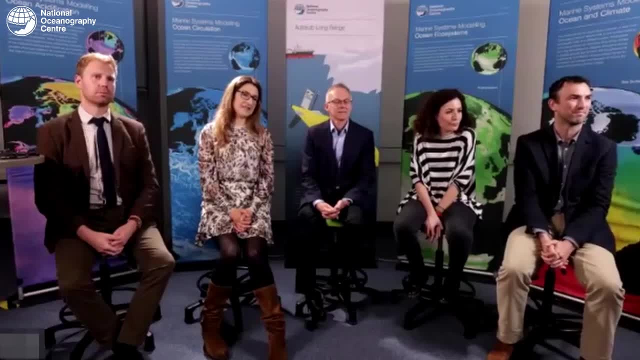 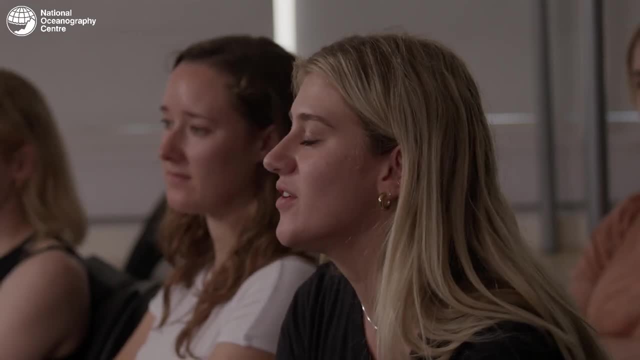 Yeah, A lot more young people have gone into science and a lot more young people have kind of taken to the interest of it, especially in climate and it's like a lot more, I think, in the media and stuff. Do you think that this next generation is going to be really focused on, you know, climate? 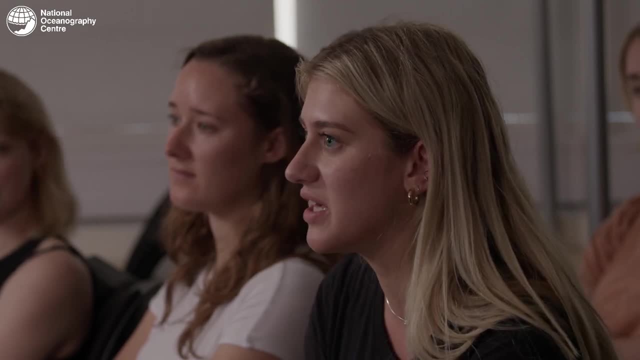 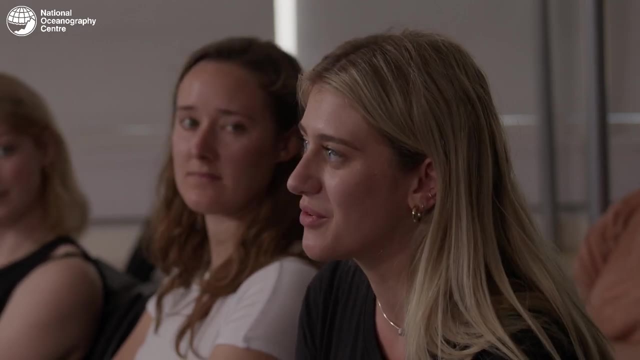 solutions And do you think, if so, how important that will be in terms of actually getting to solutions with an entire generational backing of it, as opposed to what we've seen before? So I think that's a good question. Yeah, Yeah, I think with that, I would say you're right. 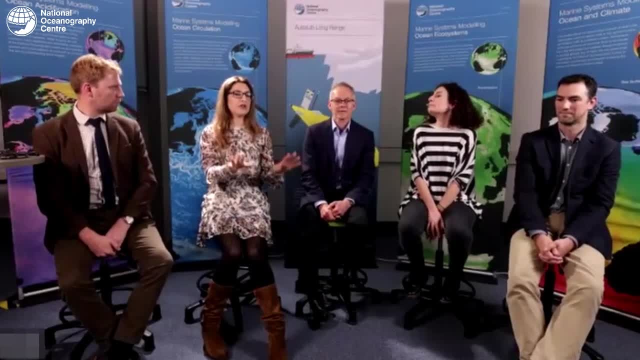 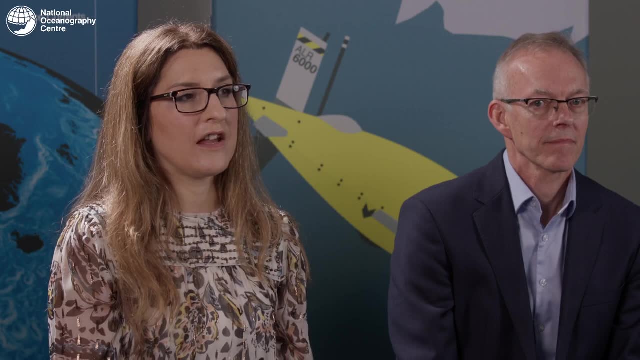 There does seem to be- you know, it's unequivocal- in the younger generations There seems to be a greater sort of literacy in terms of the environmental threats that we face right now and definitely more sort of action in terms of you know, how can I live? 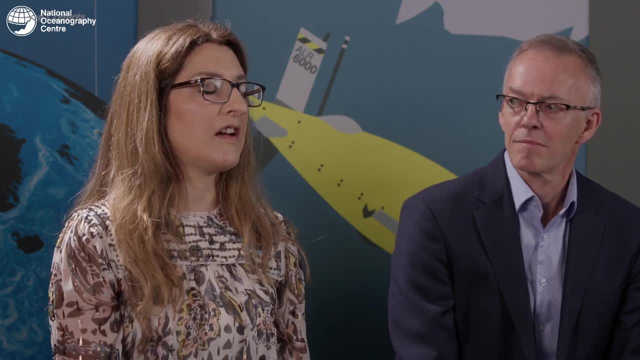 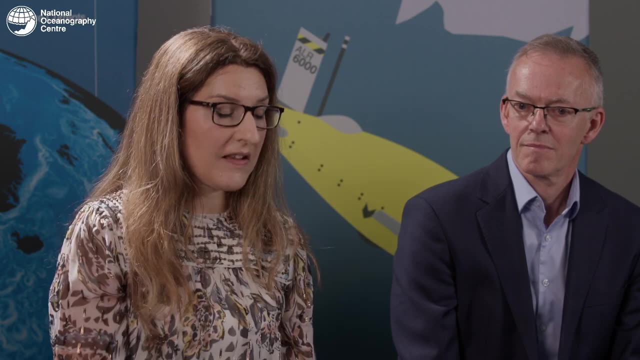 my life in a way that's going to minimize my impact. So that definitely seems to be the case, that it is more prevalent in the young generation. But I would say that we can't afford to wait for that young generation to sort of be the 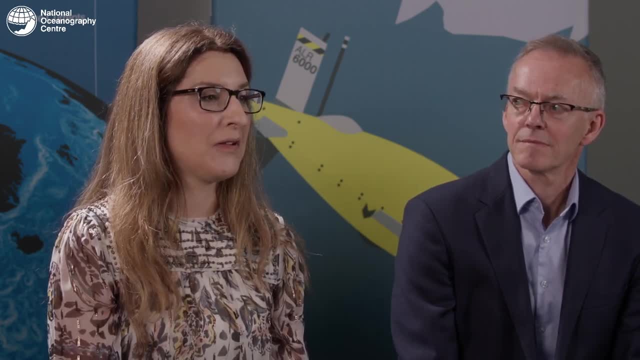 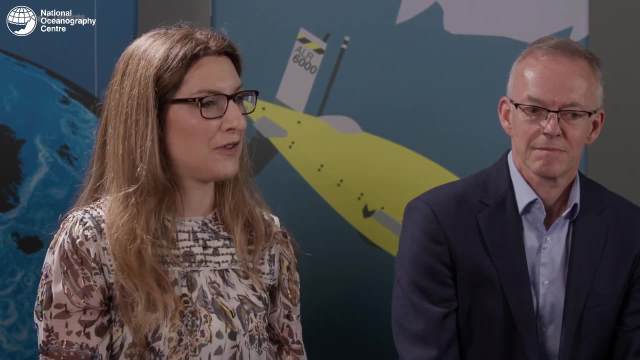 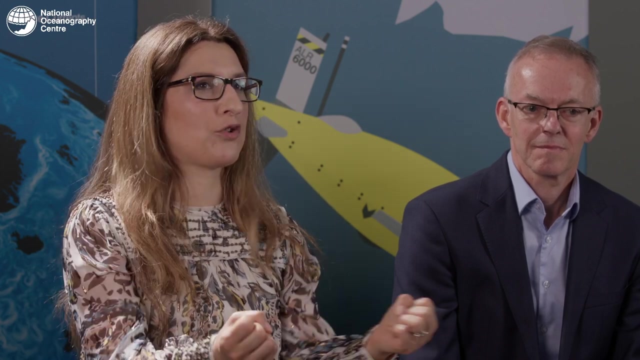 ones making the decisions. You know it has to be an ongoing process that we're all involved in and it starts now really. So I think it's important that that the youth- you know the youth are going to be extremely important, But, yes, it's the here and now. we can't give up trying to reach those unconvinced people. 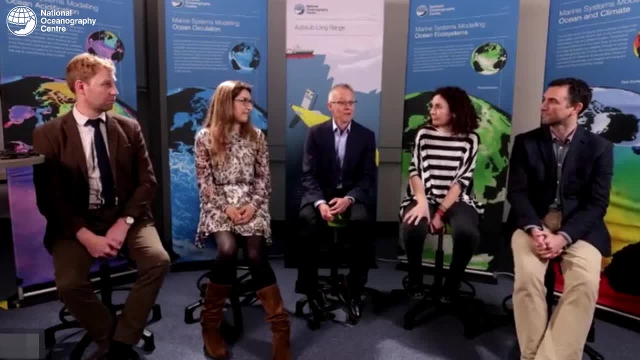 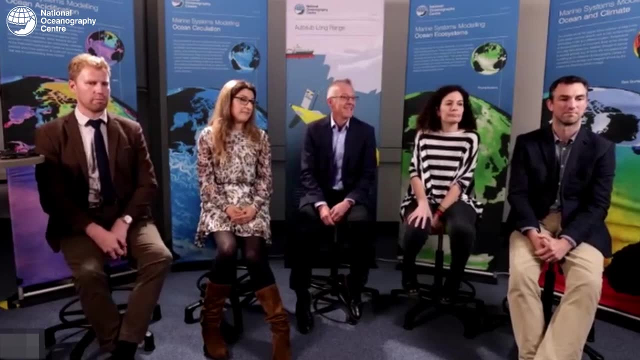 as it were. You know One thing on that: you've got a real leverage aspect there that young people in the past didn't use to vote, So politicians didn't really care about the young people. I think you saw with the you know Obama and a real mobilization of the young voters around. 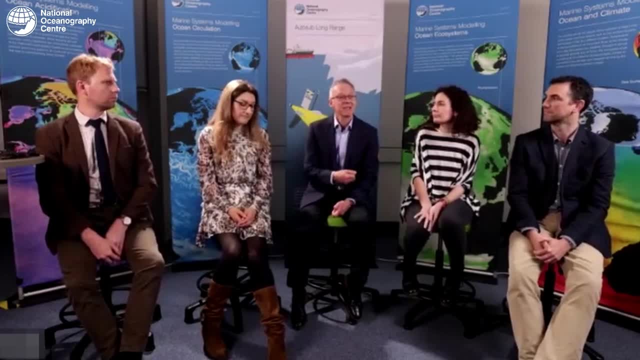 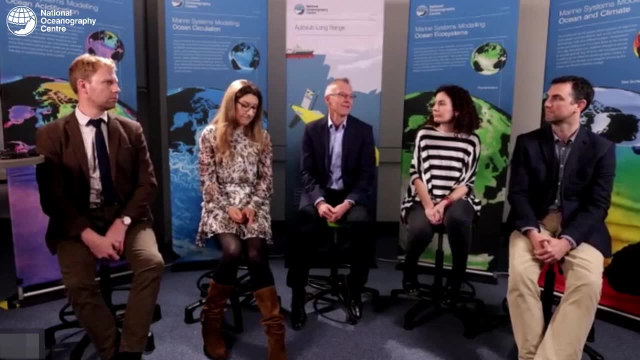 the planet. I think there's a real push there as well in shaping politicians and how they do things, And I think you ignore the youth. vote at your risk because you won't get elected. I think in the past they didn't really care, because only people like to vote. 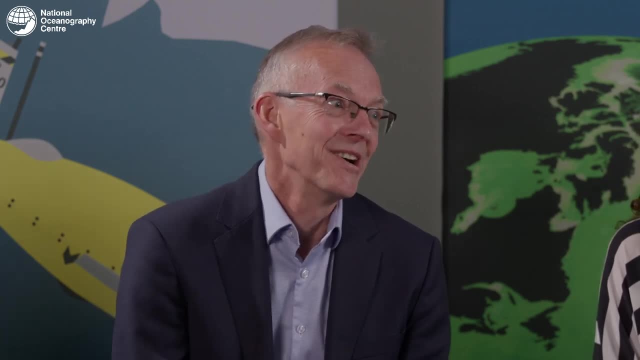 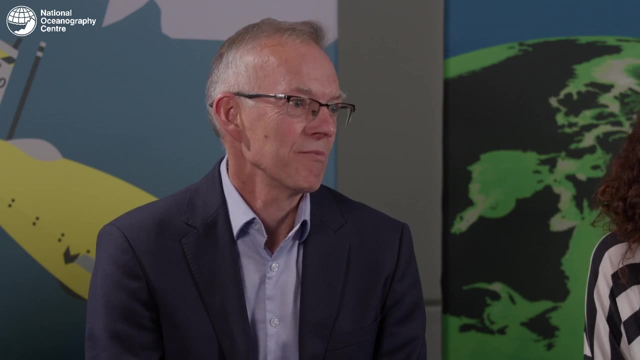 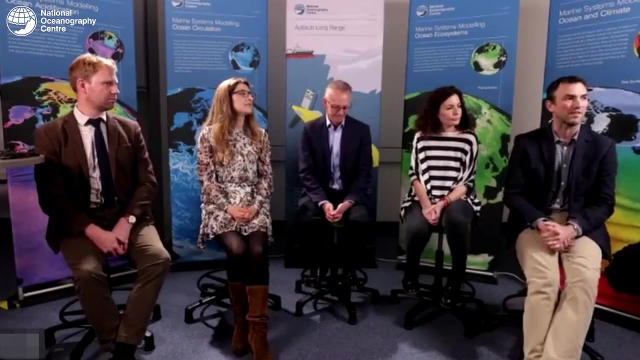 So, yeah, that whole mobilization is a real political move that will hopefully translate into good things for the environment in terms of politicians doing things. Yeah, I just want to say that I've been a marine geoscientist for 20 years and I've never seen 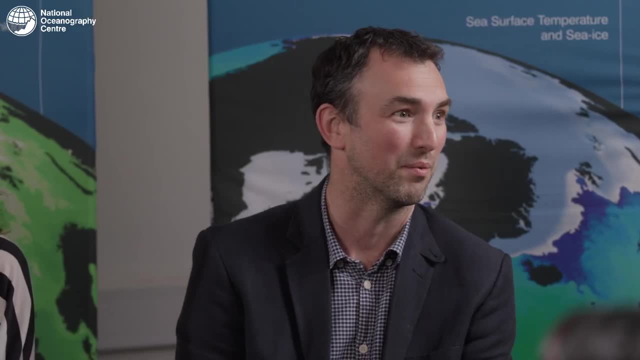 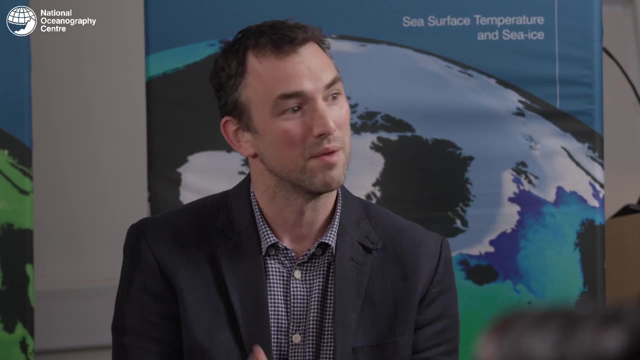 a field developed as swiftly as ocean based. This is really ramping up very, very quickly and in no doubt, a support, you know, reflection of the support, but also the urgency. I think that urgency is recognized by politicians, is recognized by people and I think just is. 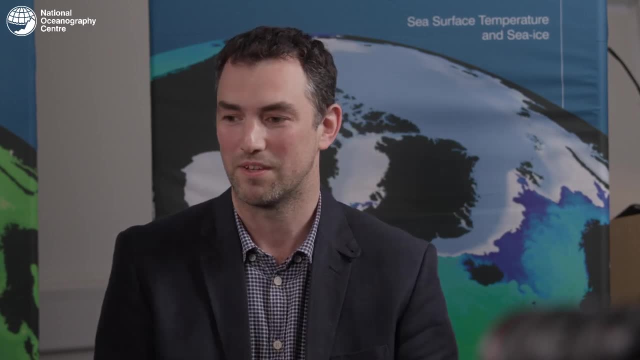 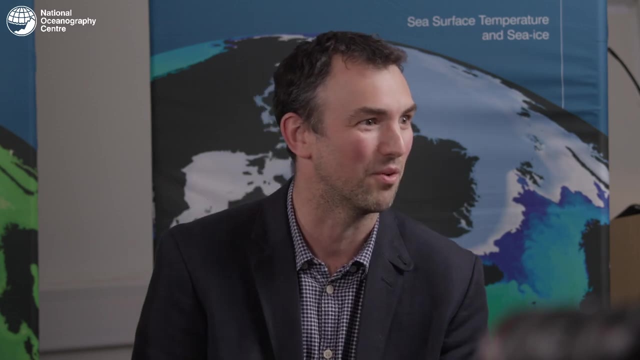 finding the right way to achieve that. I think we also need to just kind of recognize that we now live in the global society. You know this was not the case, you know, 10, 20, 30 years ago. You know there is a global voice now. 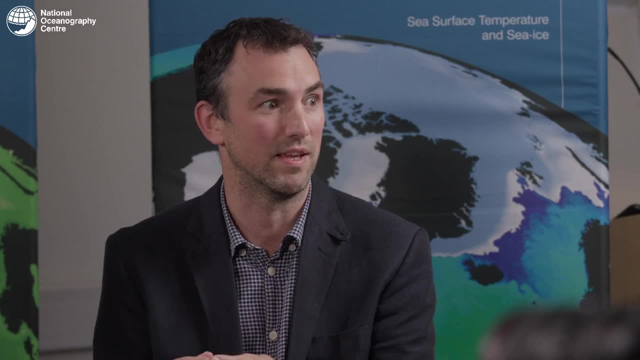 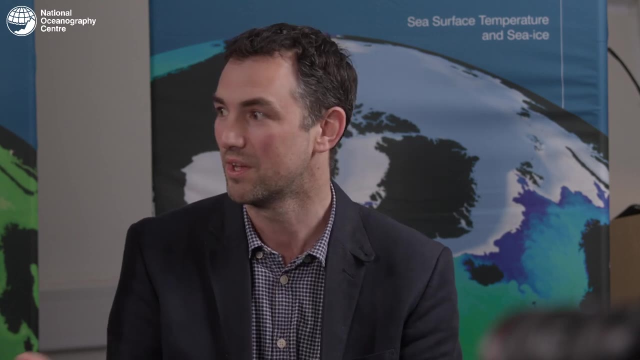 People are pulling together to tackle this problem, and that is what is needed to solve these issues, because it is a global issue And I think that is where future generations going to come to play. You know, we're going to have Our own net zero oceanographic capabilities. 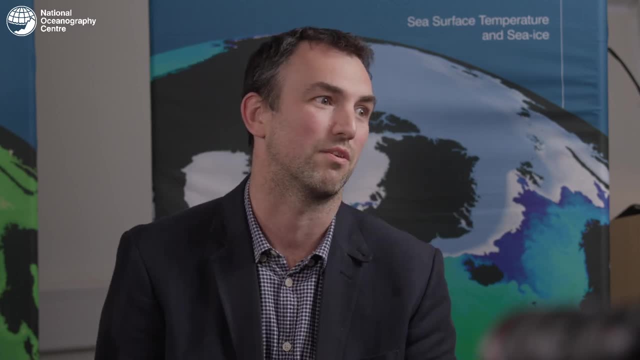 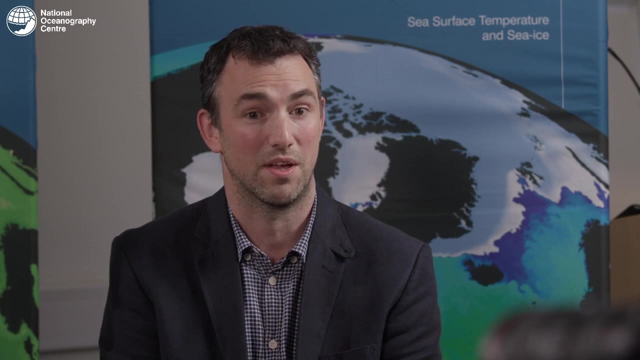 That's all of our internal targets. You know there's going to be other net zero targets internationally for travel. You know, again, we need to embrace that, support that and then find ways to live as a, as a new community moving forward. So I think that's that's the encouragement for the future. 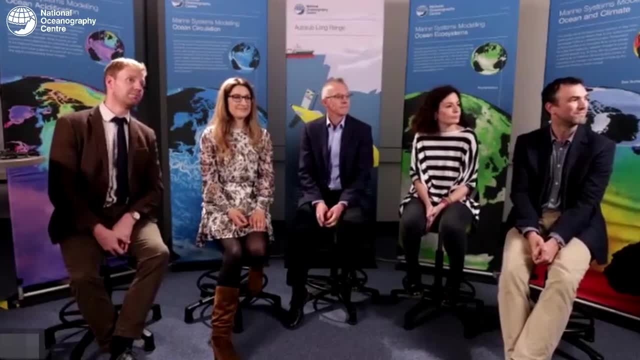 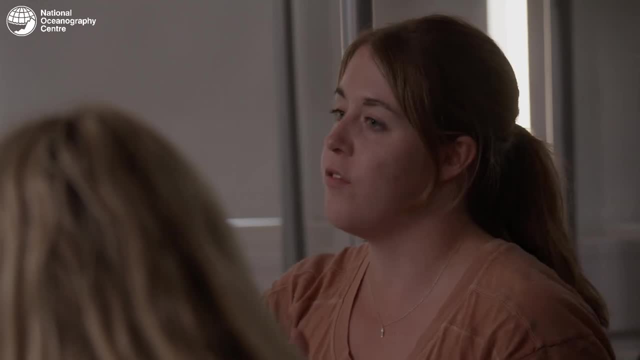 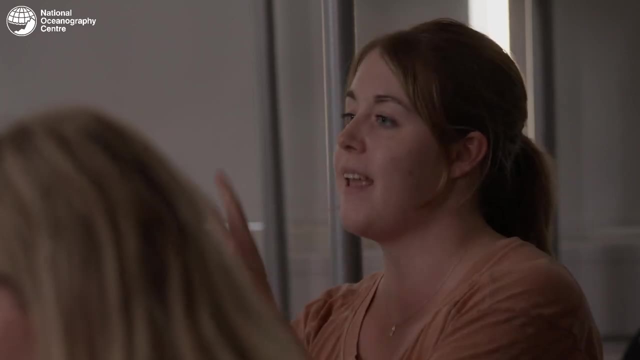 Britt, there was a question over there. Yeah, I just want to ask what you think the biggest barrier is implementation of some of these solutions. Is it uncertainty over long term consequences? So some of these, is it purely like logistical How, like practically getting this infrastructure set up, or is it just social and political barriers? 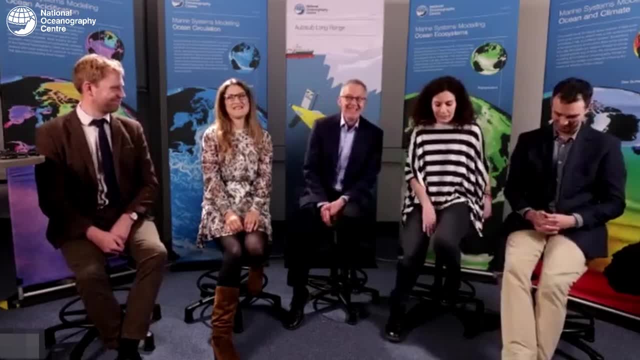 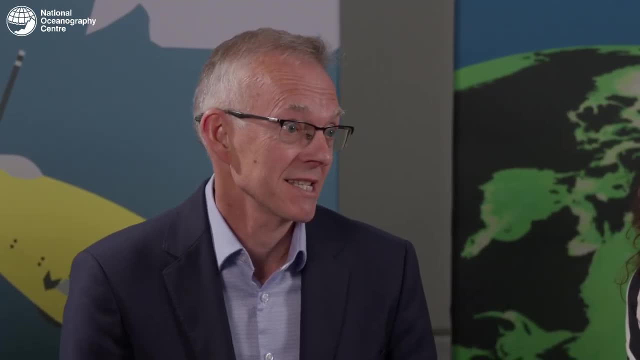 I've talked to CCS versus what I know most of. So CCS varies country by country. So Germany hates CCS. They, the public, really don't like CCS. UK is more acceptance around it, America the US is more acceptance around. in Canada It's being used a lot. 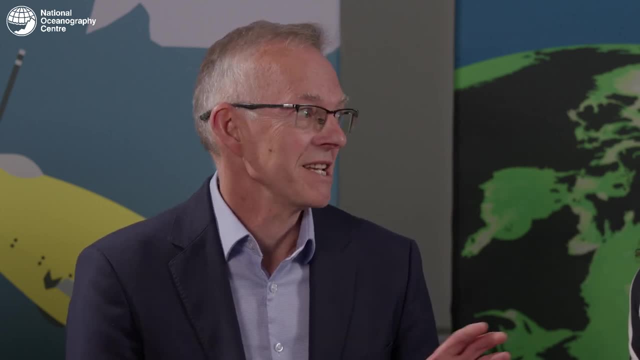 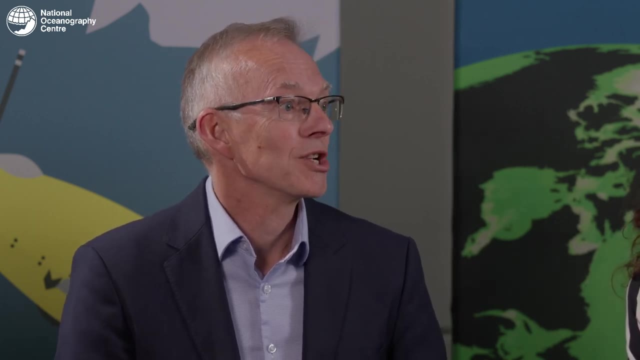 Canada it's being used lies on land. There is still the risk. People public is still a little bit disturbed as to how or whether it leaks where they could see it And financially it's an expensive process to get it off the ground because we still 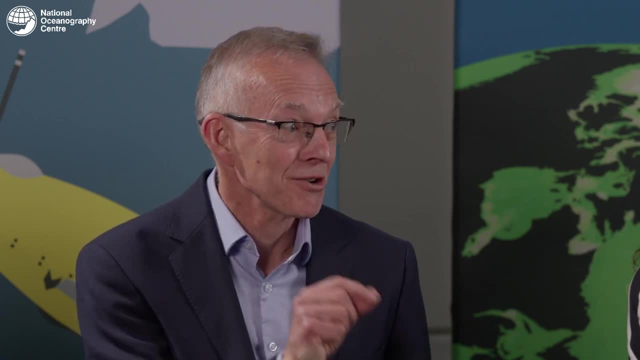 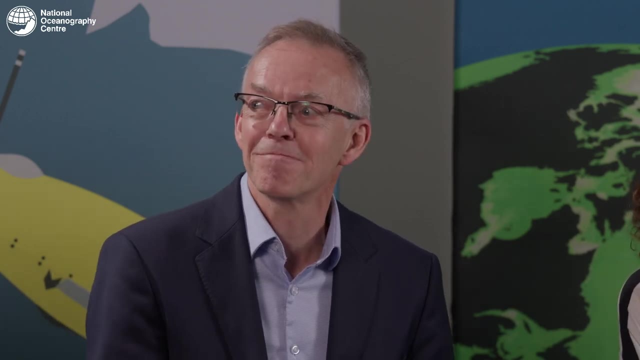 haven't got a carbon tax credit system that works. If you really charged carbon out of what it costs in terms of all the damages to the environment, we wouldn't be. we wouldn't be trading carbon at $30 a ton. We'd be trading carbon at $3,000 a ton to actually work out. 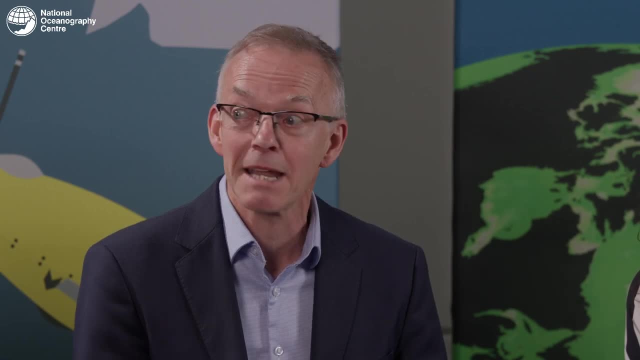 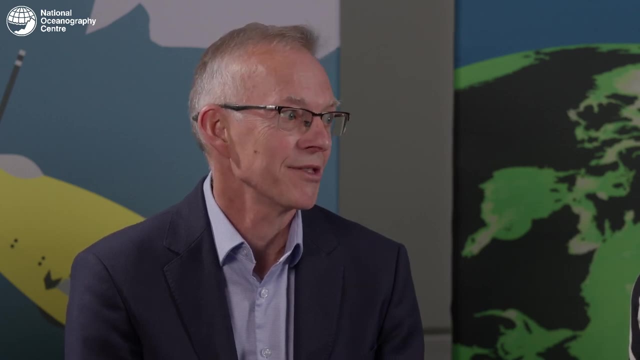 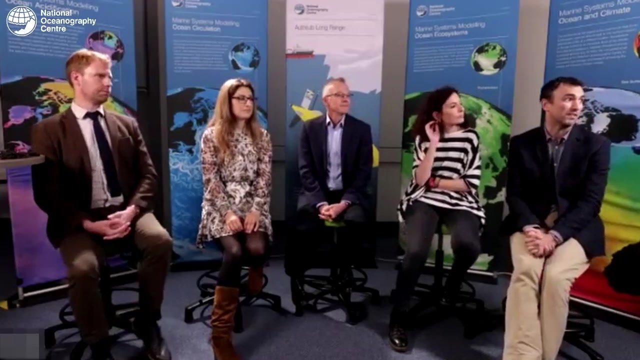 Actually what it's costing us Every man, woman, child and animal on this planet. But yeah, so that is. the biggest limit, they say, is financially, But the cost of not doing anything, I would argue, is far, far greater. I guess you know it varies per technique that you're taking. 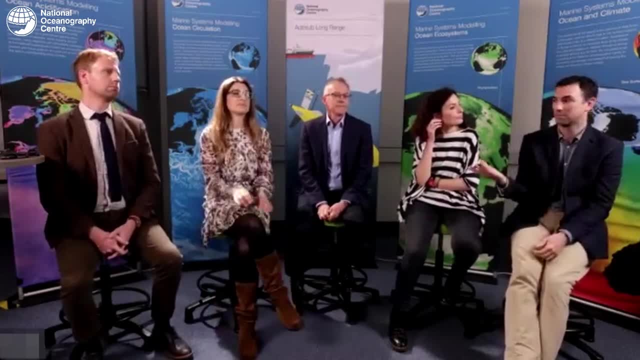 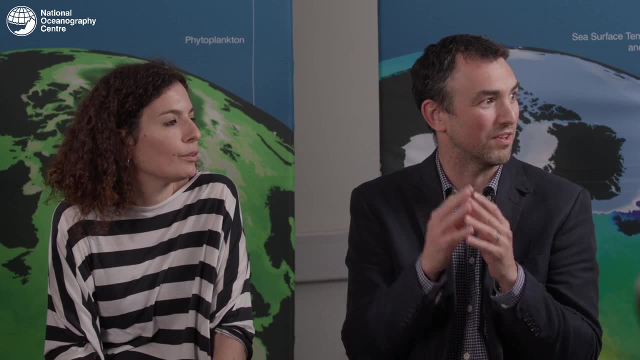 You know there are quick wins or easier wins. You know, for some of these solutions, like CCS, we already have the infrastructure. you know. But when the critical thing for us is not to just look at the solutions, It's a look at the problem. 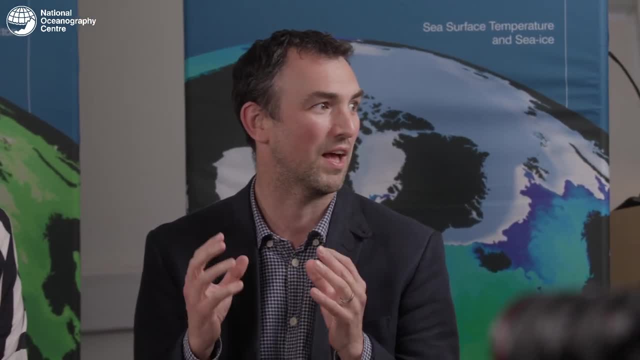 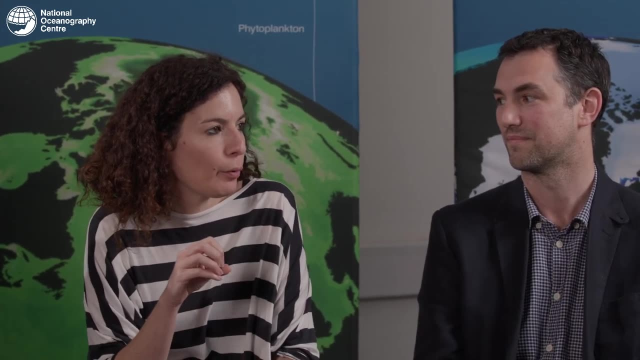 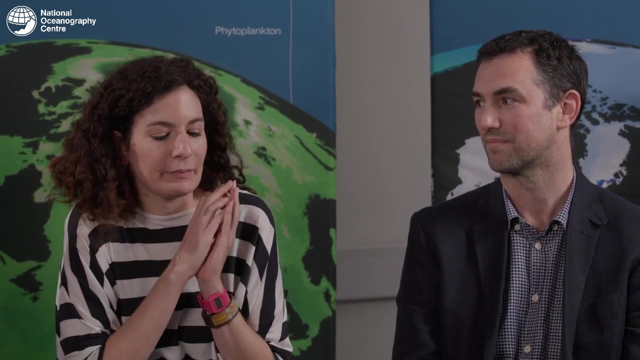 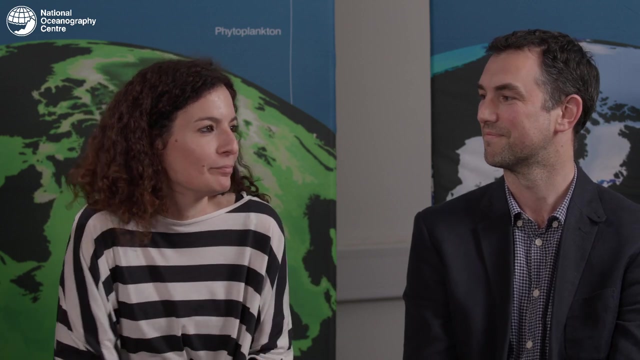 That's where marine renewables come in. Stopping this CO2 emissions has to start there. About the limitations of the technology of marine renewables, I mean putting something in water that has to stay there for a long time. It's not that easy because, whatever I mean, if you put something there, it's going to be full of microorganisms in very little time.